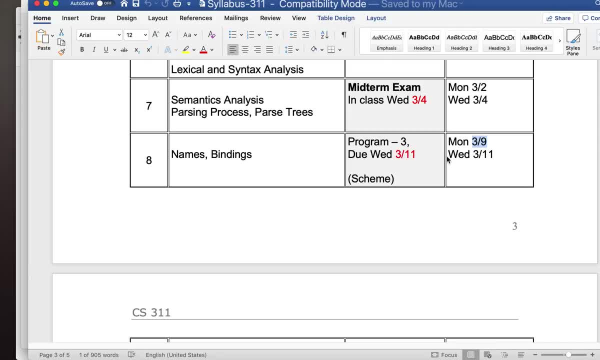 gone over it, so I'm not going to go through it. I'll go over it again. So if you have a question about one of your answers, then it's best to contact me by email and then we can connect via the phone, or actually you can contact me by phone if you. 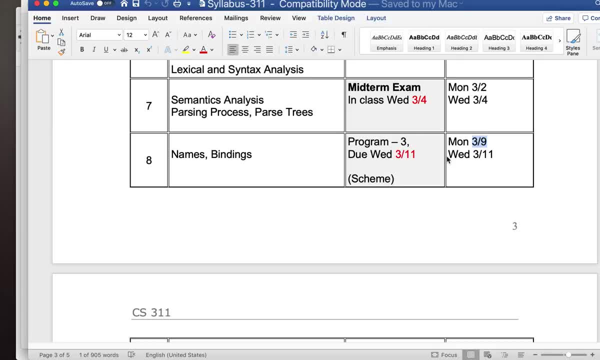 wanted to. We can connect by phone, by email, by zoom, any means electronically that you'd like. I'm just not holding office hours on campus, so you'll need to connect with me electronically, which is not a problem. I'm very available, so it should work out just fine. 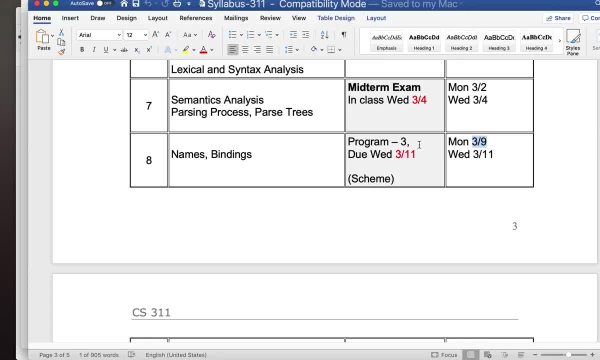 So that was my talk today. I hope you enjoyed it. I'll see you next time. Monday's class meeting: we went over the midterm and we didn't have that good of a turnout, which is why I sent you the midterm. So if you did not receive your midterm electronically, 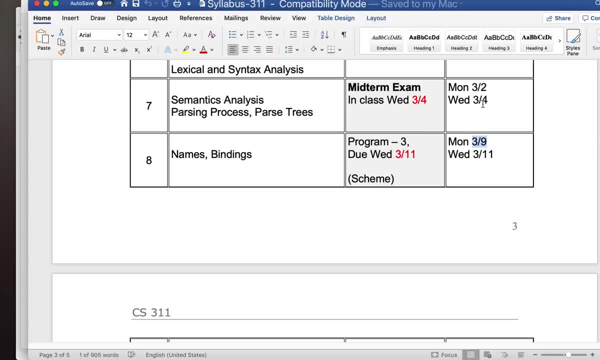 that means you didn't come to class and pick it up on that Monday the 9th and instead you you got it like hopefully you got electronically. If you did not, let me know. it means I sent it to the wrong person or something like that. who knows. 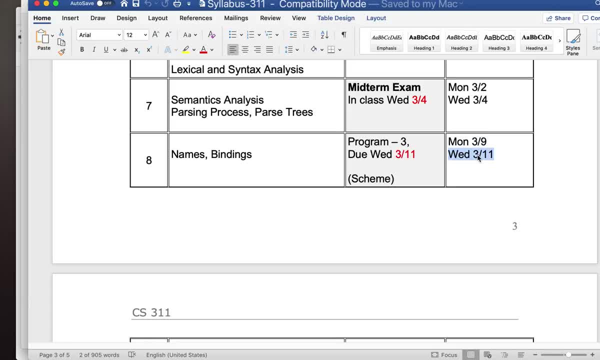 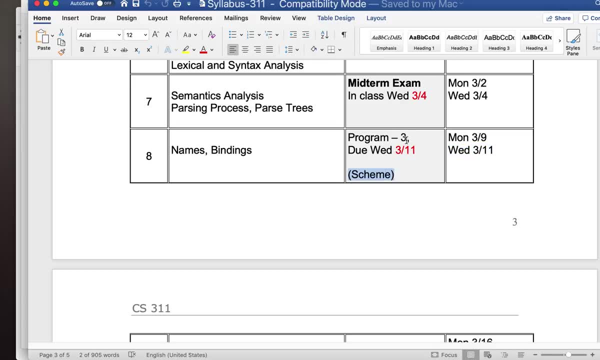 We did not have class on 3.11 because 3.11 was canceled by the university And so on 3.11, the scheme assignment number three was due. I've already gone over scheme in the class. There's a scheme lecture or two that you could. 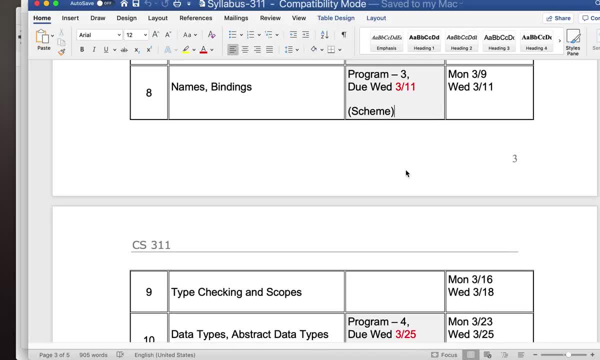 review as well. Scheme is pretty straightforward. You can use the built-in functions. You don't have to reinvent the wheel. You don't have to use just the LISP functions At this point. just make it work, Turn it in. You still have seven. 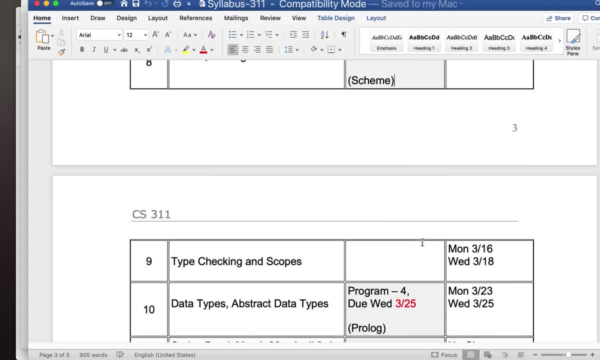 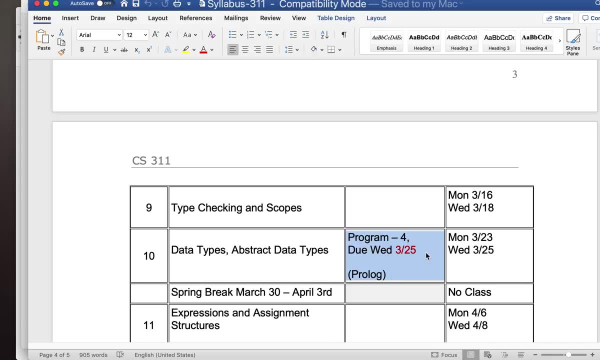 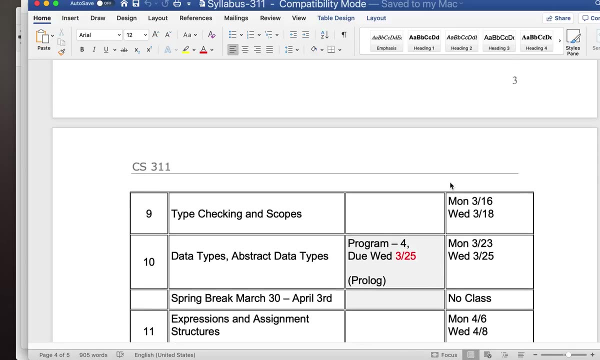 days grace on it. And then next week we have assignment number four due, and assignment number four is on prologue. So today we're going to cover the prologue programming language and get you up to speed on that one, Okay, and then after: well, it's not due this week, it's due next week is the prologue assignment, And so 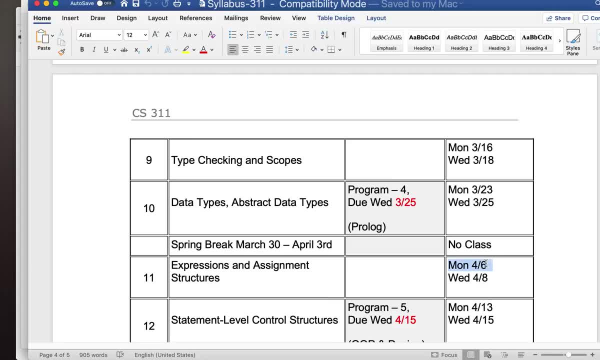 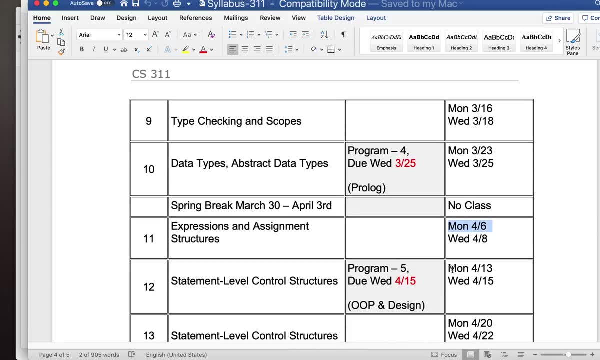 then after that we have spring break and I suspect that around Monday, the 6th- I don't know I could be overly optimistic, but I suspect around the 6th- we might actually be meeting again in person. So we'll see how long this lasts online. 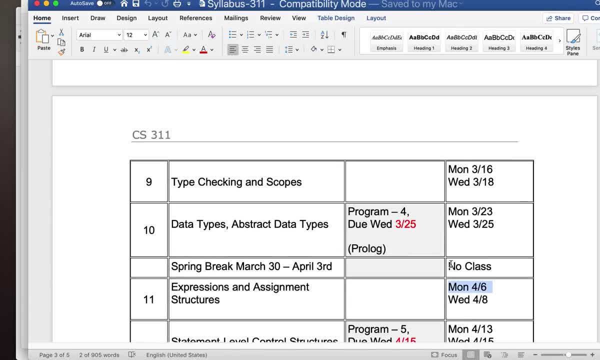 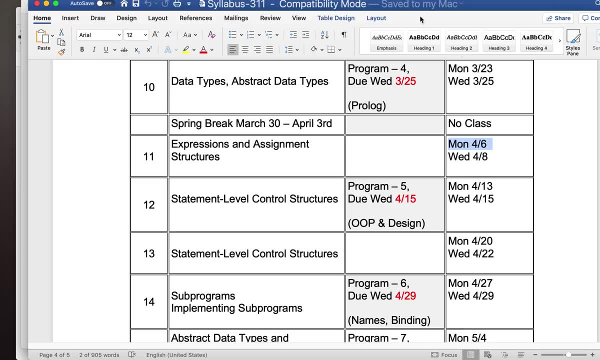 In the meantime, you can listen to me via the YouTube videos instead of having to drive to the campus. So let's see how long this lasts and we'll see what's played by ear. So if you do have any questions, I can't ask them. You can't ask. 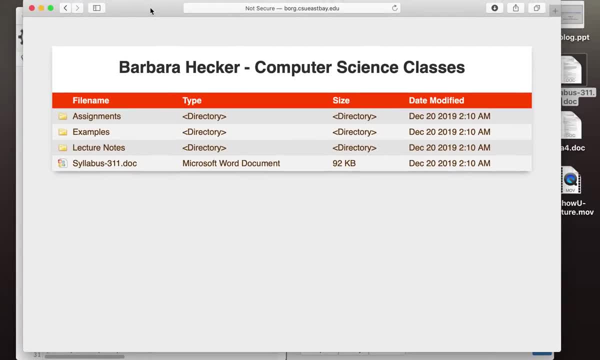 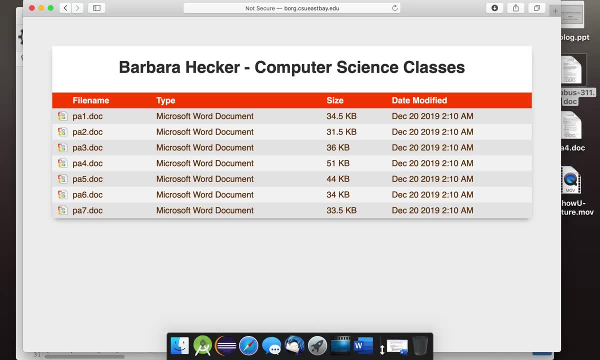 ask them. right now. You have to sort of hold on and send me an email so I can answer your questions electronically. So in the assignments folder, if you download assignment number four, assignment number four is going to bring up the prologue assignment and the prologue assignment. 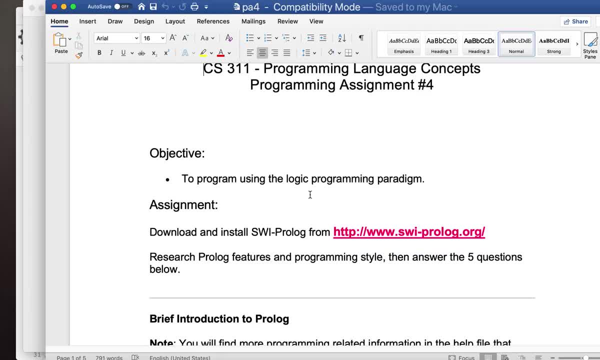 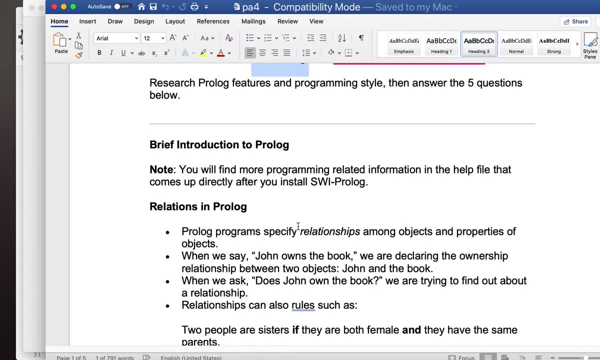 Here has you experiment with a language called prologue. Prologue actually stands for programming logic, And so the traditional form of it is downloaded with SWI prologue and you can install it on your computer and you can run prologue programs and create a bunch of good stuff on your computer and load. 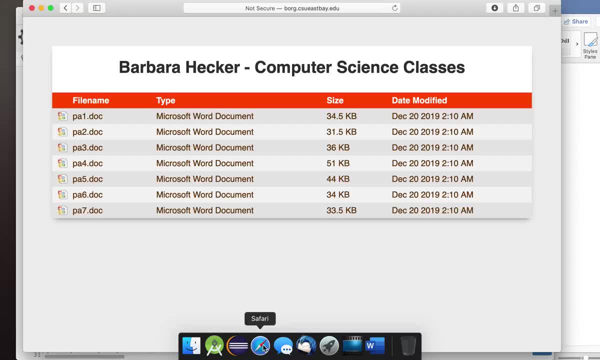 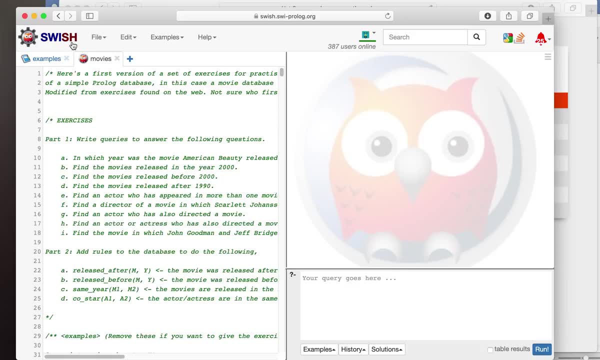 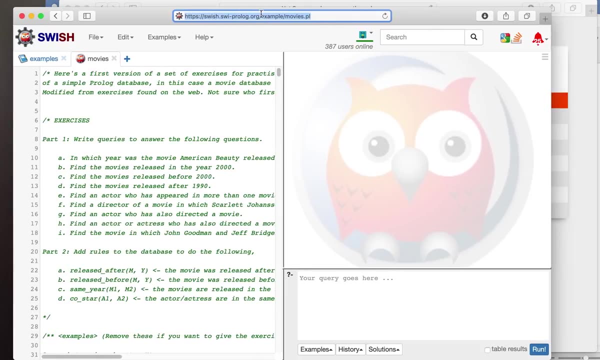 everything locally. However, there's a better interface. if you'd like, called swish and swish, SWI prologue, Which is SWI prologue. SH stands for shell. You can see it right here at the top of the screen. Hopefully you can see that It says swish dot, SWI dash. 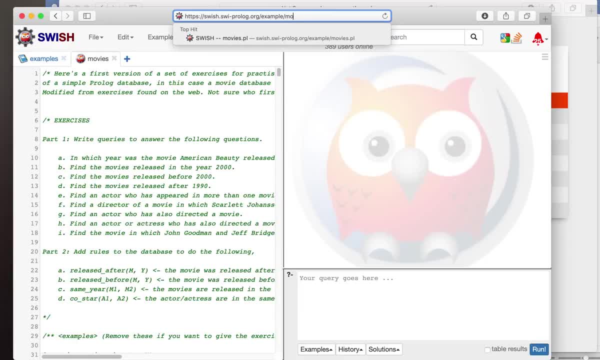 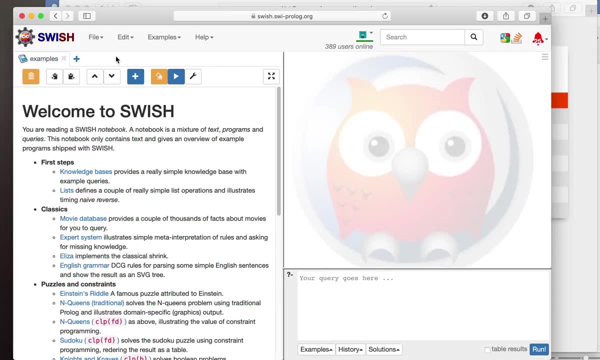 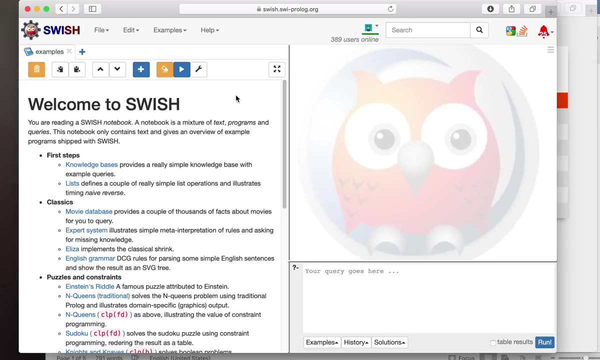 prologue dot org. And when you go to this website, you can write all of your programs online. You can do it right here. This is the welcome to swish. You can read about it. This is an online prologue interpreter That you may use for the assignment, So you do not have to go to prologue And for 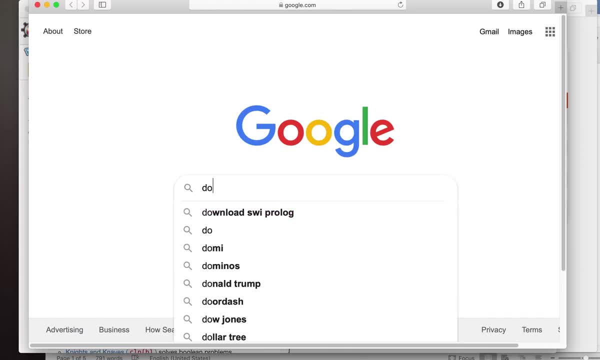 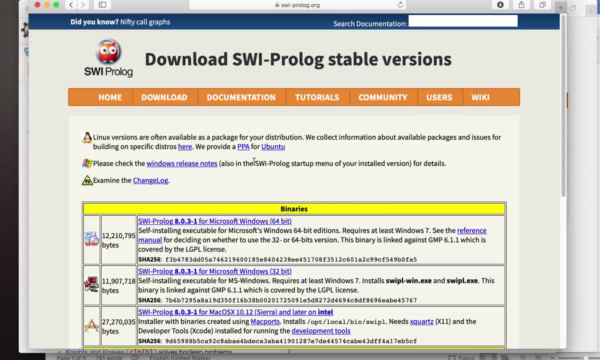 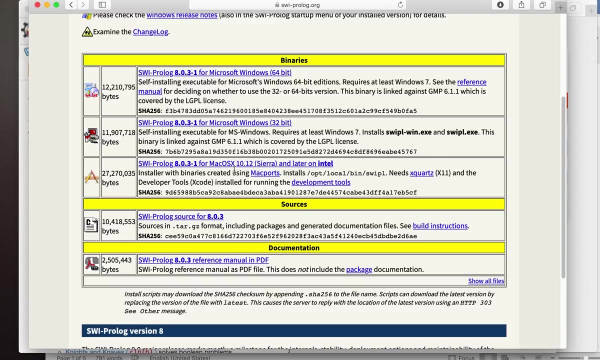 example, if I typed in download SWI prologue, You don't have to download this version of it. This looks like a website from the 1970s. It still works, though, And you can load prologue locally. In fact, there's a, there's one for the Mac, There's. 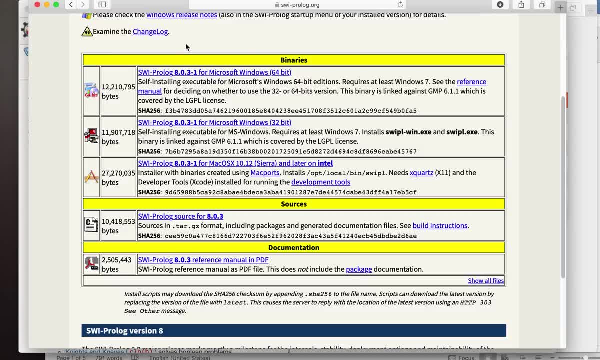 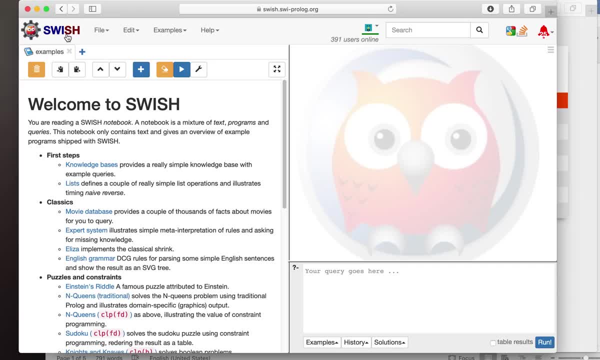 one for Windows, And you can run SWI prologue locally On your computer if you prefer, But most students would like this better, So you go to this website, SWI prologue, Which is the same prologue. It's the same logo. 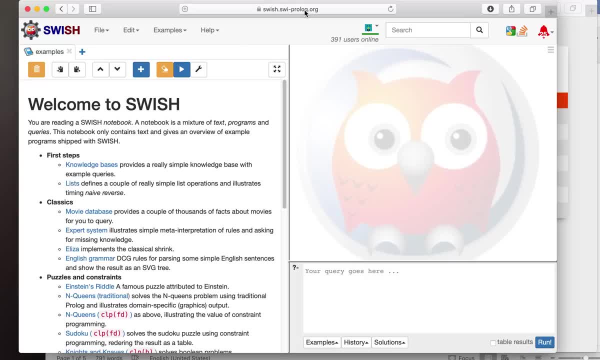 Same everything, And you can do the assignment right here. And so what are you going to do for the assignment? Well, we'll see momentarily here, But the other good thing about this is you can go into the examples folder And see the example. 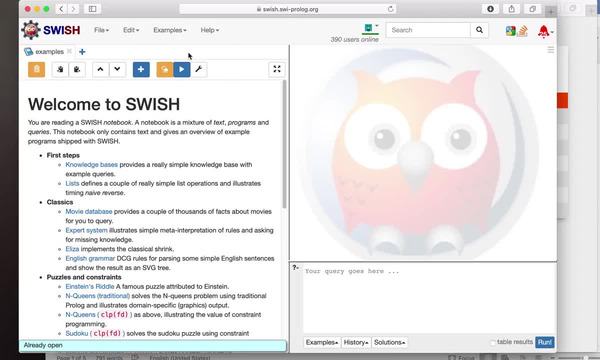 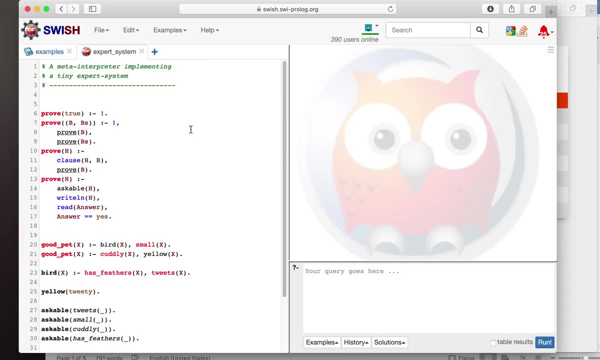 programs that are written And in the example programs you can see all of the programs you can see already opened. Okay, Oh yeah, here they are here. I'm sorry. You can click on things like the expert system. I think I had the movie database. 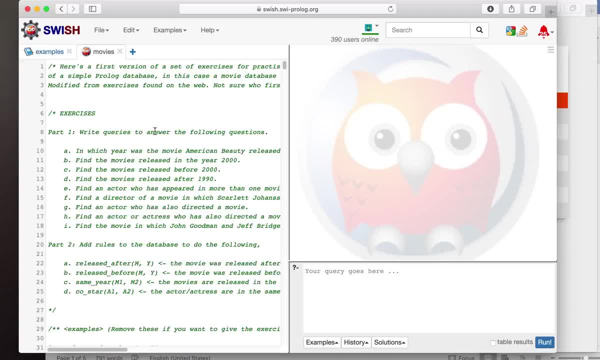 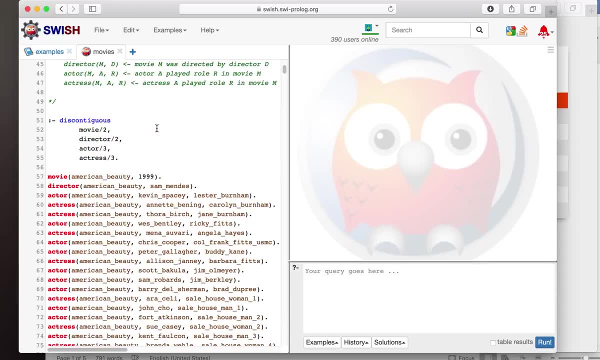 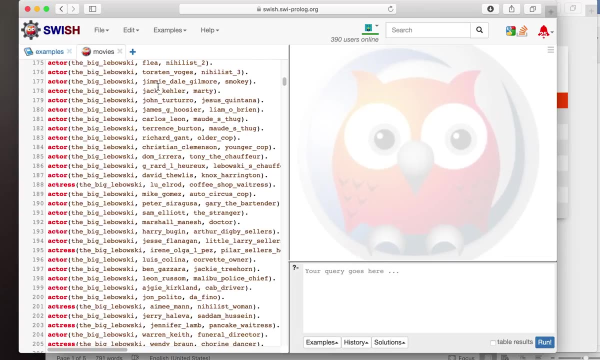 clicked on before Movie database And you can sort of see how what program looks like And there's a little explanations in here about how to write a prologue program. They're basically facts. Here's some facts- actually, These are examples of facts- And then there are some rules that are associated with it. Prologue is: 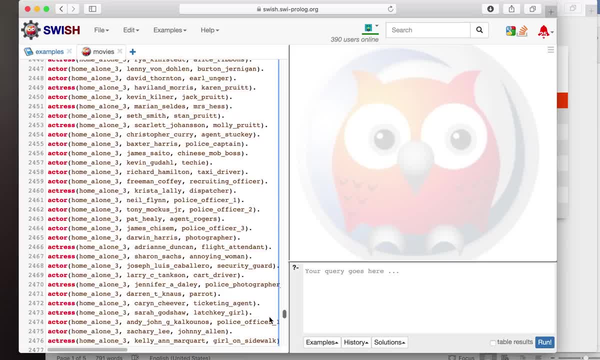 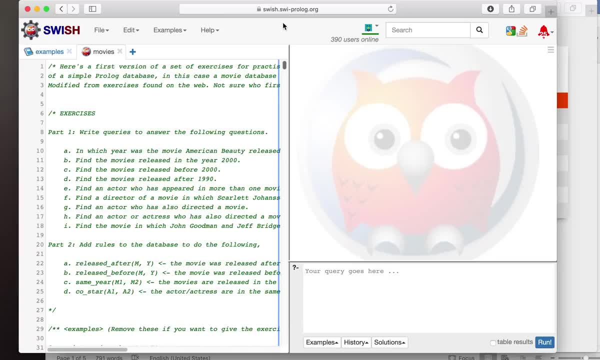 system Developing environment. Wow, there's a lot of facts in here. Wow, So this is a database of movies, it looks like. So you create a database And then you come over here and you ask it questions And the questions you might. 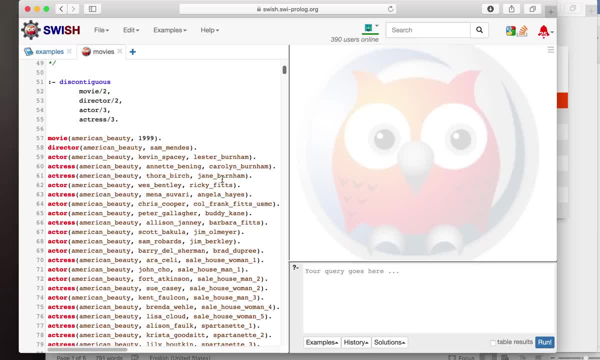 ask: is you know who, who, who played what actor played in this movie Or what actor played in that movie, So you can ask prologue questions And then prologue comes back with a yes or a no answer, Which is basically what you're doing. 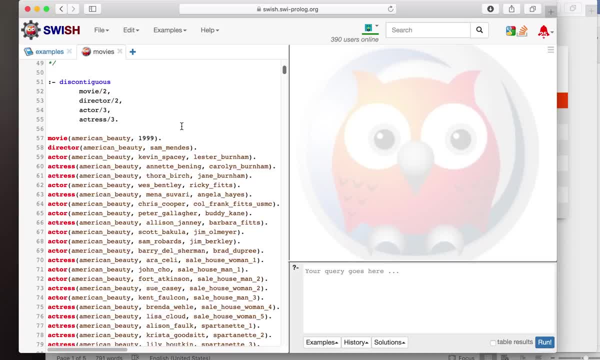 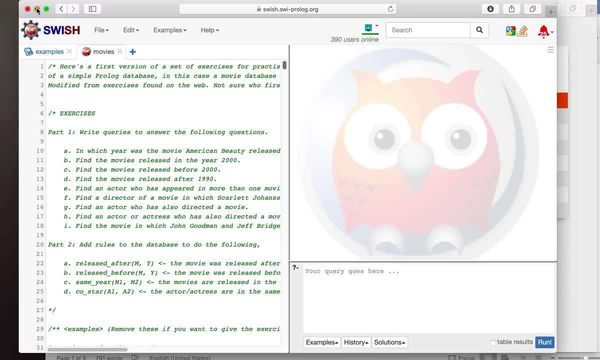 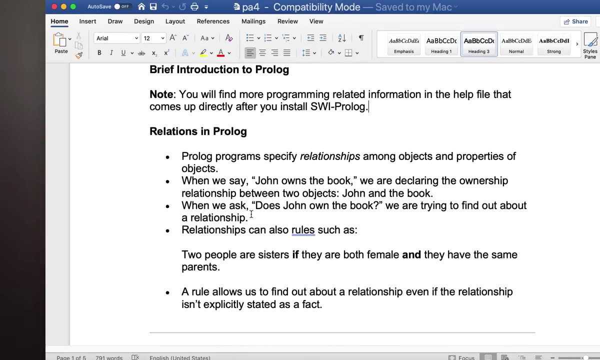 This is a, this is the programming environment, by the way, And this is a programming language. So in the lecture we're gonna see. momentarily I'm gonna go over how this works. Okay, let's go over the assignment next. So for the assignment In the assignment. it's kind of long, There's a. it's long winded. I. 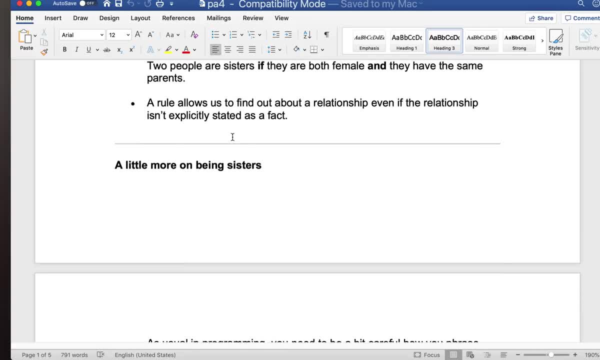 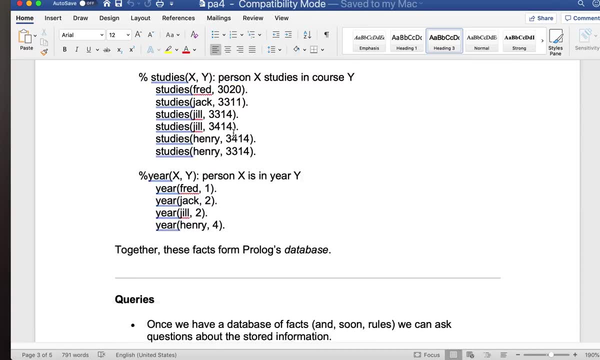 should say it's not really long assignment. There's a lots of explanation in the beginning here And there's programming and prologue, The idea of the fact, The idea of the rules, The queries, All this information, And then it says your. 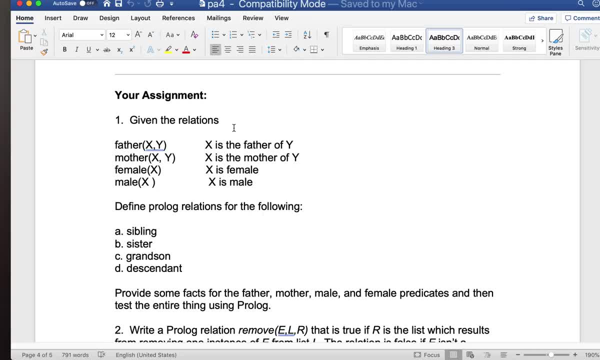 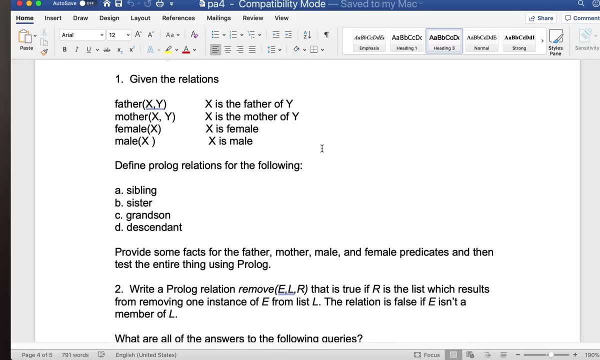 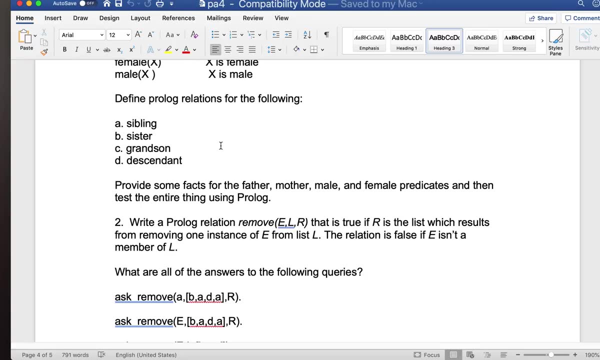 assignment right here. So your assignment is to answer five questions. The first question is: you're given the relations about father, mother, female, male, And you're going to define the relations for the following: Sibling, sister, grandson and descendant. I'm going to show you where that is actually in the lecture today. So 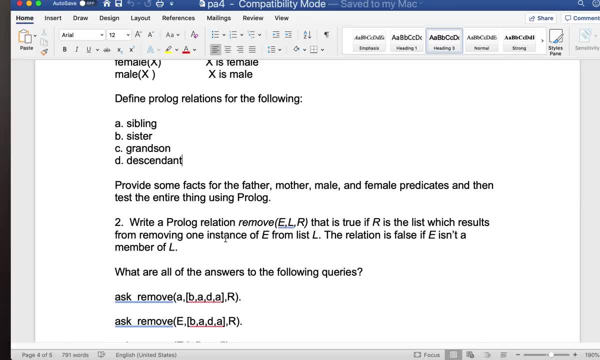 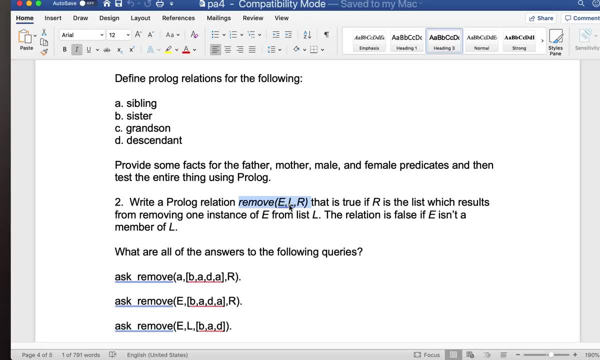 we'll see how that works. And then in number two you're gonna write a prologue relation Which is Relations are functions, And this one's called remove And it takes on three parameters: E, L and R. That is true if R is in the list, which results from: 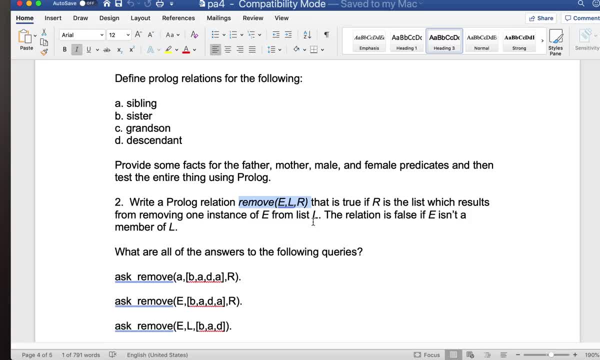 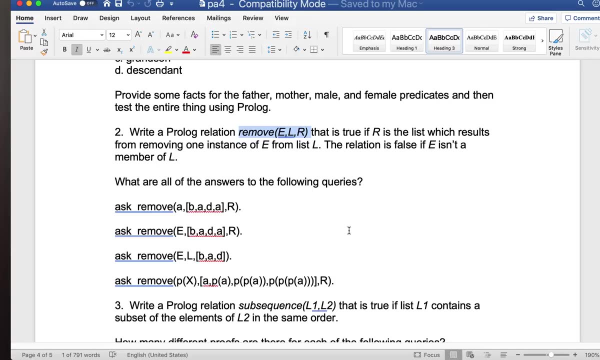 removing one instance of E from the list. So the relation is false if E isn't a member of the list. So if the element is in the list and you remove it, If the element is not in the list, then nothing happens, It returns false. And then 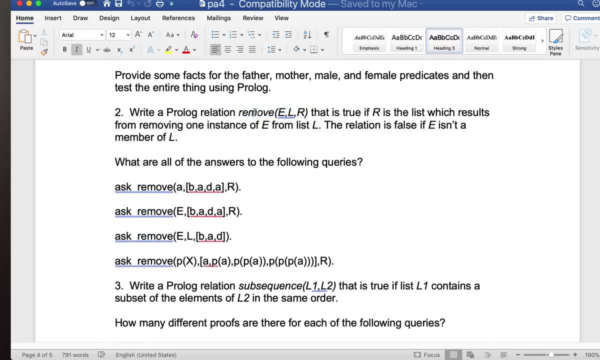 what are the answers to the following query? So you're gonna write this little relation, Which is actually quite simple, And then you're gonna run these to see: yes, no, yes, no, true, false, true, false Is really what's going to come out of it. 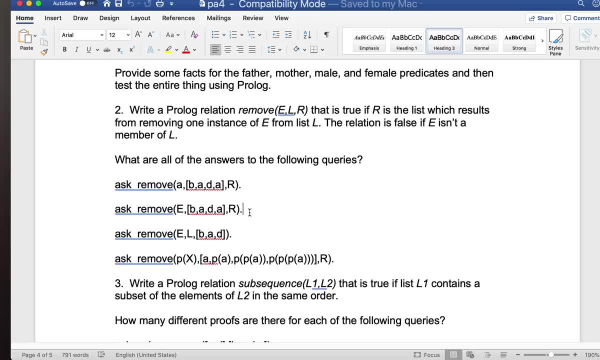 So the answers to the queries: This is going to be true or false, This is gonna be true or false, true or false, or true or false. So you answer those simple little questions And then, in number three, you're gonna write a relation. 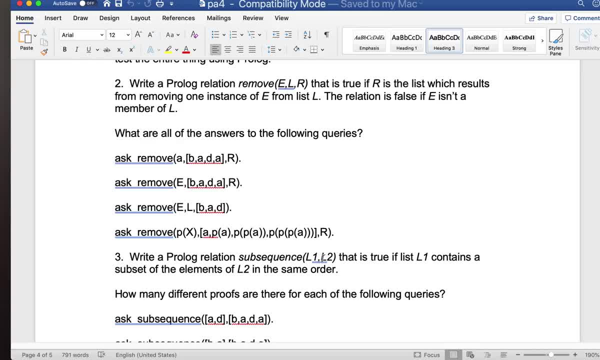 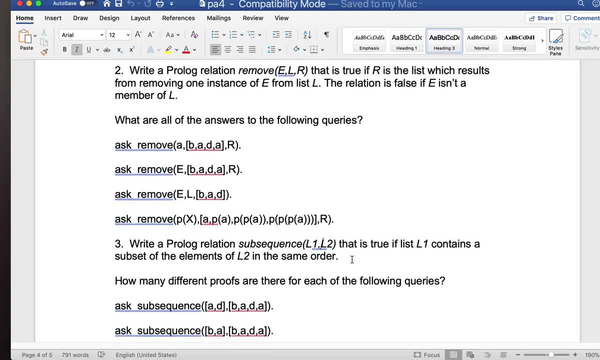 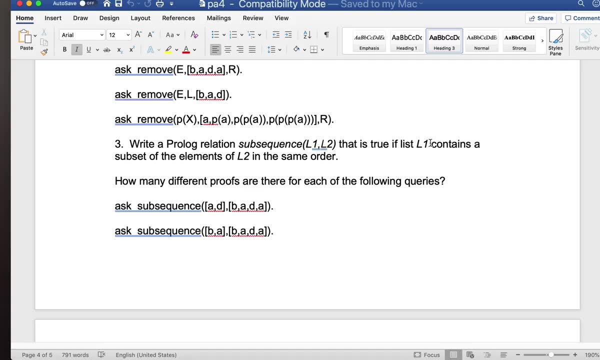 subsequence that takes on list one and list two Or L1 and L2 as parameters. And that is true if the list one contains a subset of the elements that are in list two In the same order. So if list one is inside a list two. So if list one 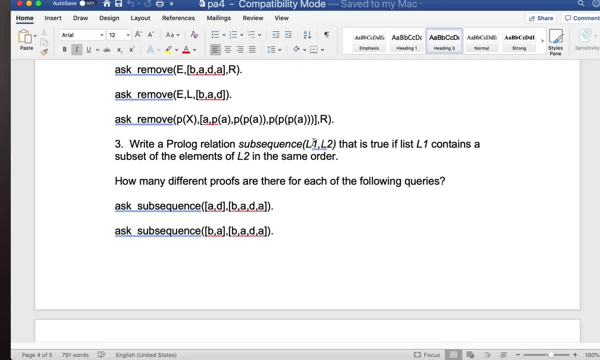 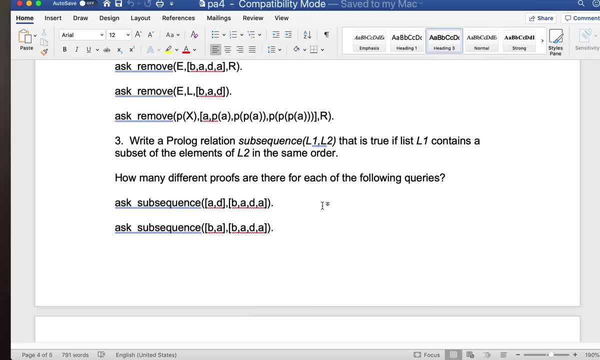 contains, or is actually the opposite. If list two is inside a list one in the same order, Then it comes back true. And then how many different proofs are there for the following queries? Well, I'm gonna talk about that too, But a proof means a. 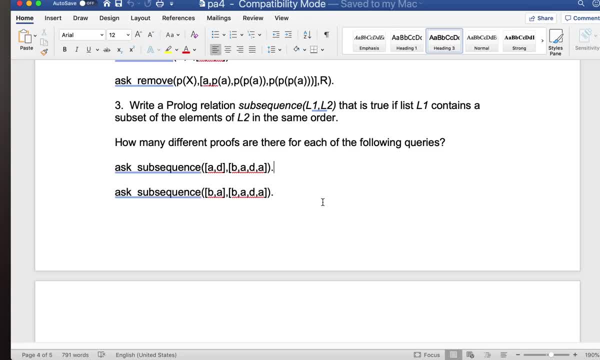 to ask it To try resolve it. And so, in trying to resolve it, the proof comes back true or false. And so in this particular case, it would come back multiple times true or multiple times false for every element. For example, in this particular case, you have a list one and list three, which is A and B. 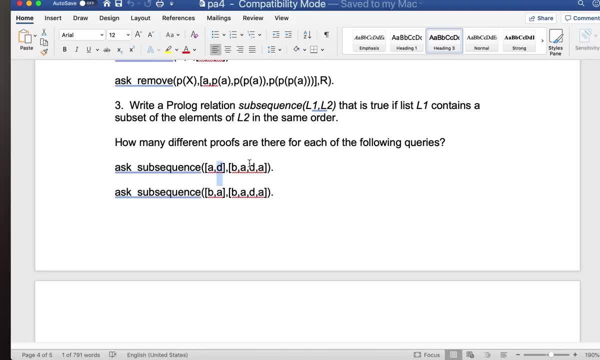 Excuse me, this is list one and this is list two. This is list one, this is list two, And it would have to check to see if this was inside of here And it would actually come back one time because it's going to find it right there. 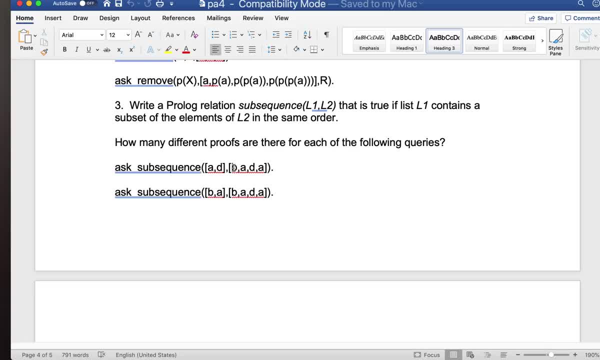 It's going to come back, true? Yes, it's there And the proofs is going to start with the first two and go: is it B, A? no, Okay then. is it A- B? yes, It would have two proofs. 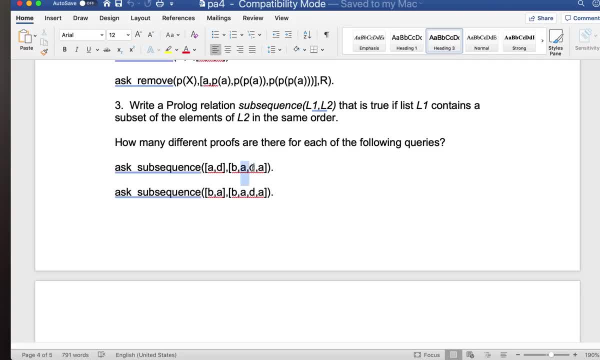 It would check twice and it would come back true because the list is found Here. it's going to come back one time because the list is found right in the beginning, Because the list now is B, A And then here we have a parameter X and Y. 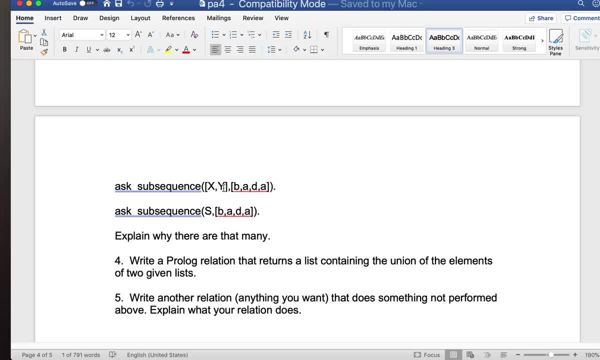 So it's going to have to check for one. two, It's going to have to check twice for the combination. So I don't want to give you all the answers here. I'll let you play with this one here too. This is an S is also a parameter. 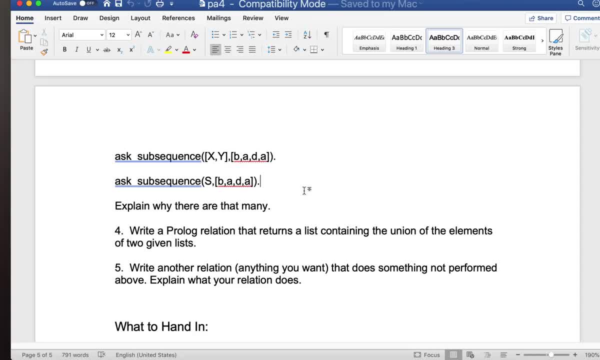 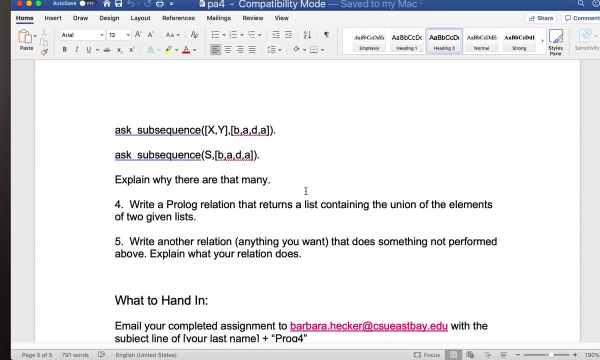 So explain why there are that many. Well, I just explained it to you, So I want to give you the entire assignment. So I'll let you explore that one a little bit more, But that's, That's what the question is actually asking. 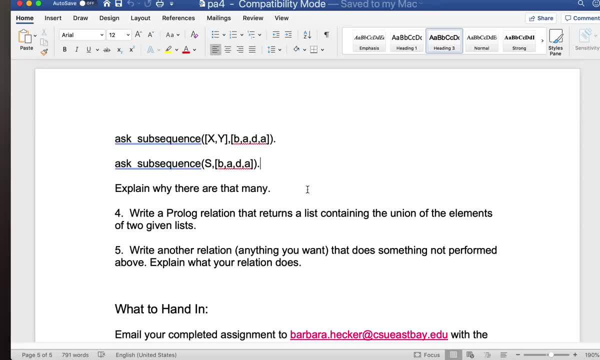 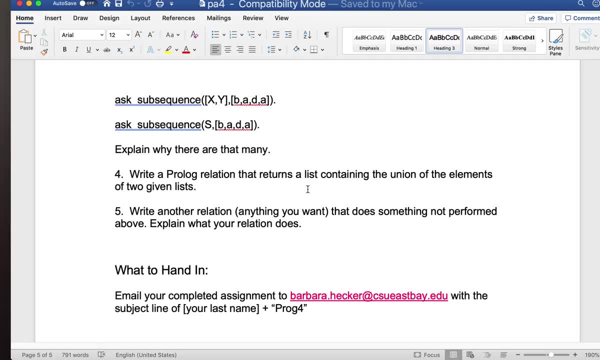 I gave you that information because it's kind of difficult remotely to answer that question on your own. So in number four you're going to write a prologue relation that returns a list containing the union of elements of two given lists. So you're going to write kind of like a scheme function. 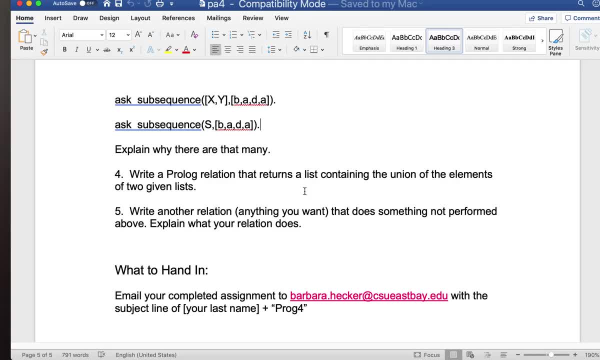 Prologue was actually made from Lisp, which is very similar to how scheme works, And so you can write functions in there too. They're really just called relations, And so this one's going to take. You're going to find two lists together. 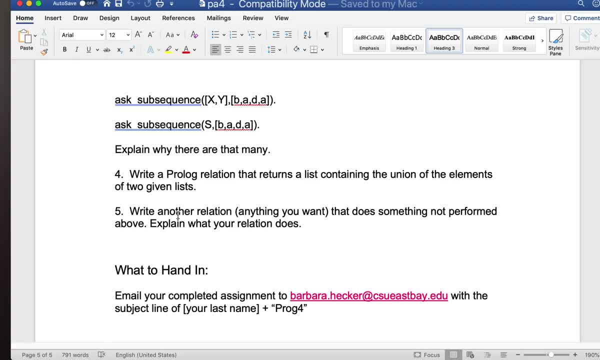 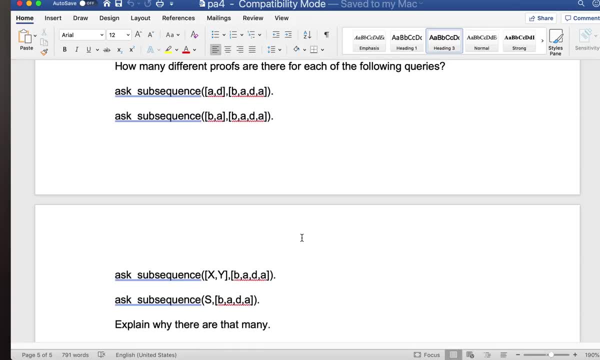 And then you're going to write another relation- anything you want that does something not performed above- and explain what the relation does, And then you're going to email it to me, just like usual. So I lied. I thought there were five questions. 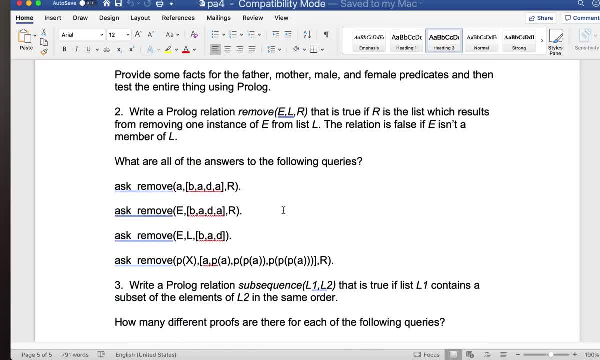 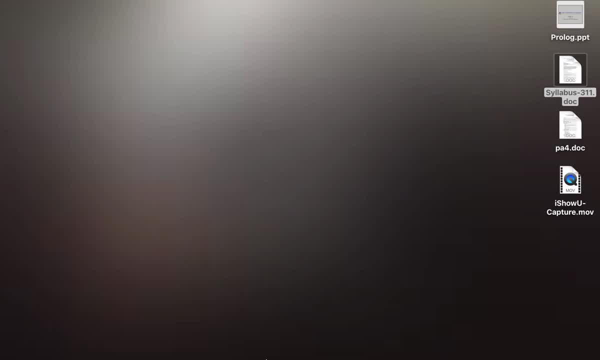 Oh, there are five questions. Okay, I didn't lie. There are five questions that are worth one point each, So have fun with this assignment, though It should be fairly easy, And so what you're going to do then is: 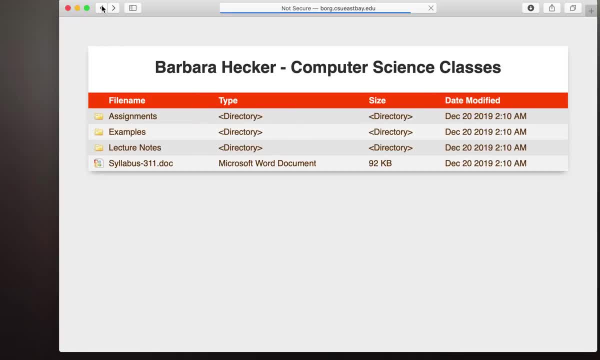 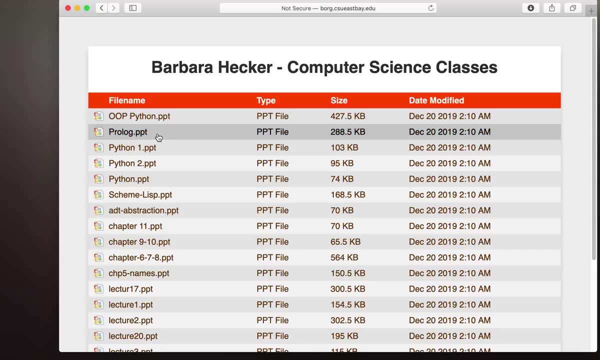 Complete the assignment. And in order to complete the assignment, you're going to need to learn a little bit about Prologue, And we're going to go over right now the Prologueppt lecture that is in the lectures folder: Lecture notes. 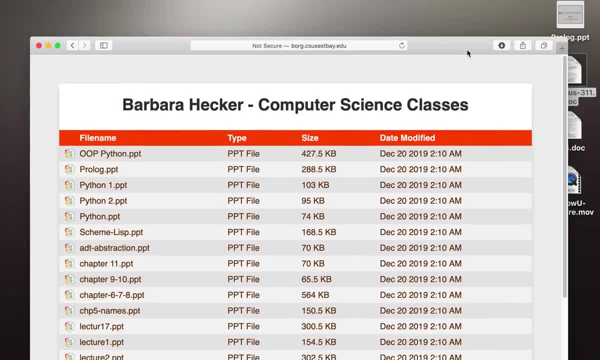 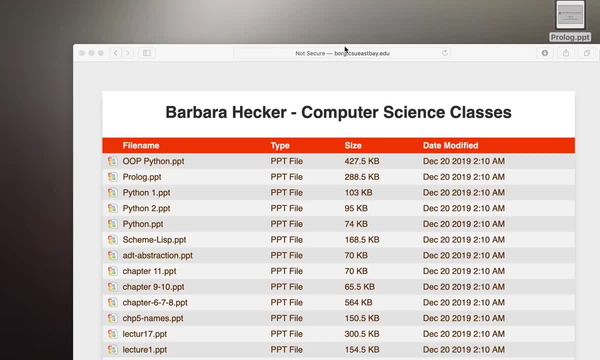 Prologueppt. I have. I thought I downloaded it. I did. It's right here, Prologueppt, And I'm going to load it up And I'm going to spend the rest of this particular lecture going over Prologue. 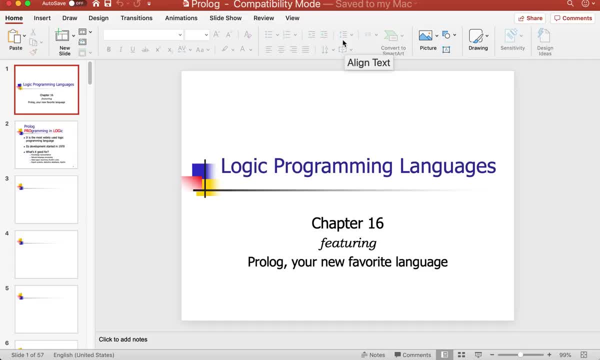 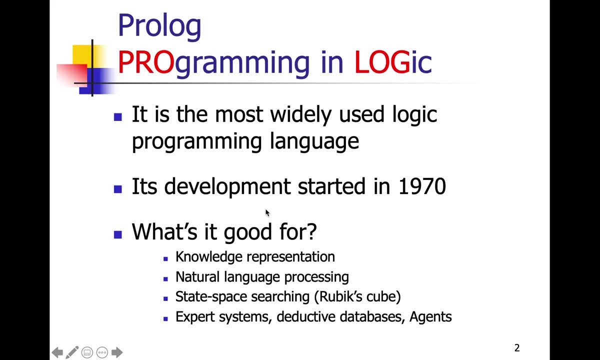 And then we'll start on a new topic for the next lecture. All right, So Prologue. Tell me about Prologue. Prologue stands for programming logic, So P-R-O is programming Logic, is L-O-G- Prologue- That's where the name comes from. 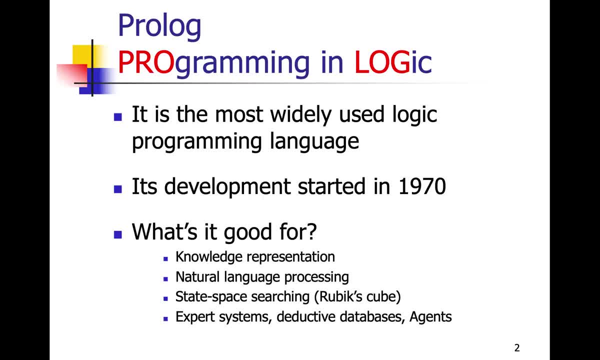 It was widely used programming language, Still widely used today. It's widely used on the internet as well. It was developed in the 1970s. What is it good for? AI- Artificial intelligence. It's used a lot in AI for expert systems. 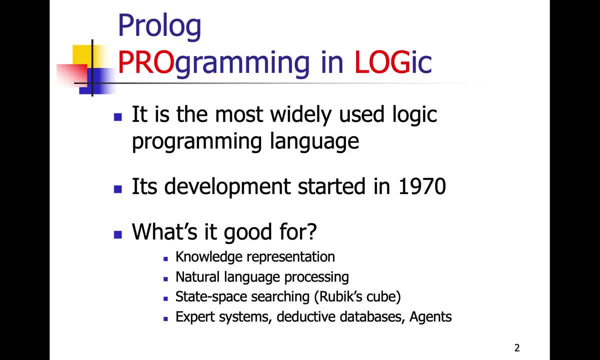 Well, what's an expert system? An expert system is a database that you can ask questions of. Remember the magic eight ball? It's a kid's toy. You shake it around and you ask it a question And it comes back with one of these weird answers: like you know, shake the ball. 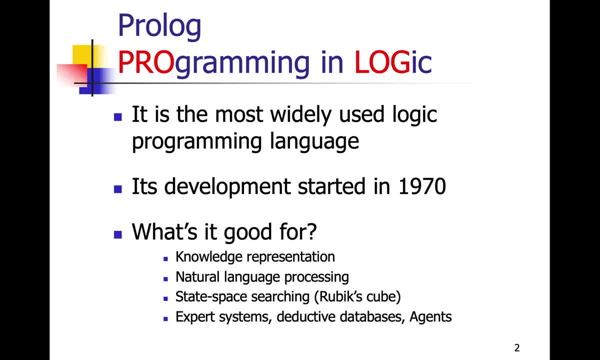 Am I going to catch the coronavirus? And it would come up and it would tell you: oh, probably not, Or ask again later, Or yes or no. It would come up with an answer for you. That's prologue. Prologue is the magic eight ball. 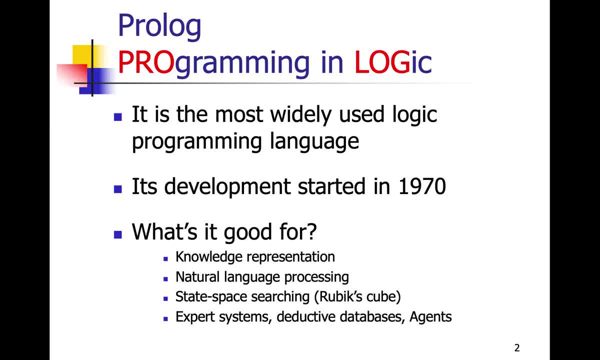 And so to make it intelligent, we load it up with information, So we build it with a bunch of facts, Like just because you live in Santa Clara County, you're not going to catch the coronavirus, And so it would use that as logic. 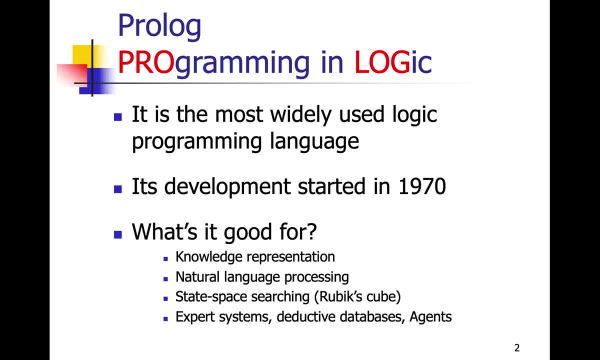 So it would have asked: am I going to catch the coronavirus? And it looked for the fact and it found: oh, just because you live in it doesn't mean you're going to catch it. All right, cool. And so then it would use that piece of logic. 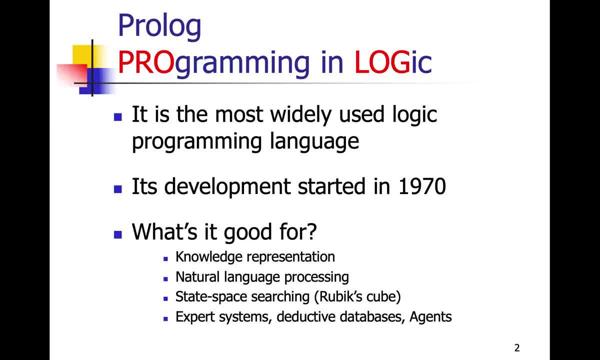 Or it would use another piece of logic that you'd put in there. that would say something like: but there's been 40%, 4,000 cases or something. I don't know how many cases there are, But there's been X number of cases. And when X number of cases gets to a certain level and the cases get beyond 1,000, then the likelihood of you catching it goes up or something. I don't want to scare anybody here. That's not really true, So you get the idea, I hope. 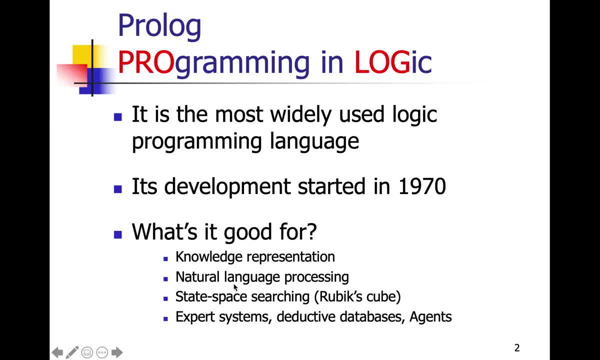 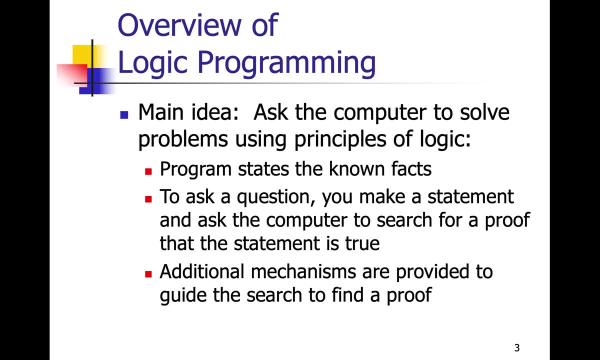 It's used for knowledge representation, natural language processing, state-space searching like the Rubik's Cube, expert systems and deductive databases or intelligent agents. Take an AI class and you'll see Prolog used a lot for those particular areas. This is not an AI class. 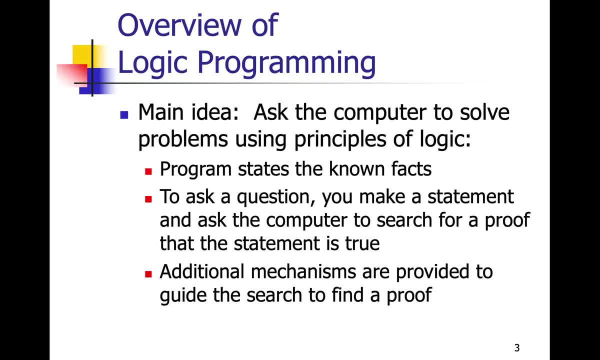 This is a programming language concept, So I'm not really going to go through all of the AI stuff, But that's a fun class. That's a fun class you might want to take in the future. So the overview: you ask the computer a question and it solves it using principles of logic. 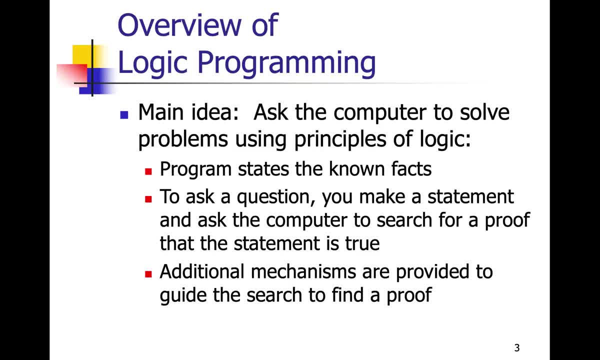 So the program states the known facts. You ask it a question, You make a statement and ask the computer to search for a proof of the statement to see if it's true, And then we have different search strategies that are used. Okay, so this is what's called a declarative programming language. 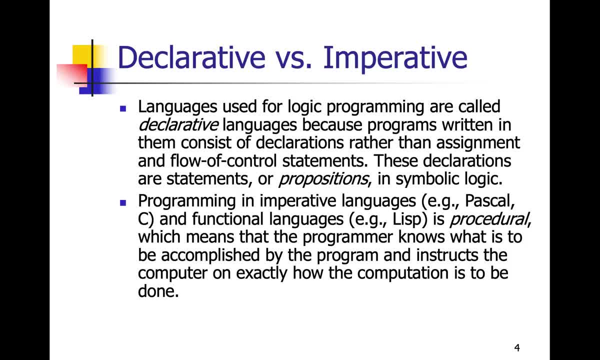 You guys all remember from the midterm we had imperative programming languages And I asked you what some features of imperative programming language is. And the flow of control is programmed by the programmer. The programmer figures out how the program is going to run from start to end. 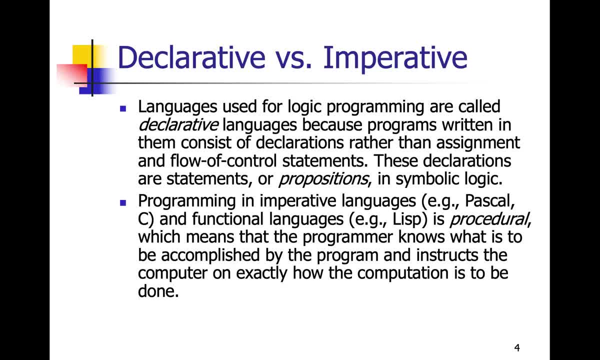 And that program always runs the same way every time you start it. We have variables in there, We have iteration, We have recursion, flow control. We have all that stuff in there. Now, declarative languages: that's Prolog. Prolog is a declarative language. 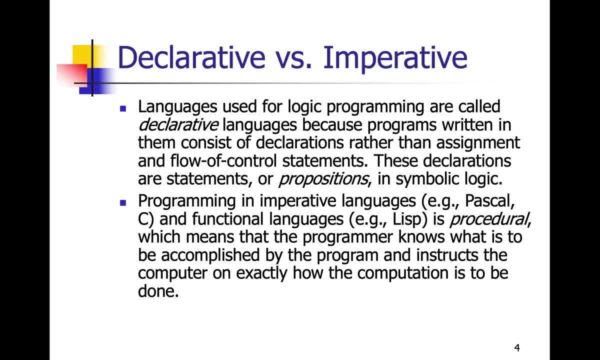 We make declarations, We don't have variables. We don't tell Prolog how to work. Prolog knows how to work itself. Prolog knows how to run its own programs. We just use the mechanisms that are given to us And we supply it with facts and rules. 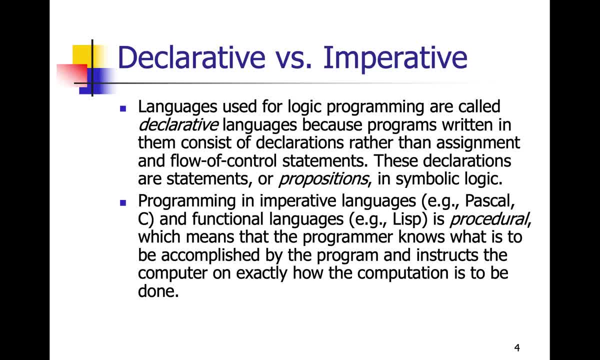 And we let Prolog run the way it knows how to run. So we're not programming that stuff like we would in an imperative language. So we have propositions and symbolic logic that is used to create programs In Prolog. So that's what it means by being a declarative versus an imperative language. 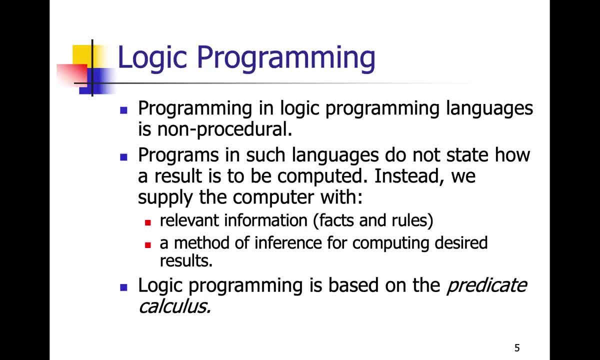 Now, logic programming is not procedural. We don't tell it how to proceed. The programs don't state how the results are going to be computed. Instead, we use the built-in mechanism. So it's supplied for us. We give it relative facts and rules. 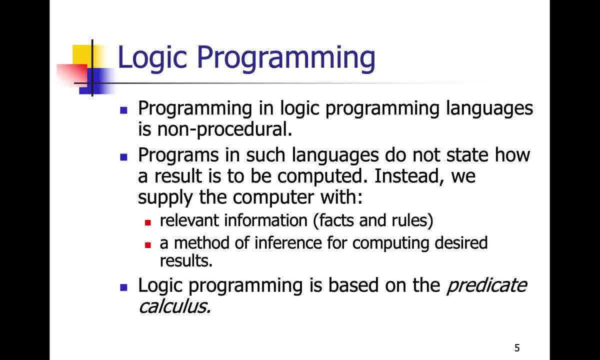 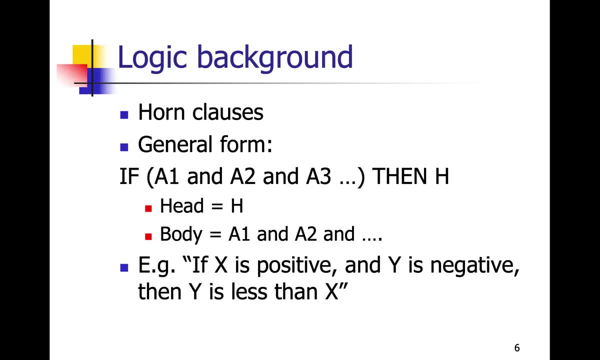 And then we have a method for inference that is done for us by default By the program And that's what Prolog is actually doing for us. So it's based on predicate calculus as another way of describing it. So here's kind of an example. 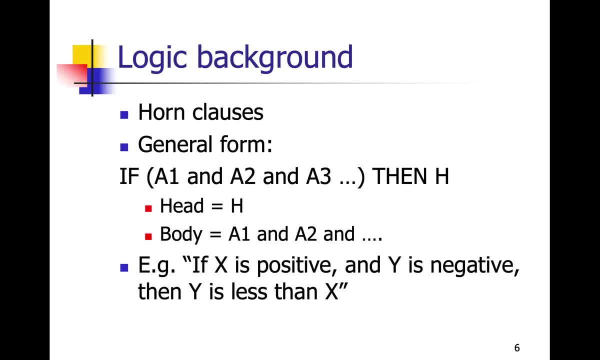 This is not Prolog syntax. I'm going to show you Prolog syntax momentarily. This is the theory behind the logic background. And if you just look at the bottom bullet point where you say: you know, if x is positive and y is negative, then y is less than x. 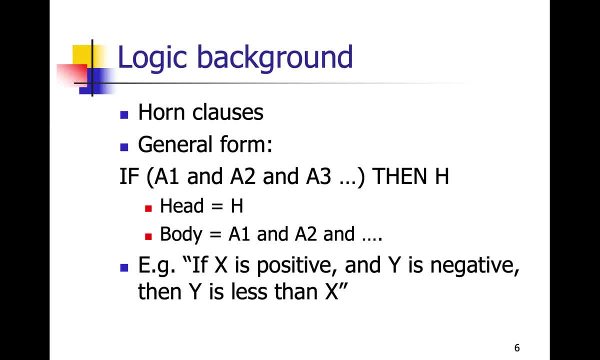 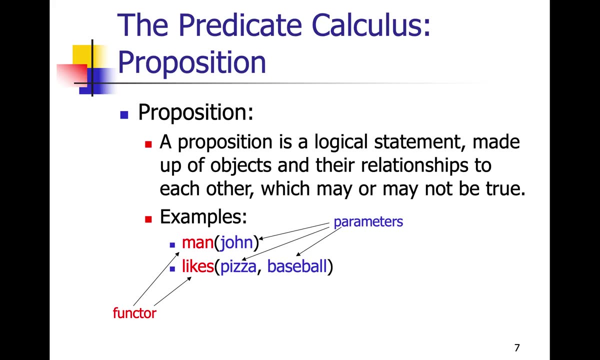 Well, that makes pretty much good sense, Which is how we're going to put facts and rules together, to create statements or horn clauses that will tell us information that is true or information that is false. So the predicate calculus, the proposition itself, is made up of the objects and the relationships to each other. 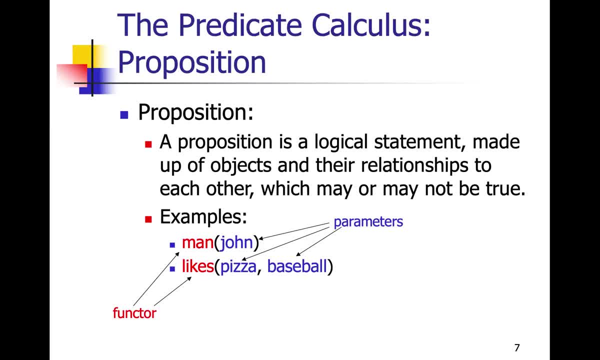 For example, these are called functors. They kind of look like functions, but they're not functions. They're functors. They have a name. The name is in red And they have parameters. The parameters are in blue. For example, man John likes pizza and baseball. 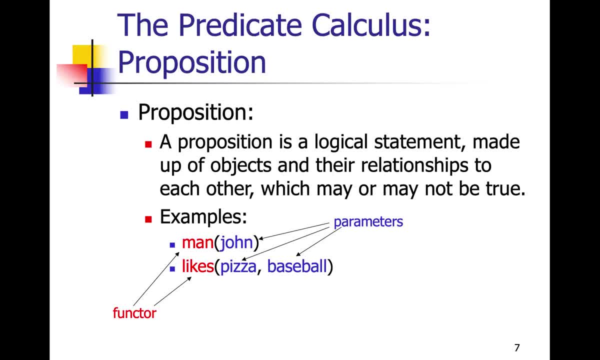 So the first thing: most students look at this and go: man like. I know what a man is and I know what likes. I know what likes means And you have this English kind of definition for these particular words and there's some symbolic meaning to you when you say likes. 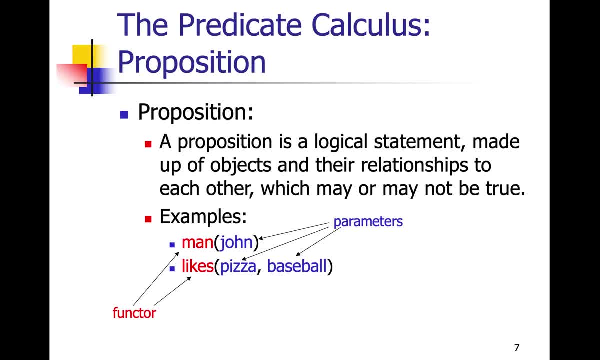 Oh, likes pizza baseball, You know, hates coronavirus. So that syntactic kind of meaning that comes along with it is part of the English language or part of the understanding. Okay prologue doesn't actually use that Prologue, doesn't know what likes means or what man means. 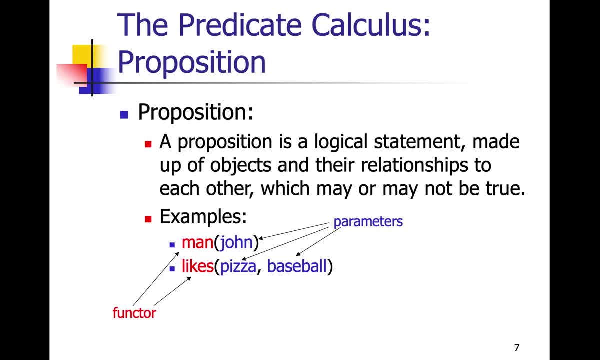 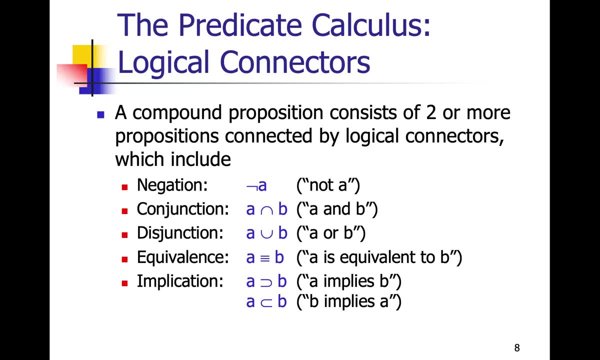 Prologue only knows that these are constant words or expressions that are used with absolutely no meaning associated with them. So keep that in mind as we go through Some of the examples and you'll sort of get why. there's no meaning, There's no hidden meaning behind any of the words. 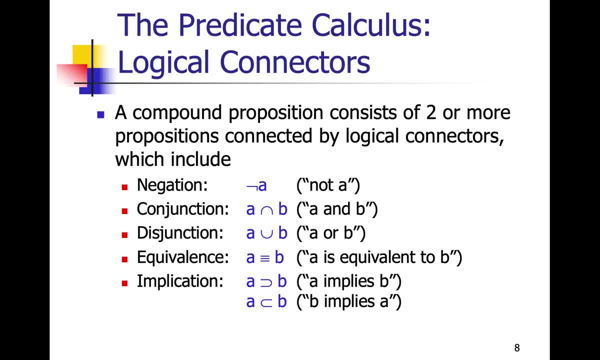 There's no symbolism with any of the English definitions of these words. You can use like A, B, C if you wanted to. So then we put things together. So a compound proposition consists of two or more propositions connected by these logical operators. 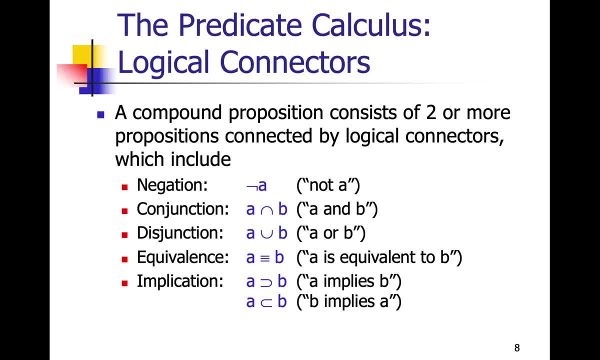 All right, go back to discrete math and review kind of what's going on there. The negative, the, not the conjunction A and B. A or B. A is equivalent to B, A implies B, B implies A. It's the same thing you learned in discrete math. 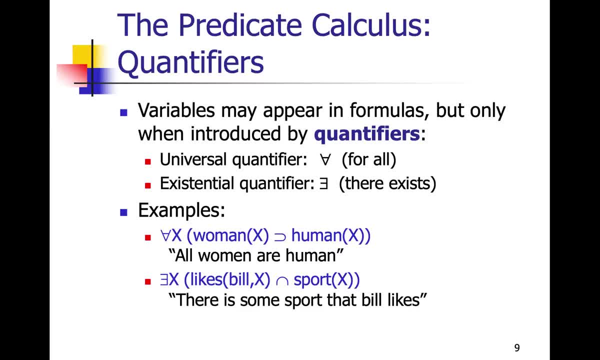 Well, hopefully you learned it in discrete math. And then also the qualifiers, So the universal qualifier, the existential qualifier: There exists or there does not exist, Or, for all You know, for all women are human. I would hope so. 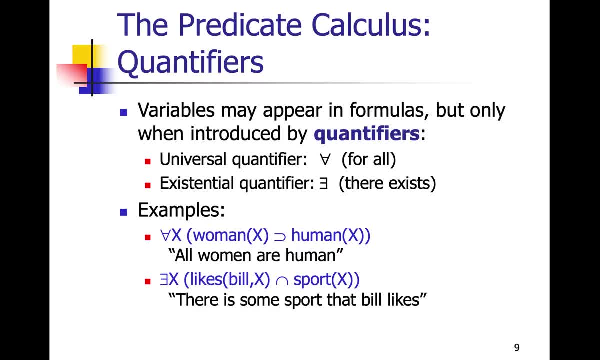 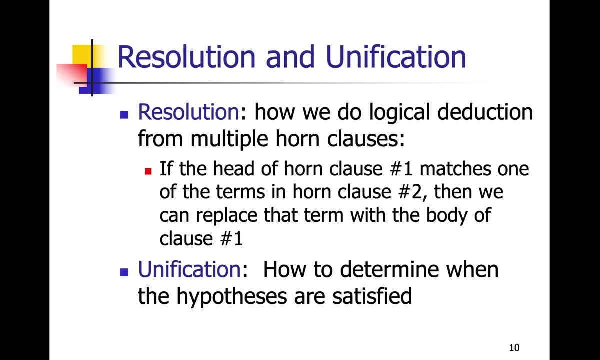 There is some sport that Bill likes. We don't know which one it is, but there is a sport that Bill likes. So you could put together, using these quantifiers, as they are called, to make more elaborate expressions, And only the concept of resolution and unification to resolve something. 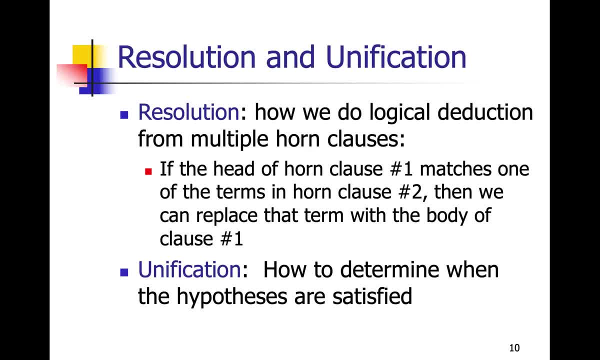 is how we logically deduce from multiple horn clauses. So we start at the beginning and we go through the problem To resolve it, To unification is we determine when the hypothesis are satisfied. You can sort of see, think of it like sort of like backward and forward chaining. 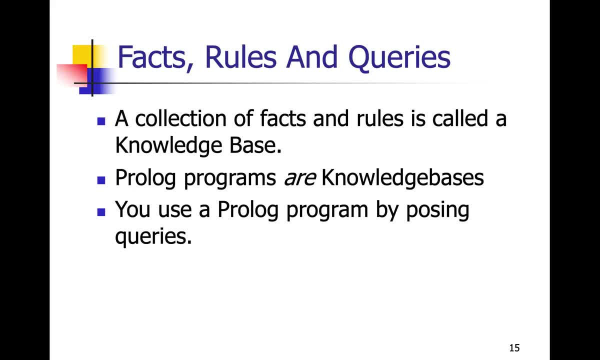 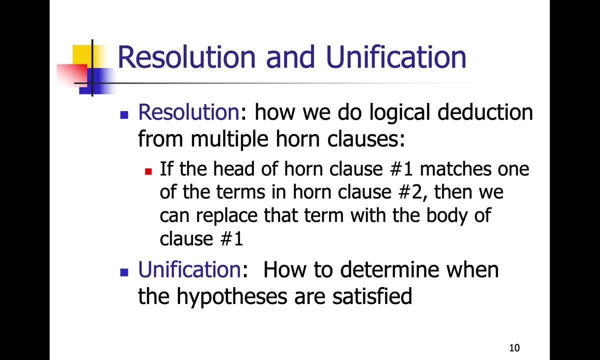 which is actually coming up, I believe One of these slides coming up here. we're going to have this concept and maybe I'll just do it now so I don't have to do it later, Backward and forward chaining If I went forward to solve a problem, to resolve it. 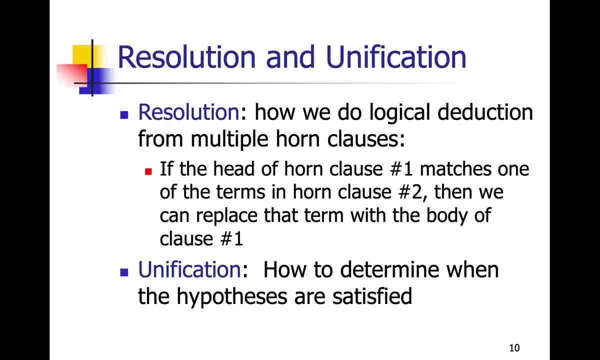 I would ask the question, and actually I'm looking at my window here. I'm looking at my window, Actually I'm looking at my window right now and I'm looking at these clouds and the question I'm going to ask is: is it going to rain? 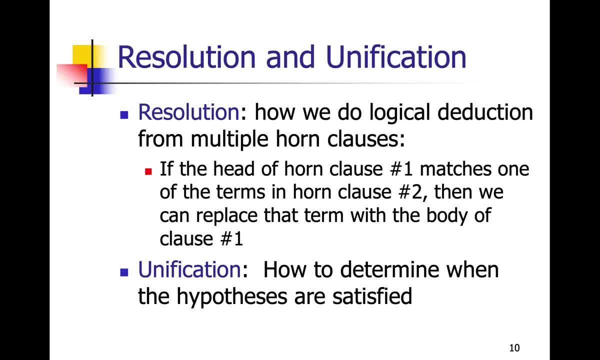 Yeah, I'm just going to say: is it going to rain? I'm going to ask Prolog this question and I'm going to have Prolog answer this question for me, doing a resolution process To resolve the question and answer it for me with a yes or no. 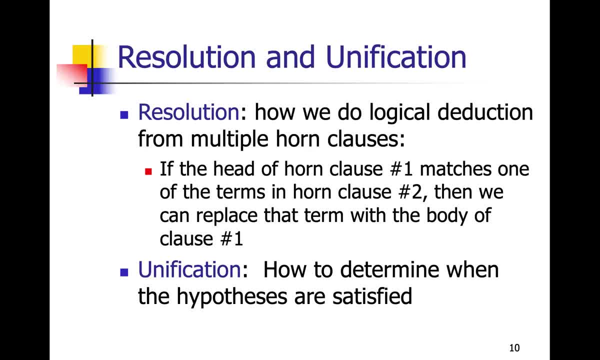 is it going to rain? Prolog is going to go through the database and say, well, are there a lot of clouds? Yeah, Did it rain yesterday? Yeah, Is it on the forecast for today that it's going to rain? Yeah, 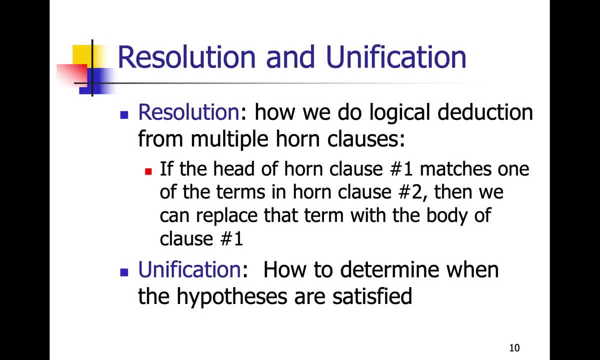 Do we have some darkness going on right now? Yeah, Then Prolog is going to come back after looking at all these things and it's going to conclude with yes, it's going to rain. I guarantee it. By the time I end finish this recording of this video. 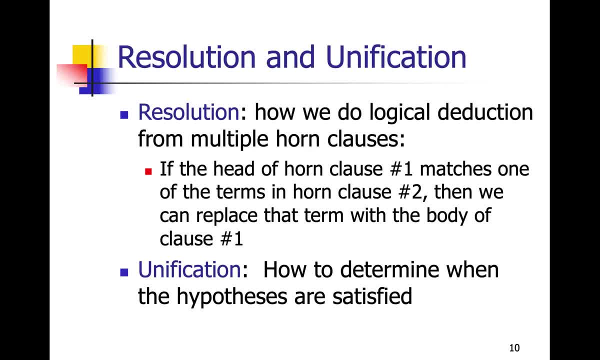 I'm going to see raindrops coming down. It's just a matter of time. So Prolog would probably come back. if Prolog had all that information stored inside of its database, It would come back and say, yes, it's going to rain. 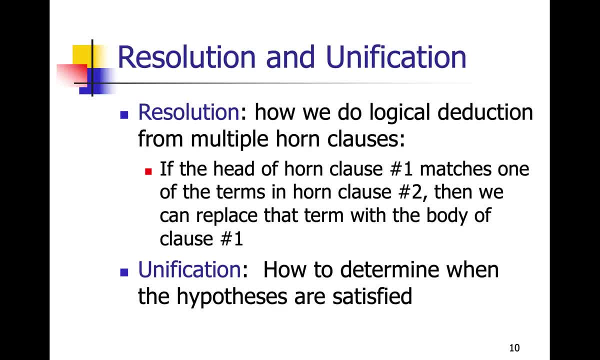 Okay, Unification kind of says: is the hypothesis, true The hypothesis? So I would say, instead of asking Prolog, is it going to rain, I would say Prolog, a definite statement: it's going to rain, Or Prolog, it's not going to rain. 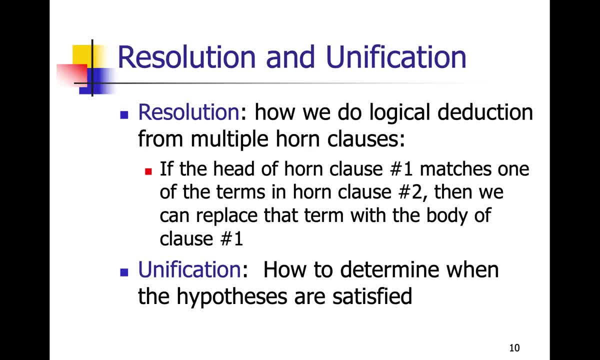 And Prolog would come back with false or true, If I was correct or not correct. So instead I just state the conclusion and then I try to find out. Prolog tries to find out if the conclusion is true or false, So it's called backward chaining. 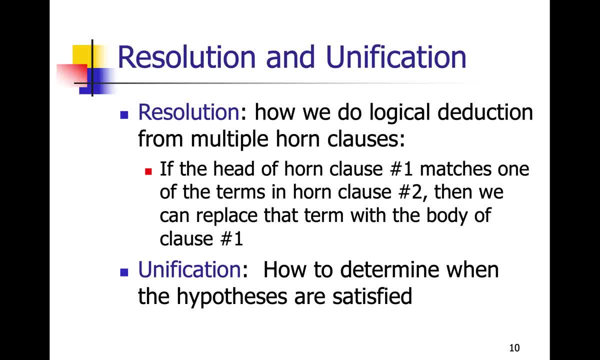 where I go backward from a conclusion to see if it's true versus a forward chaining. that says: here's my question. I don't know if it's true or false. You tell me if it's true or false. which is a forward direction versus a backward direction? 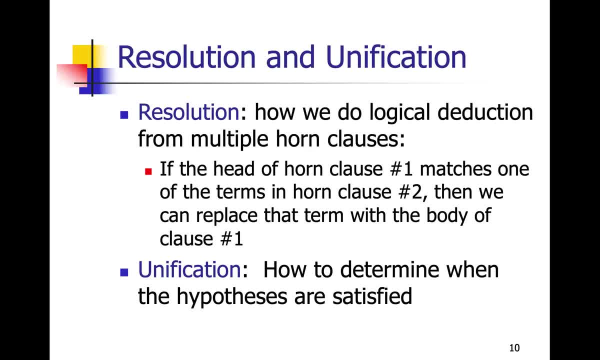 So, in a backward direction, we're going to say you know, we don't know, It's going to rain, Prolog it's going to rain. And it comes back and says, yes, Prolog, it's not going to rain. 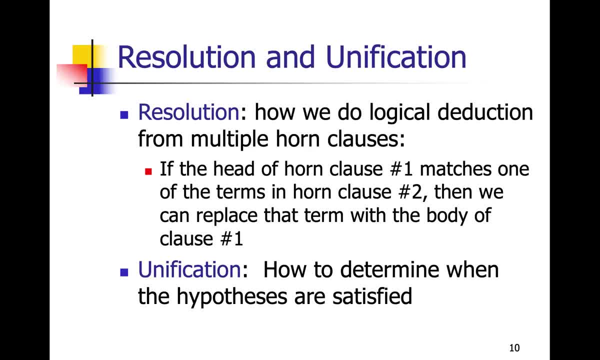 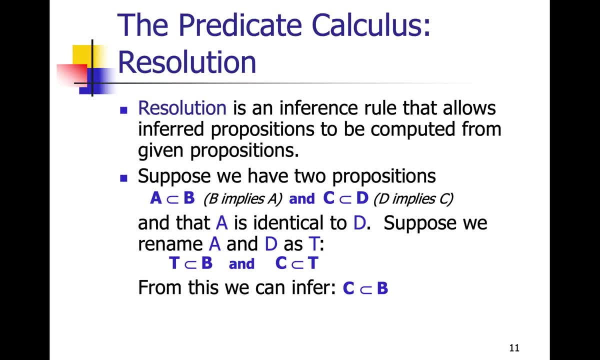 And it will come back and say: no, it's going to rain. So, depending upon what's going to happen, So I don't know if it's going to rain or not. So if we go through these resolution process and we look at how these inferences are actually going to be made, 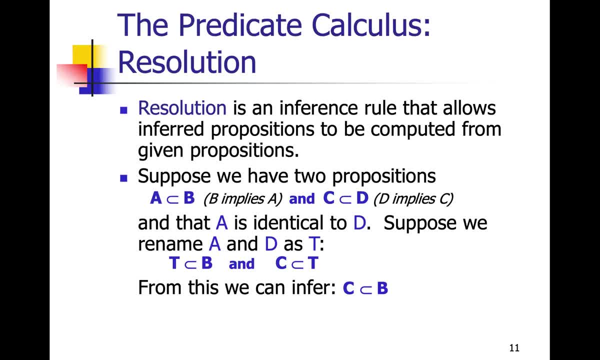 and lucky for you, you don't have to program these inferences. They're done for you automatically And Prolog uses a theory- It's called forward chaining by default. You can change the resolution process, but you don't actually have to. 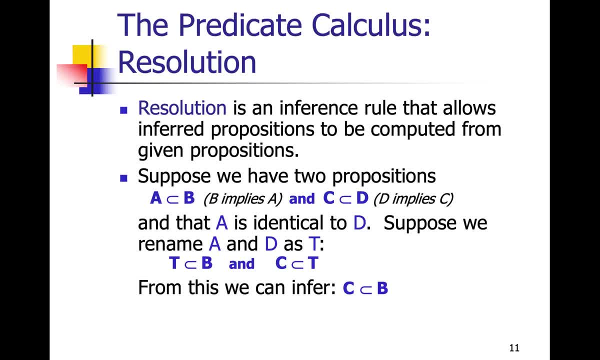 You can leave it on default settings, And Swishy doesn't actually allow you to change it, It just uses both interchangeably, depending upon how you've got it programmed. So suppose you have two propositions, that B implies A and you have that D implies C and that A is identical to D. 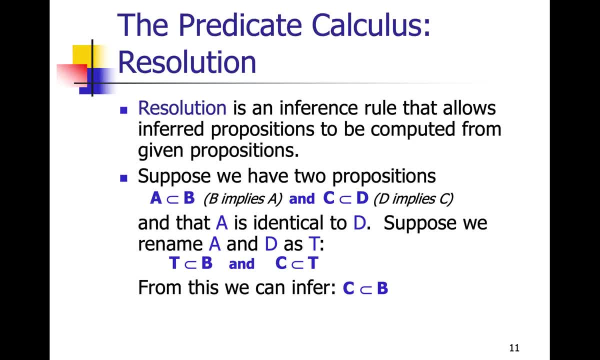 Then you suppose you rename them A to D as T, And then you can infer. So you can infer that C, you know, C implies T. Therefore, well, T must imply C. So you can infer that B implies C by substituting in: 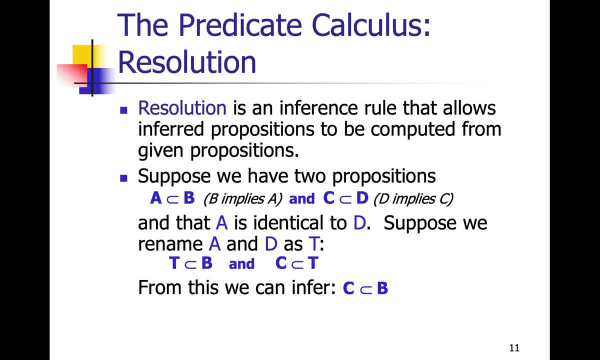 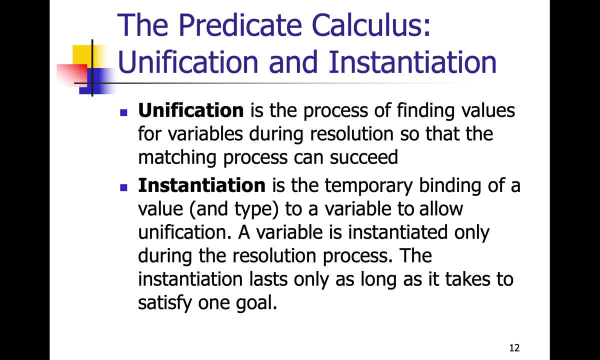 And so it's very similar to, you know, a mathematical calculation with substitution, and you're substituting in one for another. So unification is the process of finding the values for the variables during the resolution so that the matching process can succeed. So we bring it together. 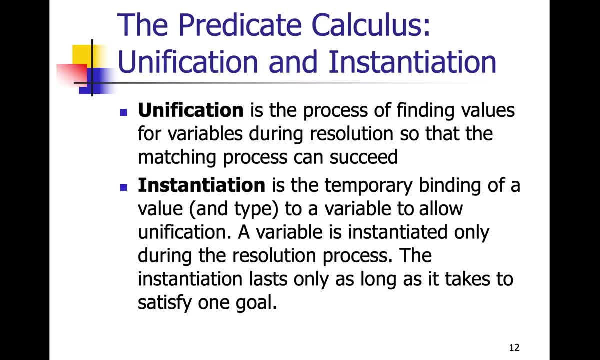 We unify it, We bring it together, And these work with the forward and the backward chaining as I just described. So the instantiation is the temporary binding. So you're like I thought you said we didn't have any variables. Eh, we don't. 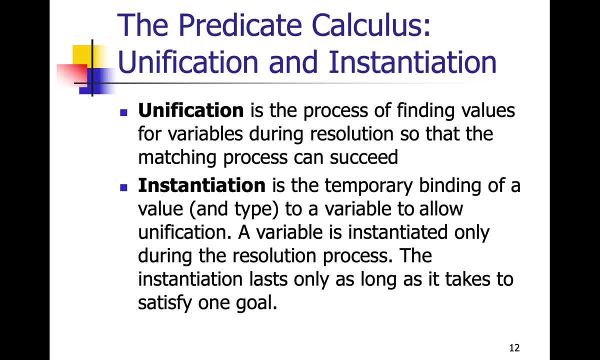 They don't call them variables. They call them instantiations. So we have X or we have S. We don't define them as variables, But we use them as instances or as temporary placeholders for data. We keep the data and then we use the data throughout the process. 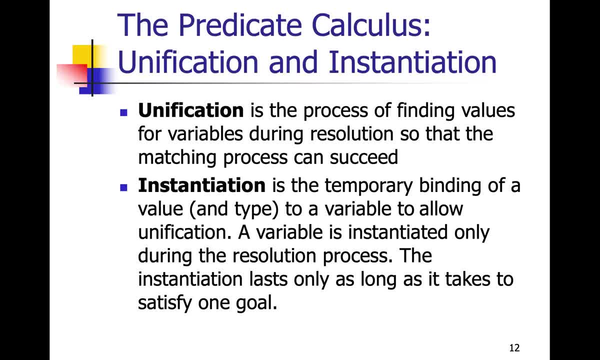 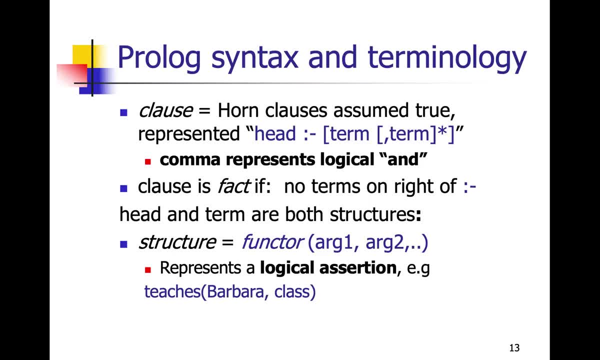 so that you know we don't have to keep repeating it and getting the data. We have a placeholder for it. So we have this instantiation that happens to allow us to hold on to the data, to the current states. So, with our terminology, here we have the logical AND. 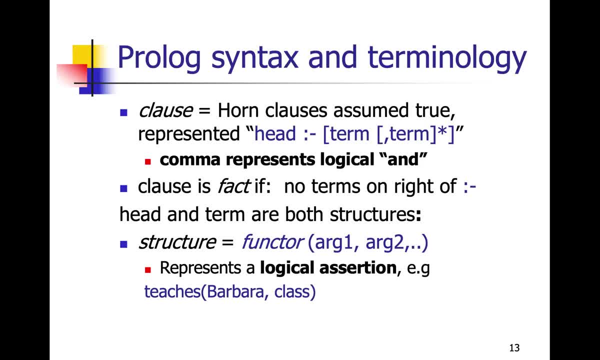 We have the logical IN. We have the logical assertions that occur here in a structure. So what we're looking at here, this is the structure that you're going to be more familiar with. It's the functor structure. See, even on video, I can't talk. 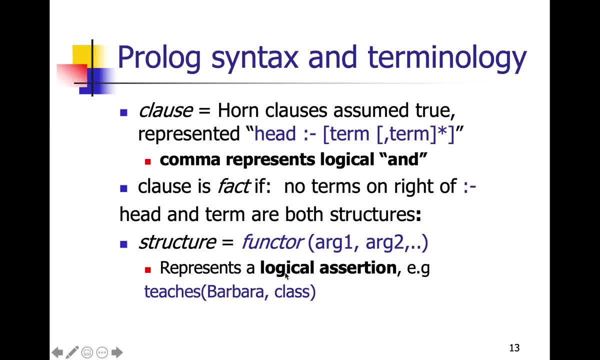 So teaches Barbara a class, which I'm trying to do. We have a functor or a fact- I like to call them facts, but they're really functors. This crap up here is just showing you how it works, just showing you how to put it together. 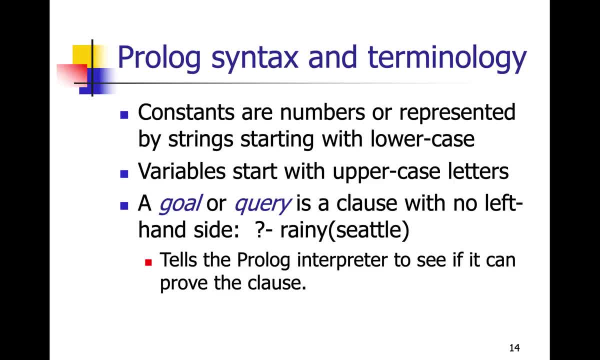 So we'll see some examples here and make a little bit more sense. And then we're going to have a question mark where we're going to actually run the program. So when you write a Prolog program you create a database. When you run it you ask it questions just like the Magic 8-Ball. 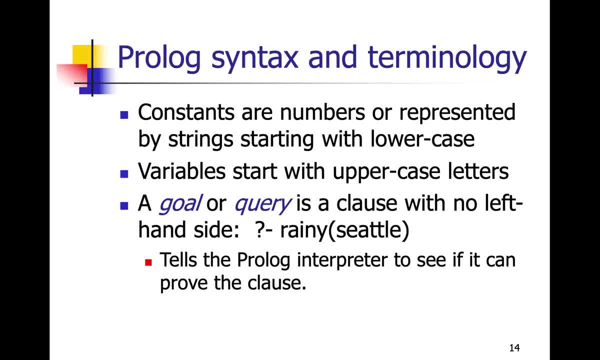 How do you use the Magic 8-Ball? Well, you shake it up and then you ask it questions. You don't have to shake up Prolog. You probably could if you wanted to, but you don't have to shake Prolog. 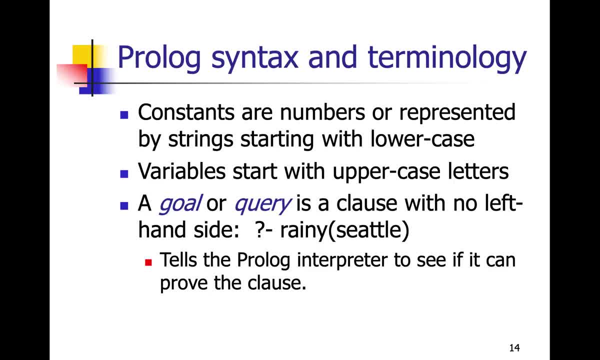 You just load it up, You just start it and then you ask it questions. That's how you run it. So the variables start with uppercase letters, remembering that Constants are numbers that represent strings in lowercase. We'll see some examples and I'll point this out in the examples. 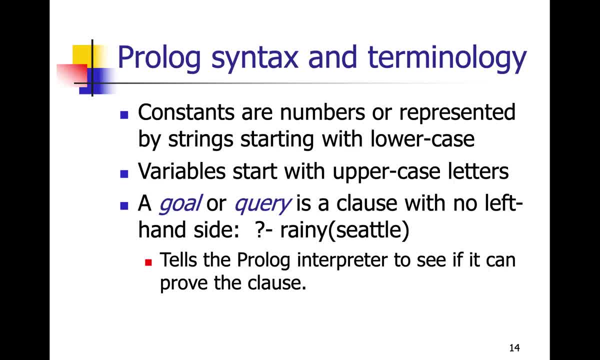 The variables always start with uppercase. The goal or the query has no left-hand side, So raining in Seattle, you'd write this at the prompt, The prompt being the little screen in the shell. It tells Prolog to interpret to see if it can prove the clause. 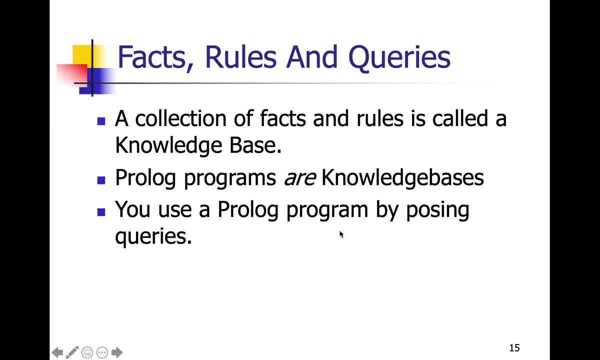 If you wrote this in and you actually had this fact, it would come back with yes, So all we have are facts, rules and queries. So their collection of facts and rules is called the knowledge base And Prolog programs are called knowledge bases. 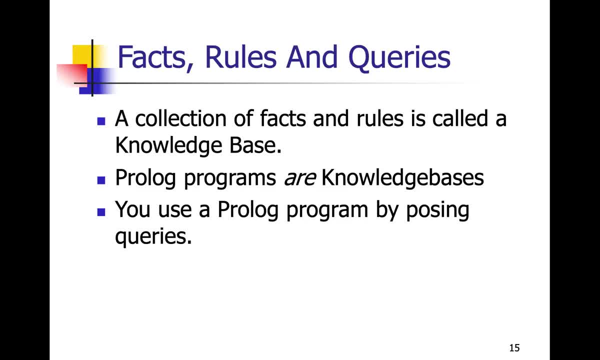 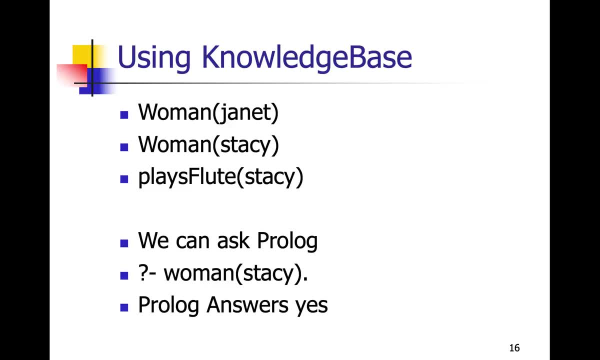 And we use Prolog programs by posing queries. We run them. So we use them or we run the program by creating a query. So here's an example of the knowledge base where we have woman Janet and we have woman Stacy and plays flute: Stacy. 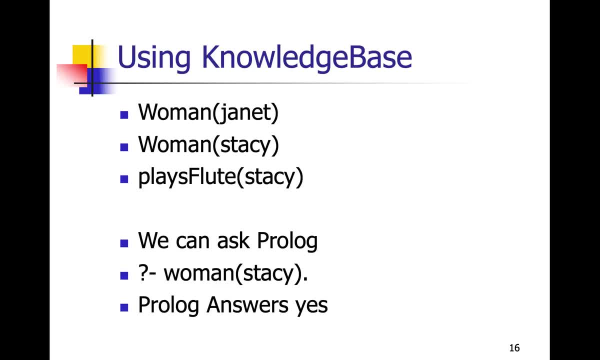 And so we can ask Prolog woman Stacy. And Prolog comes back and says yes, because it's in the database, It's in the knowledge. Plays flute, Stacy. Prolog comes back and says yes, Plays flute, Mary. Prolog comes back and says: are you kidding me? 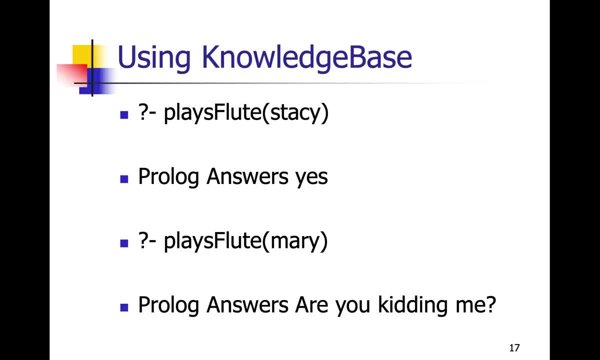 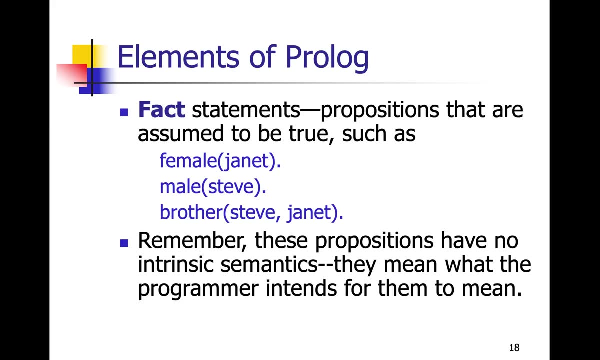 No, it doesn't say that, It just says no. You could program it to do that, But it's very difficult and it's not worth your time. But yeah, So it tries to put things together. In this particular case, these facts are statements. 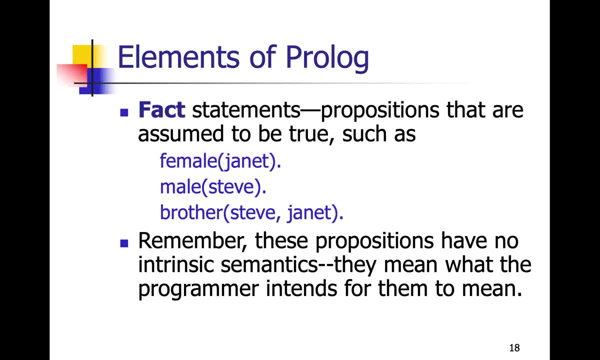 They're propositions that are assumed to be true, such as: female Janet, male Steve, brother, Steve Janet, which is the brother, Janet is the sister, Steve is the brother. Remembering the propositions have no intrinsic semantics, What the programmer intends for them to mean. 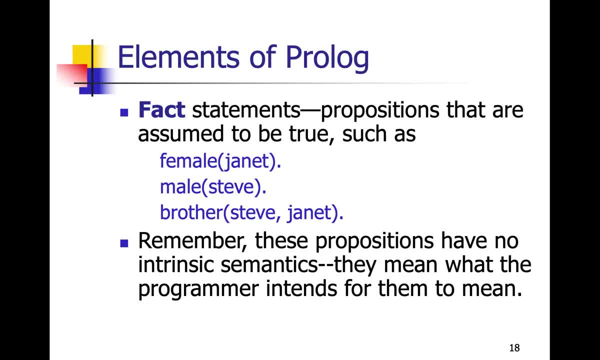 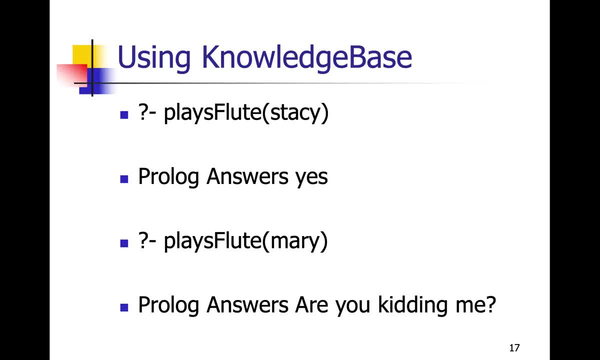 not what they mean in English. So let me give you another more sophisticated example here to sort of tell you how things can be put together So I can say stuff like all short people, like pizza, which I think is probably true, John is short. 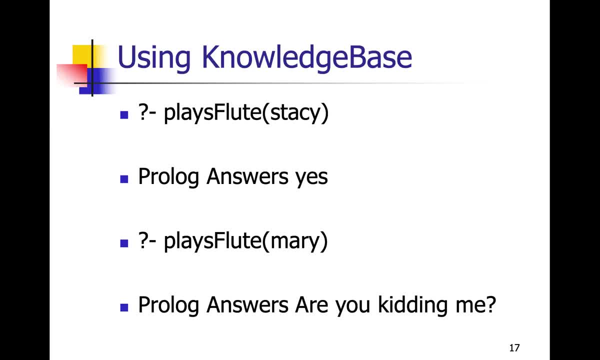 And then you're going to ask Prolog, Does John like pizza? Prolog can come back and say: yes, because John is short and all short people like pizza. Yeah, good. And then you could say: well, Larry is tall. 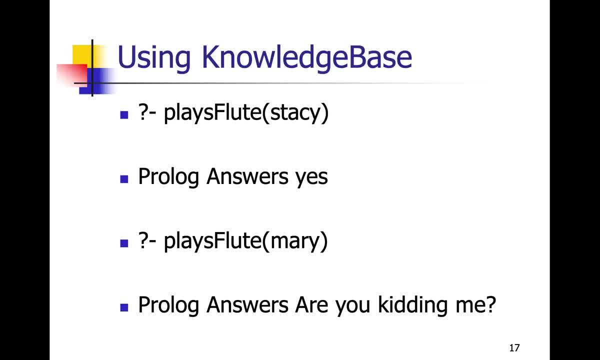 and all tall people like chocolate. Does Larry like pizza? Prolog is going to come back and say no, It's not. going to come back and say no, he doesn't like pizza, He likes chocolate. You actually have to ask it. 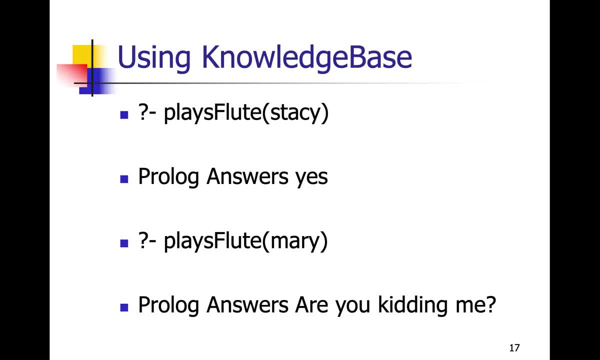 Well then Prolog, does Larry like chocolate? And then Prolog will come back and say: yes, because all tall people like chocolate and Larry is tall. Okay, very simple, Take that concept and complicate it a little bit more with more logic. 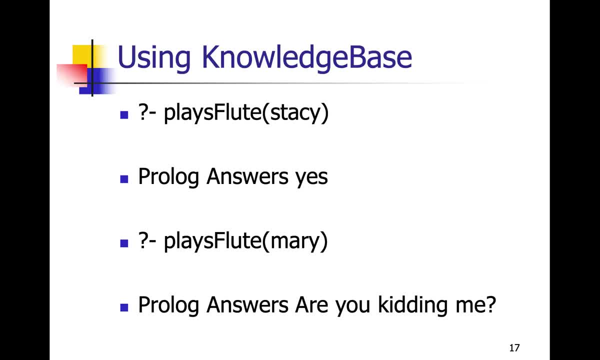 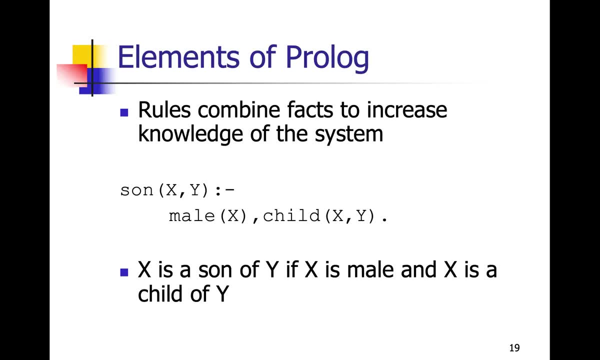 And then you get into mimicking how humans actually think. If you think about it, how much different is that from how humans think? Don't humans memorize a bunch of stuff Like the earth is not round or the earth is round And if I walk to the edge of the earth I'm going to fall off. 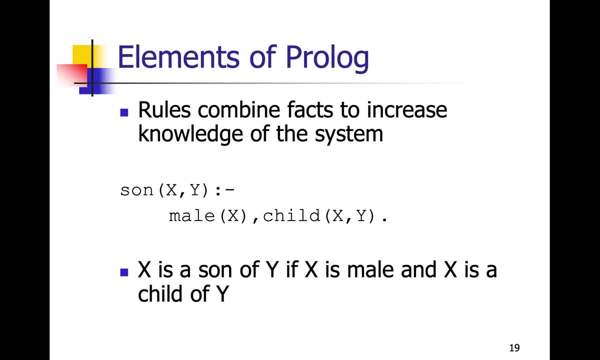 So therefore I should not walk to the edge of the earth because the earth is flat and I'm going to fall off. It's not round. Okay, that's kind of primitive thinking from the beginning of time, But if you think about it, kind of people go. well, it's raining outside. 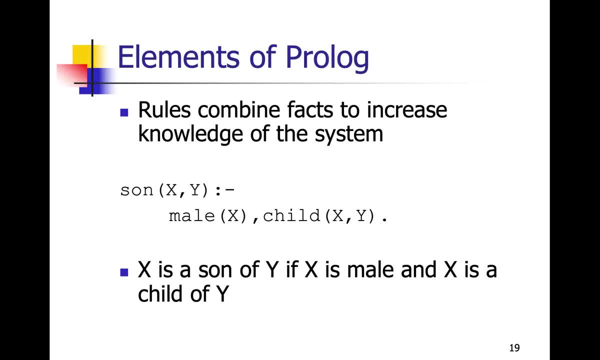 If it's raining outside. it actually started raining, So you have this live update Whether the report Prolog was correct. it's going to rain. So if it's raining outside, then I'm going to bring an umbrella, And if it's not raining, I'm not going to bring an umbrella outside. 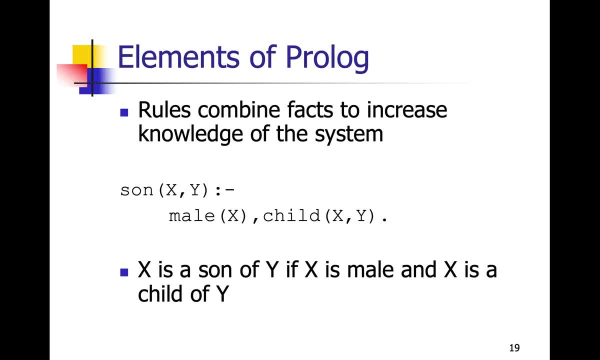 So if I were a human and I was asking myself this question, I look outside and go: oh, it's raining. If I'm going to go outside, I'm probably going to grab that umbrella, Maybe, who knows, or throw on a jacket or something. 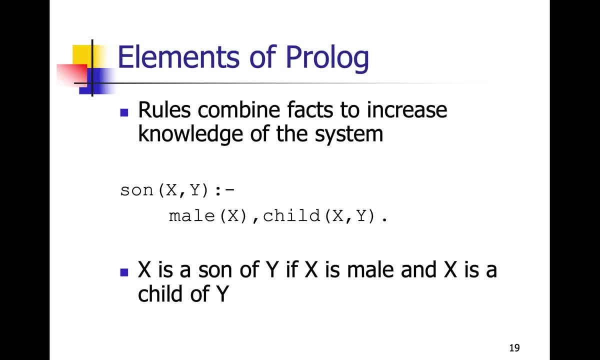 It's the same kind of logic we use as humans, which gives it that AI component, So it's pretty much an AI thing. We have another element of Prolog and this is called the rule, And what you're looking at is a rule. 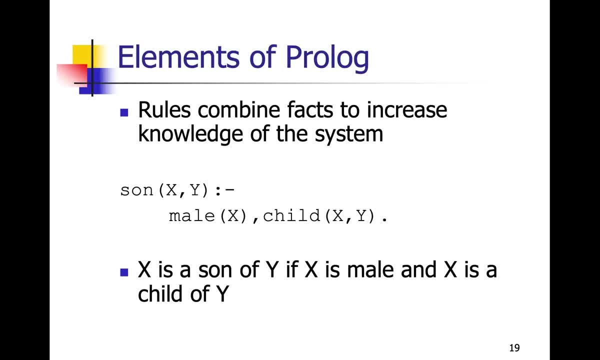 The rule combines the facts to increase the knowledge base of the system. So we have a sun x, y, And then this is actually an arrow, believe it or not, If you imagine this being an arrow here, kind of like if you drew a line between this little dot here and this little dot there. 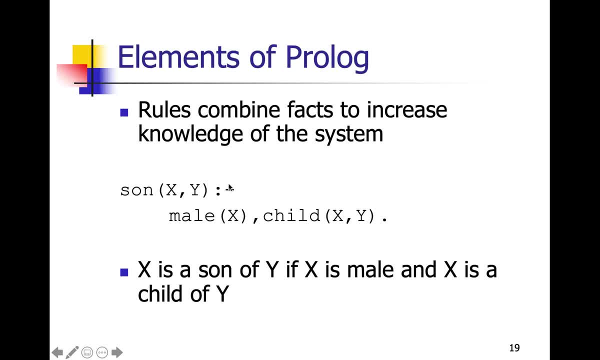 it looks like an arrow, which actually stands for: implies: So x is the sun of y if x is male and x is the child of y. So these are two facts that are separated by a comma, that are put together that imply this: So the sun x, y leads to or infers that number one, that x is a male. 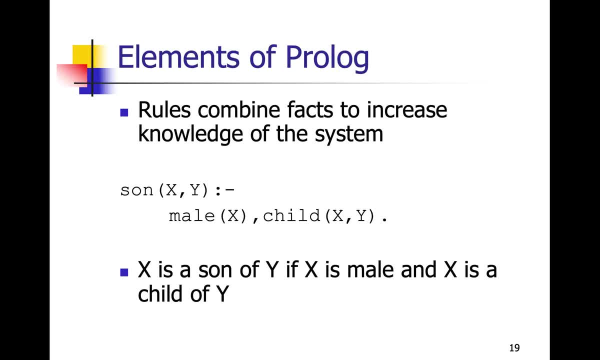 and number two, that x is a child of x- y. That way you're a sun if you're a male child. So read about that a little bit on the website and kind of dwell on that one for a bit and it'll start making sense to you. 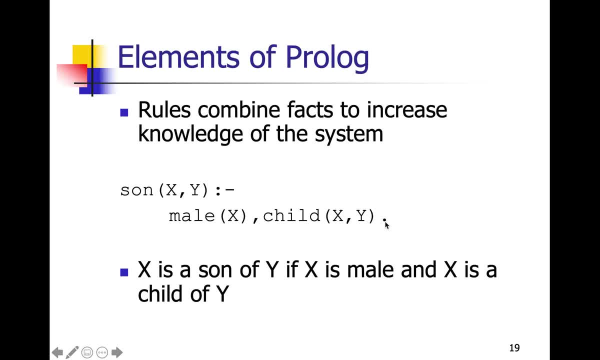 This is Prolog syntax. by the way, There's a dot at the end of the sentence. This can and should be. I don't know. for illustrative purposes it's on two lines, but you could put it on one line. 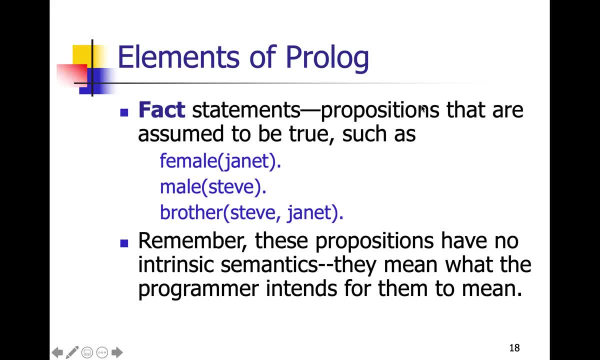 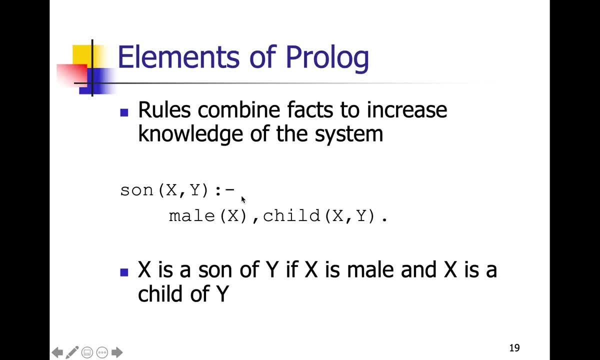 The facts look like this: There's a dot at the end. So the dot says: we're done. That's how you make a fact, That's how you make a rule, And that's all you do. That's the syntax of the language. 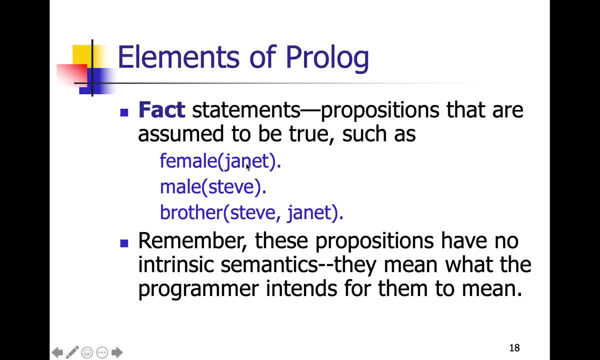 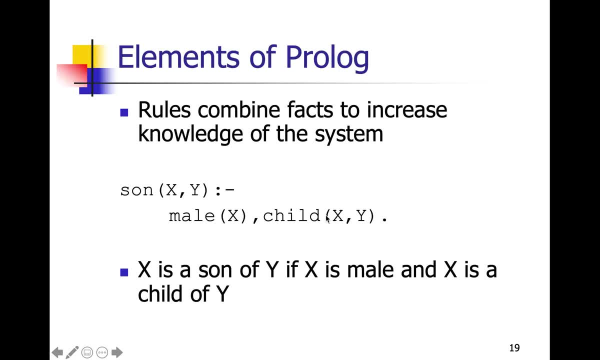 So if you were going to make a function, well, the function looks like this And there's stuff combined in the function to make it like concatenate two lists together, And I'll show you that momentarily. But So here's the elements of a Prolog database. 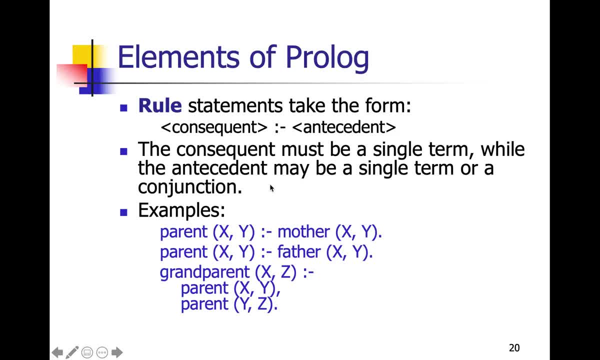 Okay, so remember that question number one, where you're going to define sibling and sister and brother. So this is slide number 20, and it's pretty much the answer to the question. So here we have an example, and this is going to show us the resolution process as well. 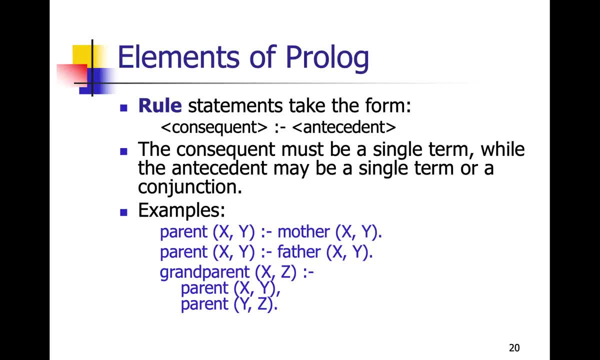 So we have a parent of x? y that is a mother of x? y. We also have a parent of x? y that has- that's, a father. So we have two parents: We have a mother-parent and we have a father-parent. 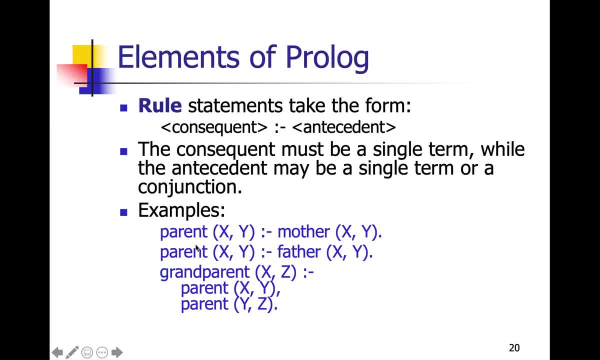 And what I'm talking about are these two lines right here And you're like: well, aren't we defining this twice? No, we're not. So don't think about this semantically as a definition. This is not a variable. 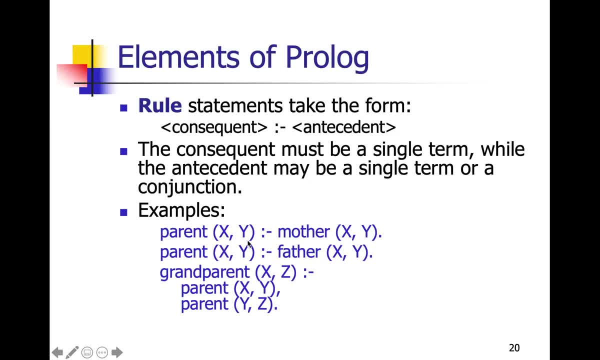 This is not a fact, that This is a fact. Well, actually, this is a rule, These are facts. This is combined into a rule And there's no, There's no. There's nothing wrong with repeating it, Because a parent is a mother and a parent is a father. 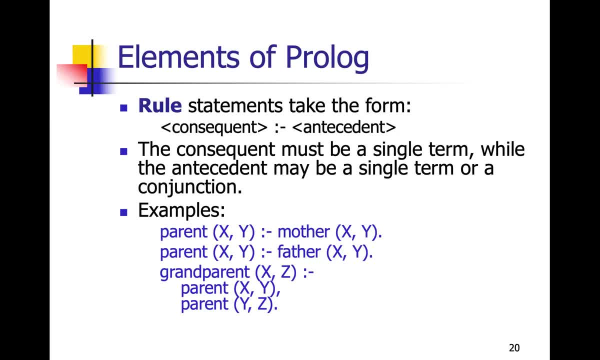 The traditional family has a mother and has a father, And then the grandparents. Well, each one of the parents has a grandparent And there's two grandparents. Well, originally, you're lucky if you have all of them alive still, But the grandparents should have. 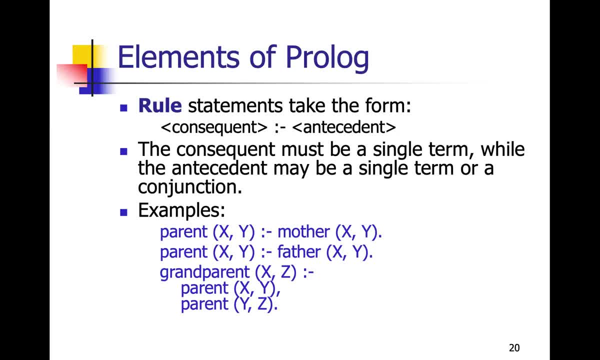 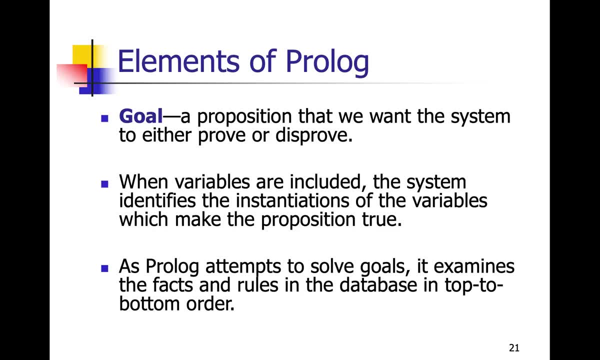 Each one of your grandparents should have a mother and a father as well, which are grandparent mothers and fathers. So the goal to the system is either going to be proved or disproved, And when the variables are included, the system identifies the instantiations. 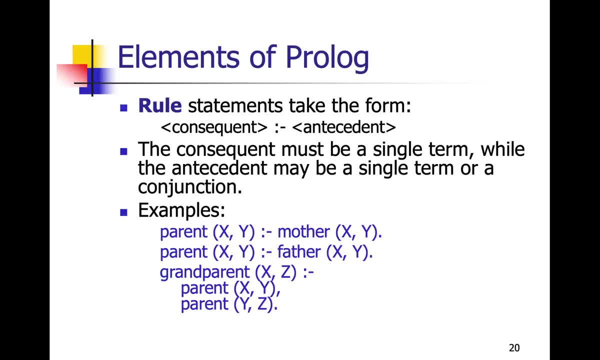 and makes them true or false. So this X- Y are placeholders for people's names, So you can create a database of your family And then you can ask: well, is Larry the brother of so-and-so or the son of so-and-so? 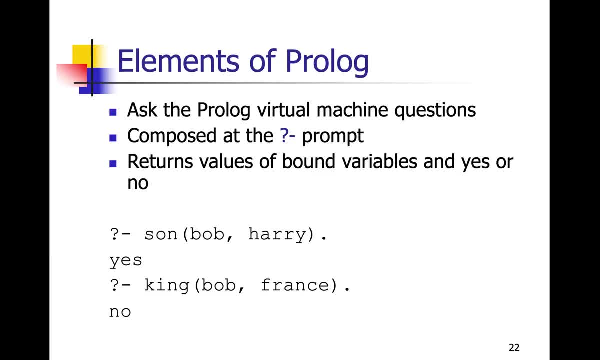 You ask Prologue the virtual machine questions. Son Bob Harry: yes. King Bob of France: no. So it returns the bounded variables with yes or no answers. Prologue only answers with yes or no, or true or false, depending upon the Prologue system that you have installed. 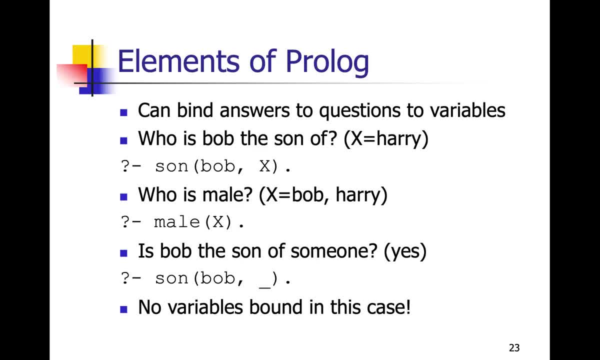 So you combine answers to questions, to variables: Who is Bob? the son of X is equal to Harry. And then it comes back and says You would say son Bob X. Who is male? X is equal to Bob and Harry. Well then, male X. 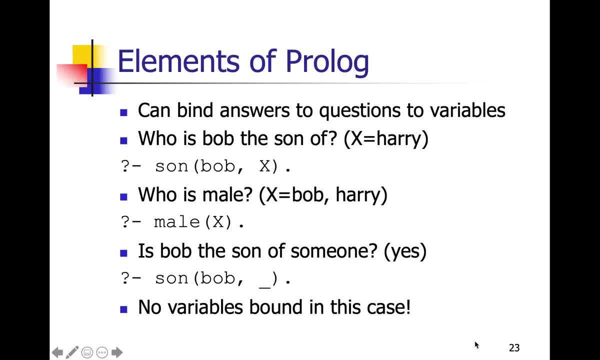 Is Bob the son of somebody? And then you have this little empty placeholder that means we don't know, And then no variable in this particular case is given. We're just trying to figure out: is he the son of somebody? And then it will come back true or false. 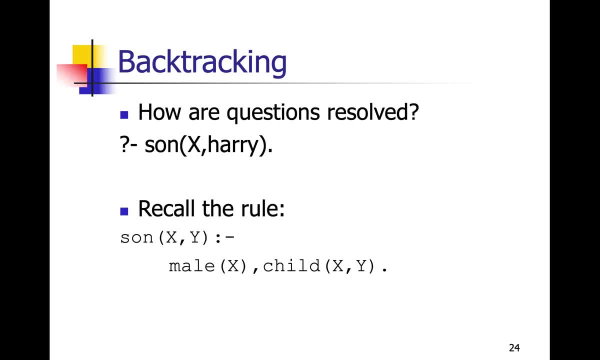 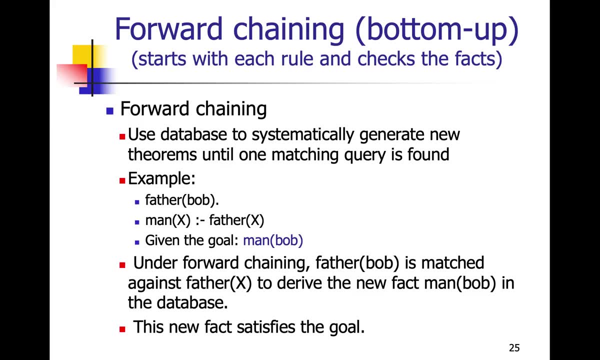 So backtracking, How are the questions resolved? Well, we start with recall the rule And then go to the facts, And then forward chaining. I've already talked about backward and forward chaining, But forward chaining starts with the rules And then it applies it to the facts to see if it works. 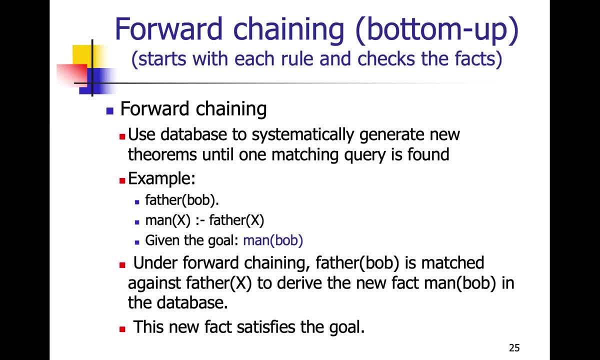 So under forward chaining father Bob is matched against father X to derive the new fact that man Bob is in the database And the new fact satisfies the goal. so it stops. You don't have to really worry about the forward versus the backward chaining. 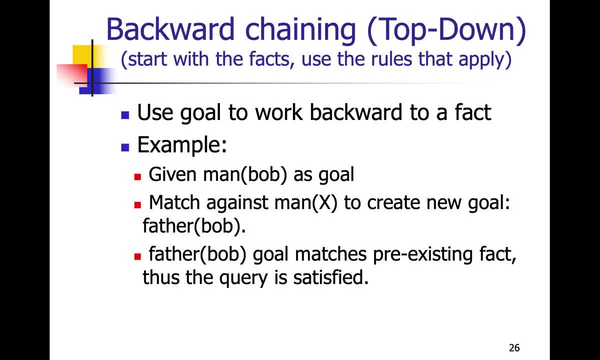 It's just explaining how the system actually resolves the data. So in the backward example in this particular slide, you use the goal to work backwards to a fact. So in the backwards you start with the conclusion. You say it's going to rain or man. 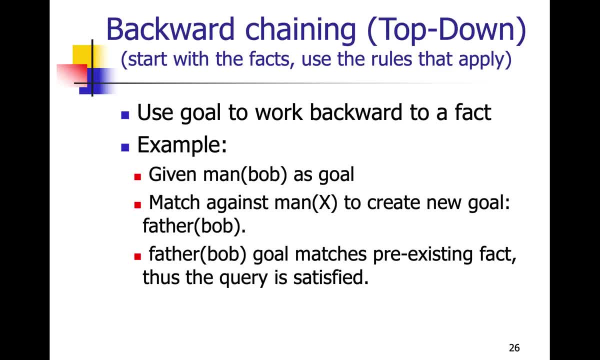 You're giving man Bob And you're just going to say: is Bob a man, Yes or no? Match against the man X to create the new goal: Father Bob, Father Bob goal matches- preexisting fact. Thus the query is satisfied. 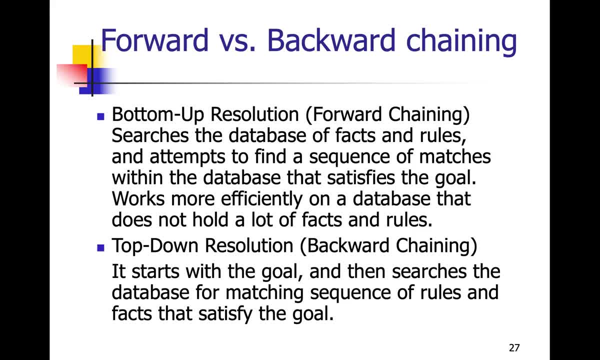 And yes, we can go back and say: yes, it is So. are you going to solve by following the question forward to an answer, Or are you going to start with a conclusion and go backwards? So I already actually kind of talked about this. 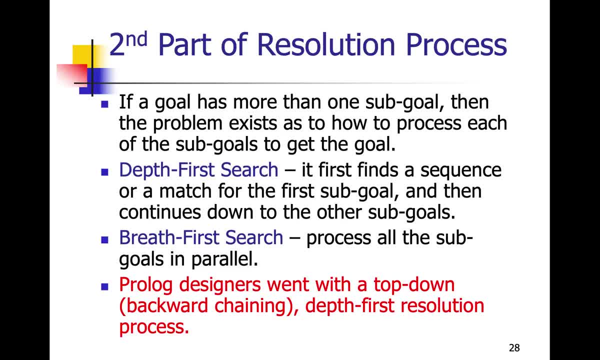 So I'm going to pass through it again. The second part of the resolution process does what's called a depth first or a breadth first search. Go back to data structures and algorithms and take a look at the depth first versus the breadth first. These are just the resolution processes. 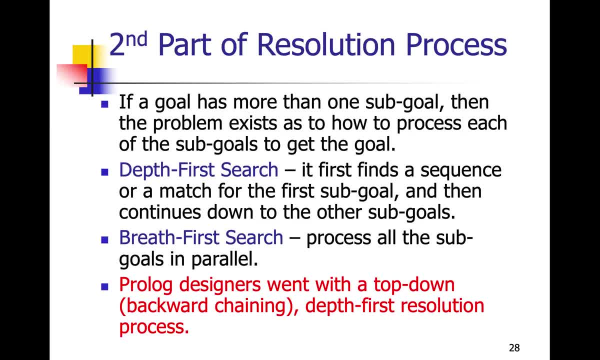 Prolog designers went with a top-down, which is backward chaining depth, first resolution process. That little bullet point in red here is telling you what the default is. You're not stuck with that. You can actually change that, But I wouldn't do it for this assignment. 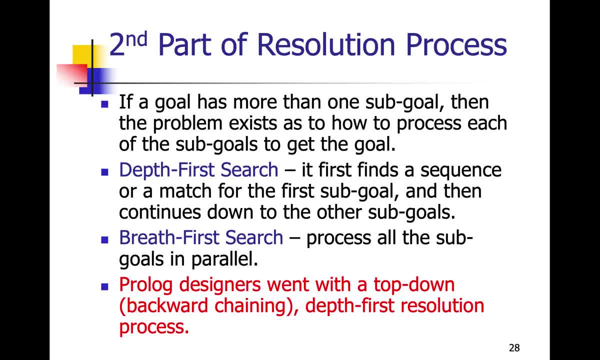 If you get into Prolog for artificial intelligence in the future, you might consider changing around the resolution process depending upon how your application is designed. So, depth first, Depth first starts first finds a sequence or a match of the first subset goal and then continues down the other subgoals until it finds it. 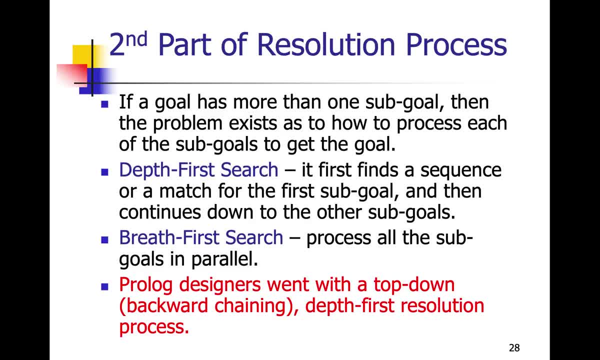 Breadth first processes all levels in parallel. It's like we're going to start at the top of the tree and we're going to go through each level, down to each level, down to each level. That's the breadth first versus the depth first. 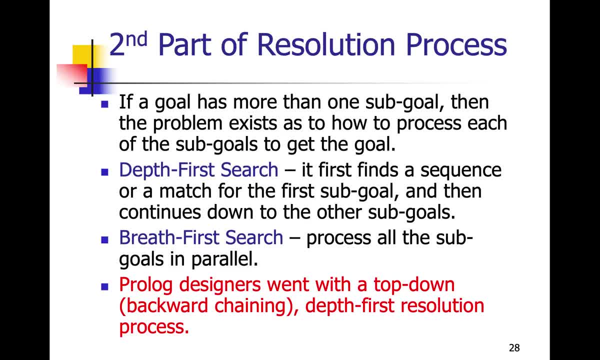 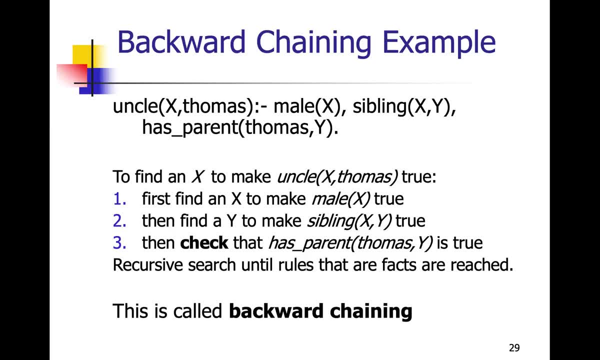 Go down until we can't go anymore. We hit a leaf node and then we go back up and we try another branch. So that's the search process. So we have the uncle X, Thomas, with male X, sibling X, Y, as parent, Thomas Y. 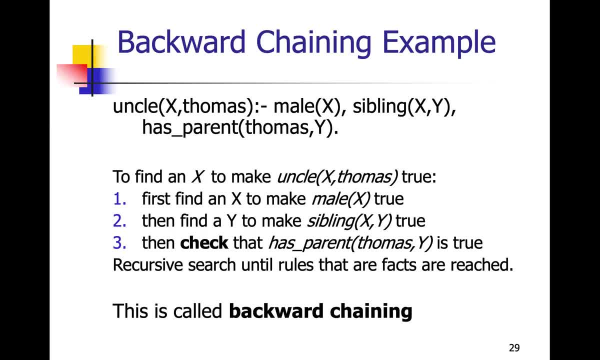 And if we were to use backward chaining here, we would find an X to make uncle X Thomas true First. find an X to make the male X true, Then find a Y to make the sibling true, the XY sibling true, Then check to see if it has parent. 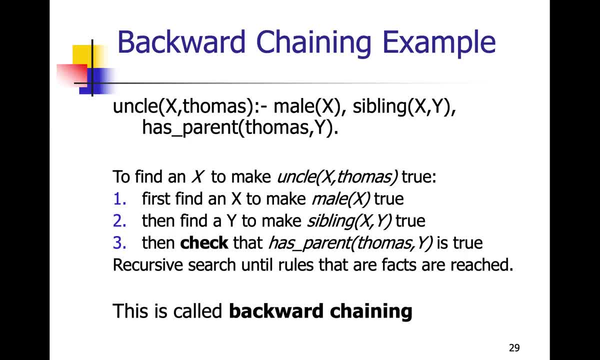 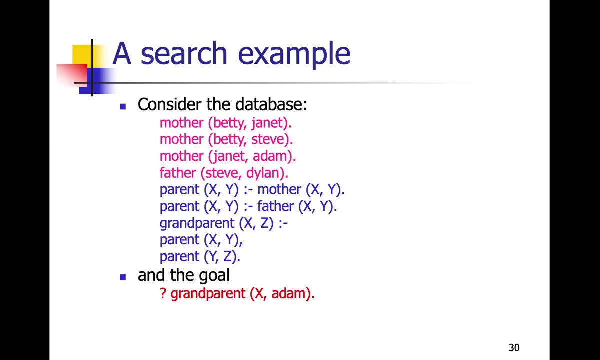 If it is, then it's true. This is a recursive search until all the rules and facts are reached. Until the facts are reached, I should say So it's called backward chaining, All right, So here's an example that's going to help you with the assignment. question number one: 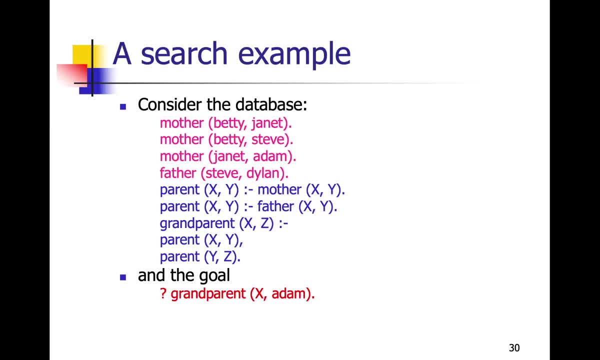 Consider the database. So now, instead, we're going to populate it. So we have mother Betty Janet, mother Betty Steve, mother Janet Adam and father Steve Dillon, And then we have the rules. We have a parent which is a mother and father. 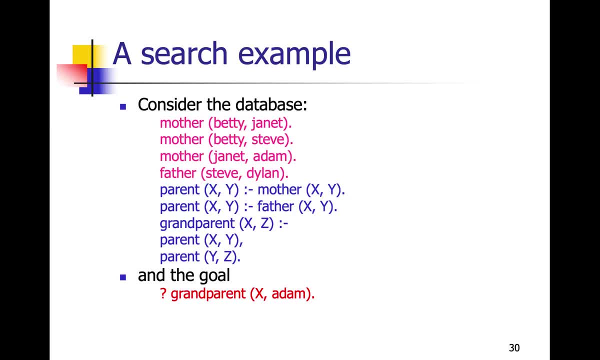 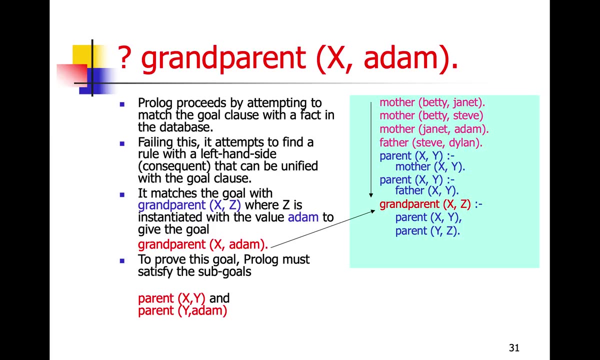 We have a grandparent that has a parent on both sides- mother and father- And the goal is grandparent X comma Adam. So is the grandparent of X Adam? Hmm, So if we go through the resolution process and you can download this slide and go through it a little bit slower if you'd like, 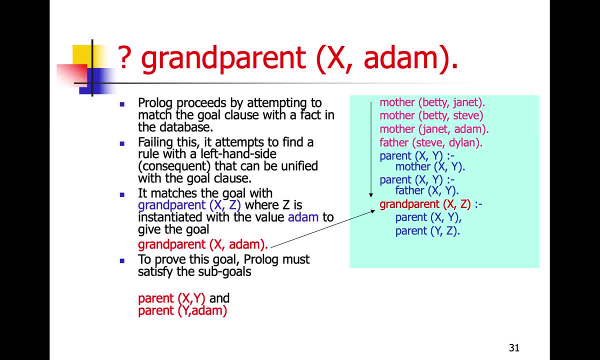 we need to proceed by attempting to match, And so in this particular case, we're going to start with, because the question in this particular case is grandparent X Adam. So we're going to start with grandparent X Adam here To prove this goal. we must satisfy the subgoals. 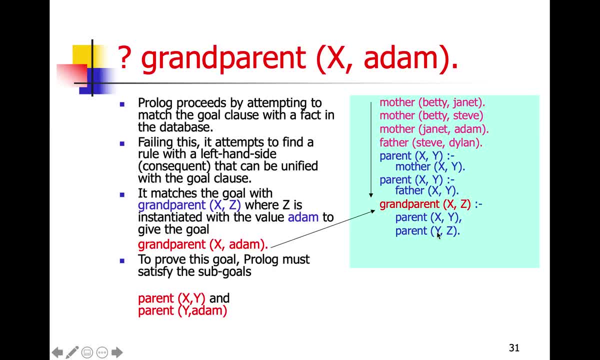 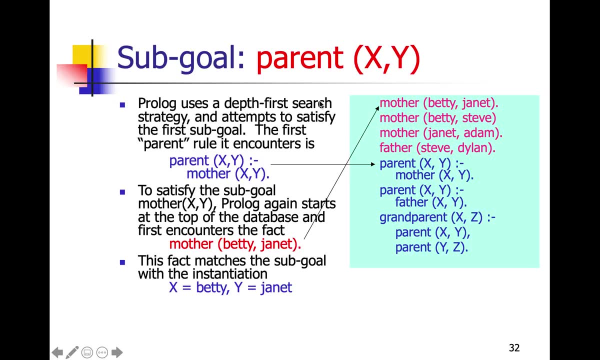 And the two subgoals are parent XY and parent YZ, And so we're going to put the Adam in for Z And so we have parent Y Adam. So we can use a depth first search in this particular example and attempt to satisfy the first goal. 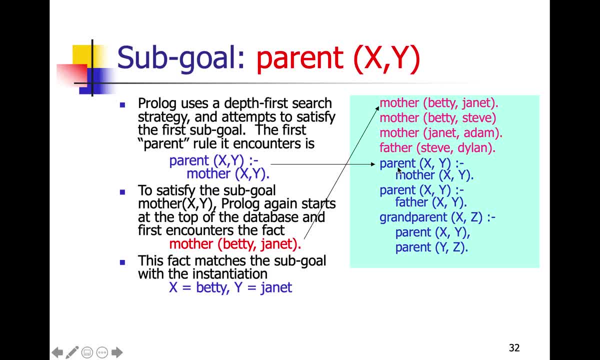 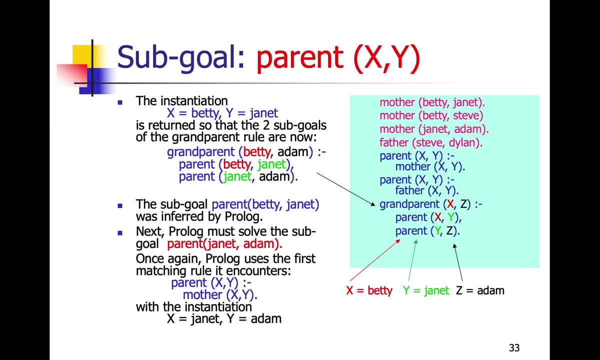 So we're looking for parent XY here And then to satisfy it. well, we're going to find it up here. We have mother Betty Janet, And so the fact matches the subgoal with the instantiation of X equal to Betty and Y is equal to Janet. 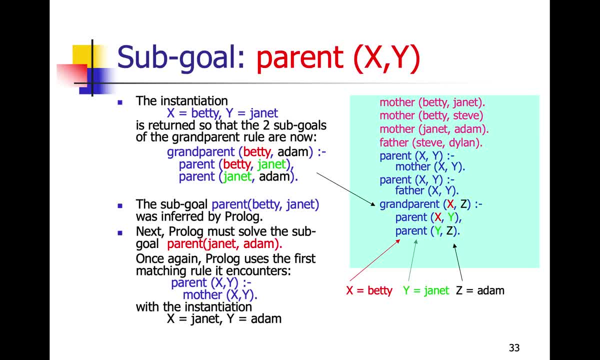 And then we're going to instantiate it. So X is now Betty and Y is now Janet. We're going to substitute those guys in to the grandparent and see if it's true. And so the Z is Adam And we're trying to find we have the Y is Janet and X is Betty. 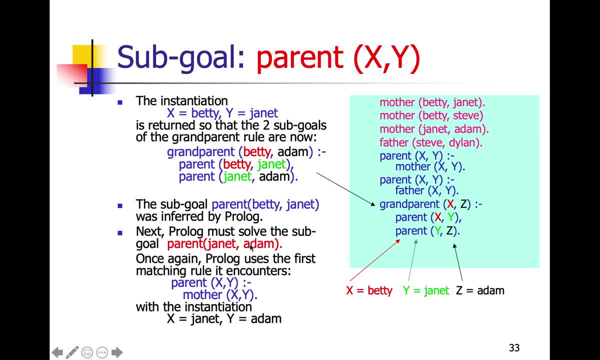 And so next prologue must solve the subgoal parent Janet, Adam. Can it do that? Once again? prologue uses the first matching rule it comes into Instantiates, the X with Janet and the Y with Adam, to see if that's true. 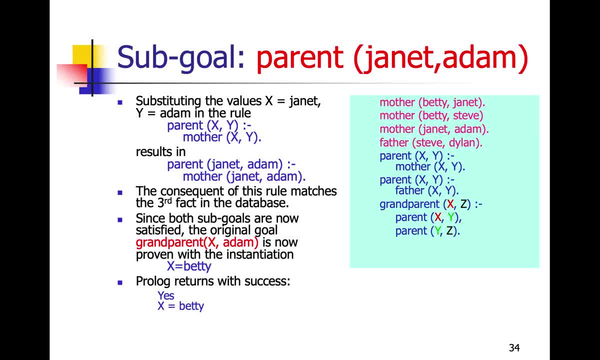 Substituting those values in it results with parent Janet Adam. mother Janet Adam. So the three facts in the database are applied And now we have to satisfy the original goal. Can we satisfy the original goal that grandparent X was Adam? 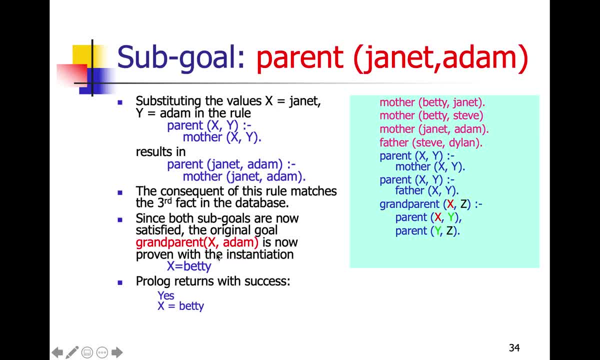 So it's now proven with the instantiation of Betty because it found a combination with Betty. So prologue returns with success. It will say yes because X is equal to Betty. So the answer is yes, Proven that Janet comma Adam is true. 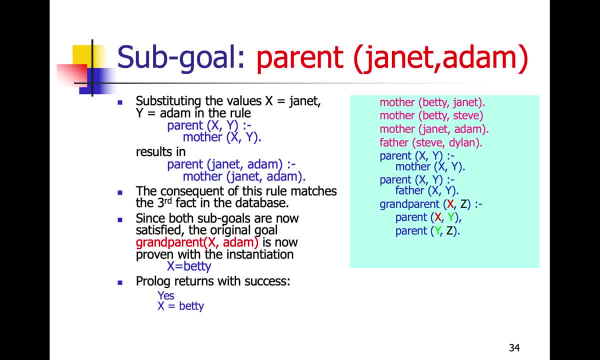 Um, So we found the match. essentially, You don't have to do any of this. You don't have to program any of this. This is done for you. This is an example of how prologue works. Prologue is doing this for you. 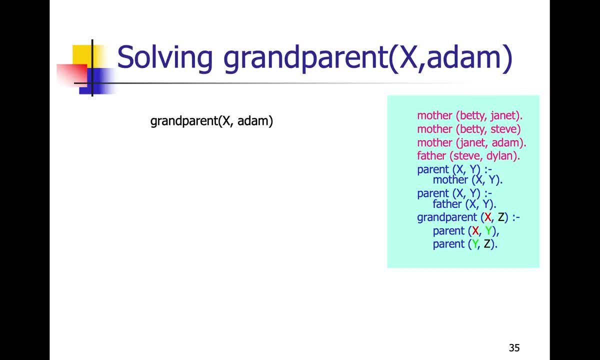 So if we solve this graphically- and I'm just going to kind of step through this here- It's the same problem we just looked at a few minutes ago- And stepping through it so you can sort of see how the resolution process works- 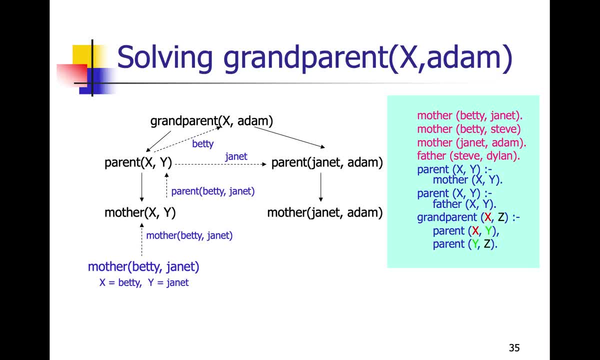 This is demonstrating the depth first approach, Knowing that it went down the side of the tree first. Now it's going down this side of the tree All the way to the end until it resolves it, And so we have the resolution process demonstrated with a depth first approach. 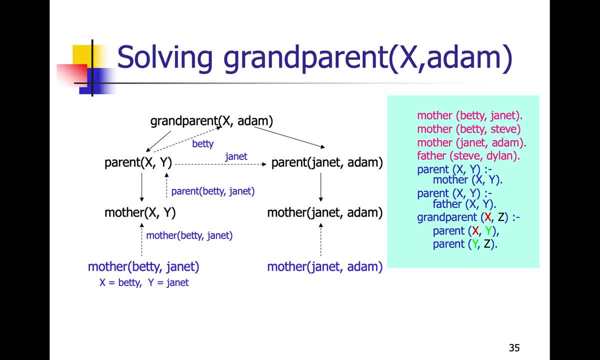 Which is the default used in prologue. Alright, Believe it or not, that's everything you need to know about facts and rules in prologue. You're going to need to probably study this a little bit more before you do the assignment, Or maybe you can just jump into the assignment. 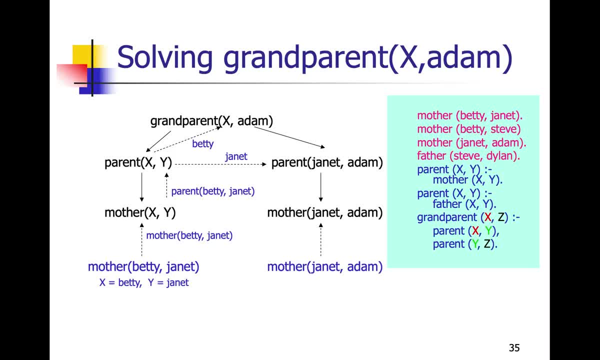 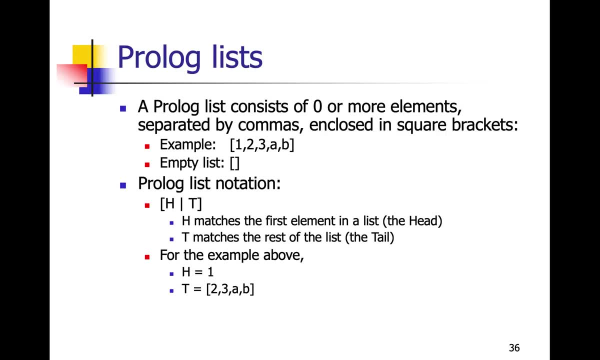 Take a look at some of the examples And lots of this stuff will start making more sense to you. So now let's talk about the prologue list. You're going to have a couple questions in the assignment that's going to have you work with a list. 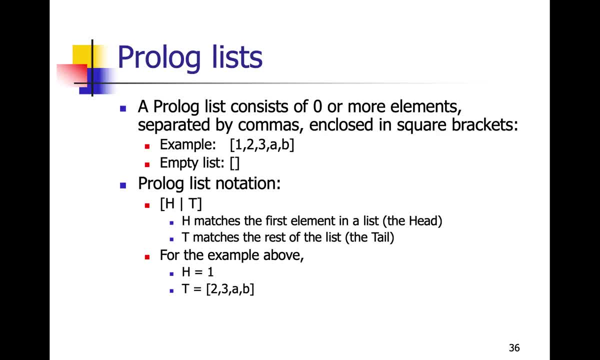 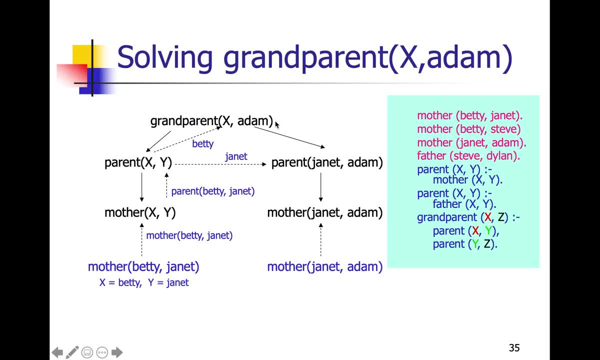 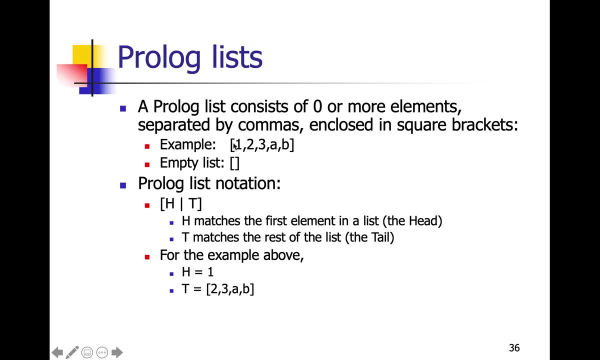 So it consists of zero more elements separated by commas, Enclosed in square brackets. So, knowing that the syntax over here had rounded parentheses, Prologue lists have brackets. The notation is using brackets. So if we're using brackets, we know we're looking at a list. 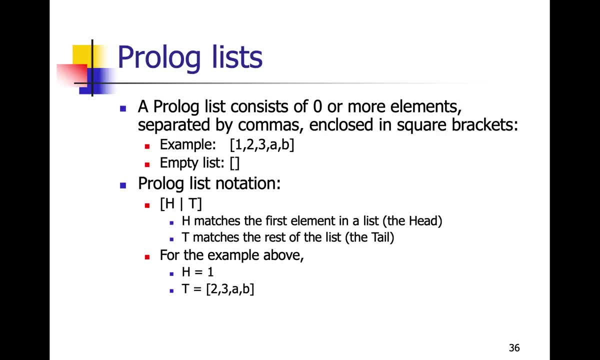 And the prologue lists are linked lists, So you don't have to invent the linked list concept. that's already given to you, Not like C++, It's given to you already. The empty list is just an empty list here. This is what the empty list looks like. 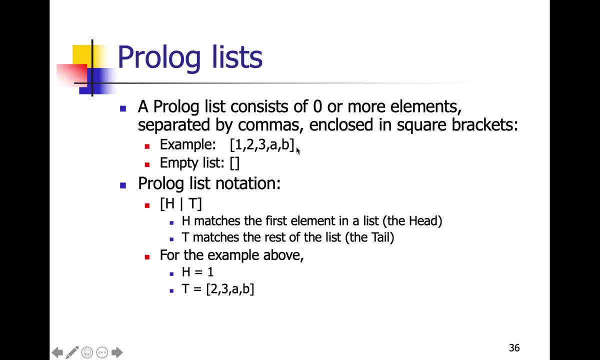 Here's a list that's populated, that's not empty, And it contains numbers and characters. You can put words in there, You can put a list in there, You can put anything you want in there, So you can mix and match the data types. 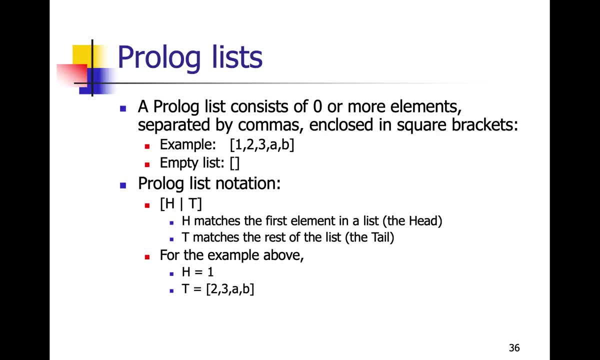 Because there's no such thing as data types in this language. Instead, there's just elements. All the elements are treated equally. You can also put placeholders in there, You can put facts in there. You can put anything you want in there. 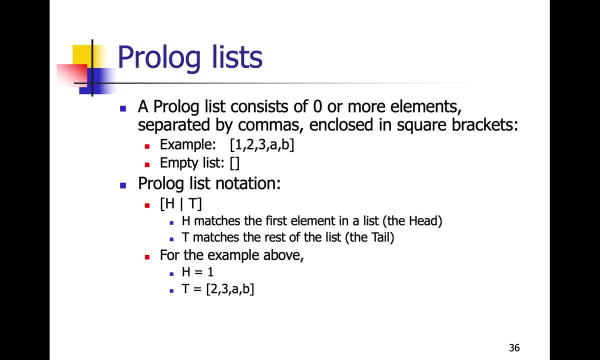 The prologue list notation has a head and a tail, So this is where the head and this is where the tail comes into place. For example, the head might be 1.. The tail might be 2,, 3,, A and B. 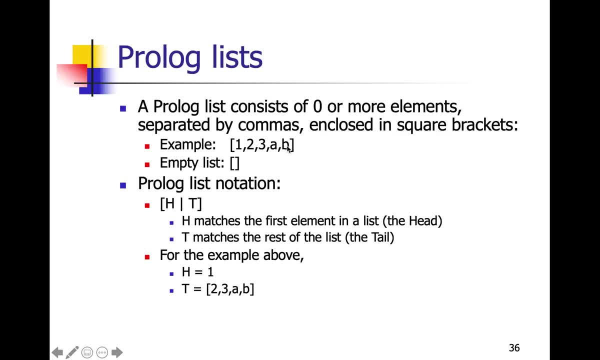 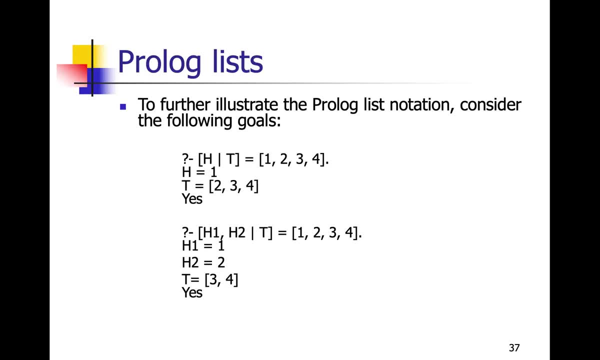 Here. this is the head, This is the tail. So the head is the first element. Go back to your concepts of linked lists And this will make a lot of sense, hopefully. To further illustrate, here we have the list notation, considering the following goals: 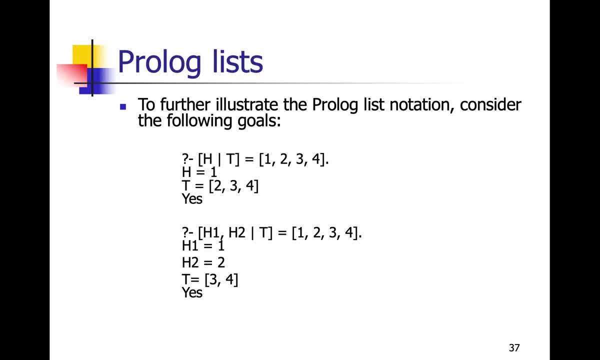 With the head, tail is equal to 1,, 2,, 3,, 4.. Head is 1., Tail is 2,, 3,, 4.. And prologue will come back and say, yep, that's what we got here. 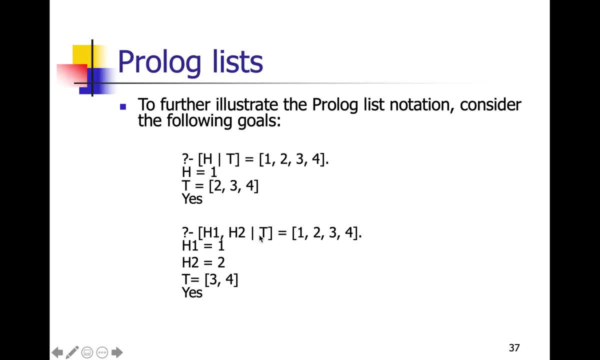 Or we could have head 1,, head 2, and the tail. Well then, that would be: head 1 would be 1, 2, and then the tail, So we can have as many heads as we want. We only have one tail. 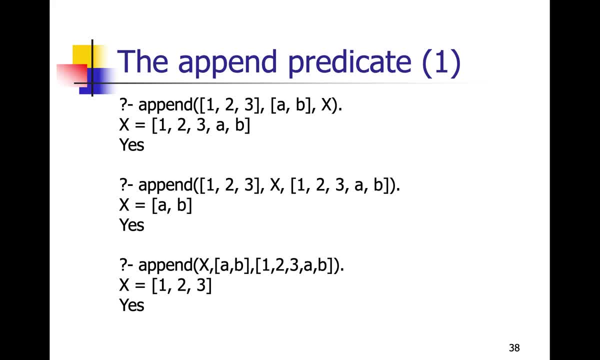 But we can have as many heads or as many components as we want in the list. OK, Remember, you're going to write a list that takes two lists and puts them together. Well, not to totally give it away, but all the answers to the homework assignment are in this lecture. 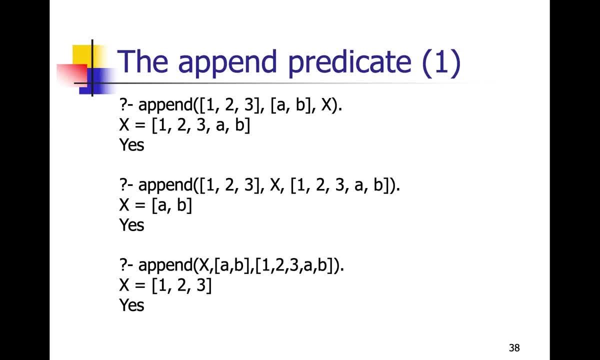 Yeah, I guess I totally spoiler alert. I have given you well too much information, Because this lecture is going to cover everything. But the idea is I want you to take a look at the lecture And I want to take you to look at the assignment. 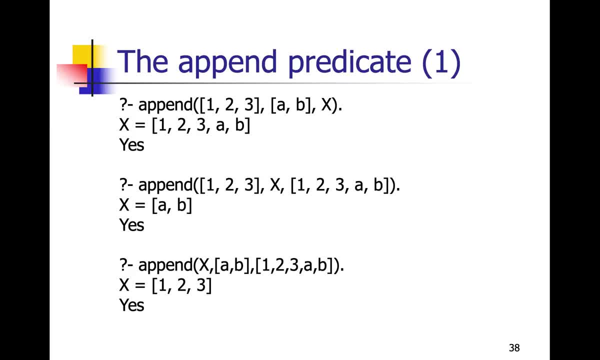 See if you can put the pieces together yourself, to see if you can figure out how to do this. But it's all here. There's nothing else you have to read. So here's append. What does append do? Append is a built-in function. 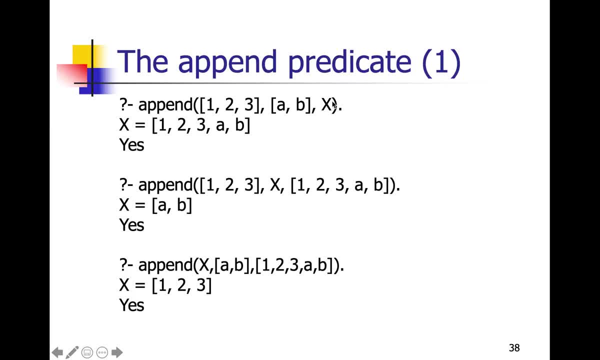 Append. And so we have this function here, functor, with the rounded brackets, And inside we have two lists. We have the square brackets that say 1,, 2, 3.. And then we have ab, And if we append this together we have 1,, 2,, 3, ab. 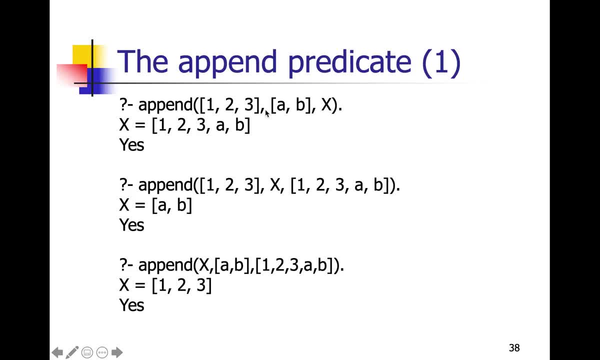 x is what we're going to append it to, So this is not okay. so don't think of these as parameters to a function. This is not a function call. This is a functor or a fact that says a list. x is 1,, 2,, 3, and ab put together. 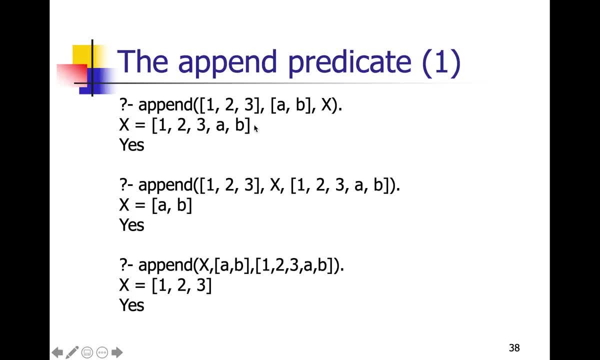 And so if we actually asked what x was, we would say: well then it's 1,, 2,, 3, and ab. So here's two items that are put together for x. And then we have this guy going on here where it says: append 1,, 2,, 3, and x. 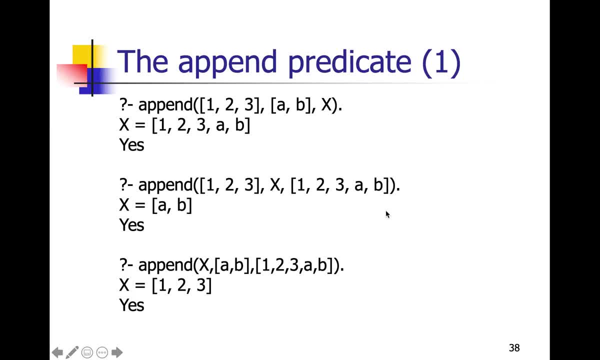 Well, x is 1, 2, 3, ab from here, And then we get 1, 2, 3, ab. So then x is really ab, because it's the difference between 1, 2, 3, and 1, 2, 3, ab. 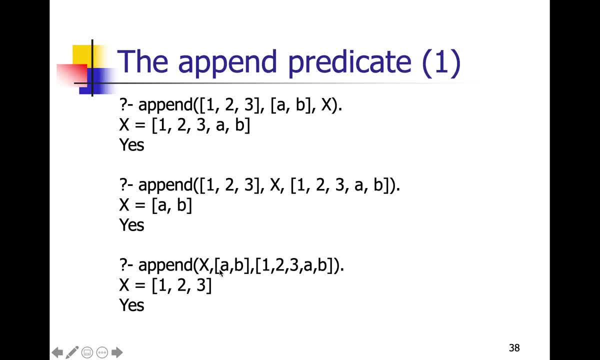 Yeah, stare at that one for a while And then stare at this next one here where we have x. These are just different combinations of the append x, which is the 1,, 2,, 3, ab, and then ab. now x is 1,, 2, 3,, which is the difference. 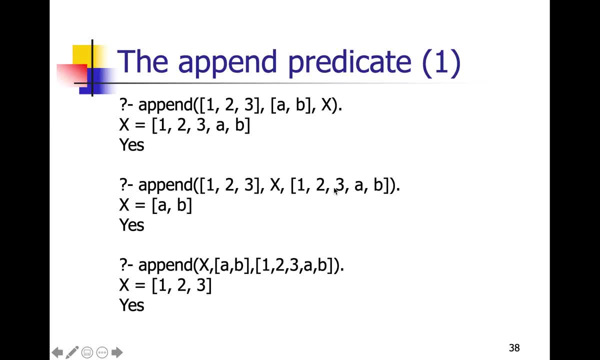 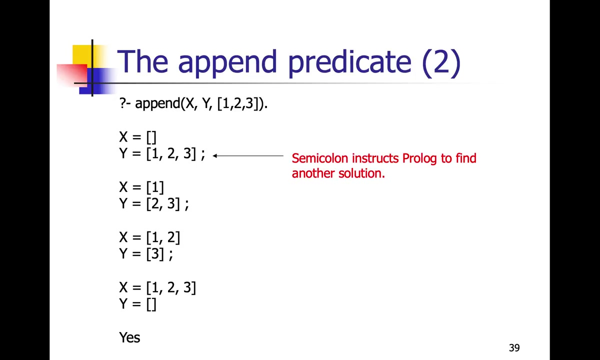 So we took out the ab. Here we combine the ab together. So this is the difference. So these are different combinations. Go online, Take a look at the append And see how the append works. There's a really good documentation on the SWI prologue site as well as on swish the prologue site. 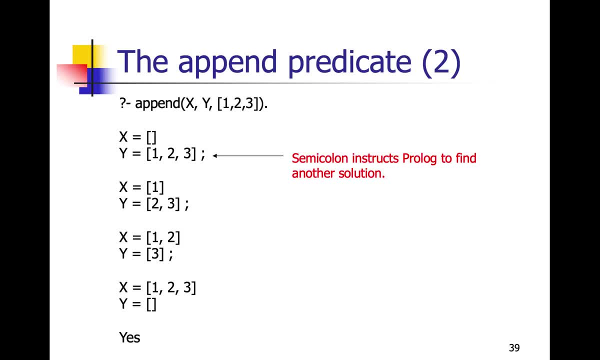 So remember before I said you could find multiple proofs. A proof is to ask prologue a question and have it come back and give you an answer. So here's an example of how the proof works. You put in a semicolon. If you put in a semicolon, 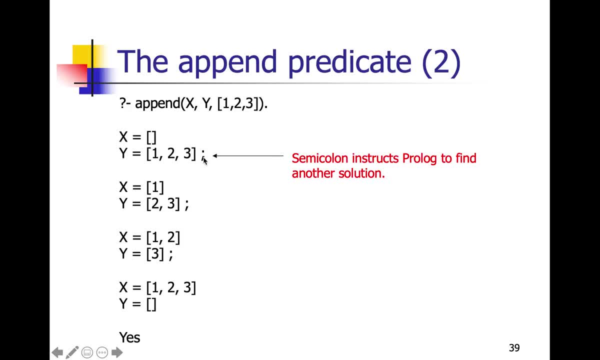 here's the semicolon. instructs prologue to find another solution. Go ahead and just find another solution. So if prologue was trying to find x, y with 1,, 2, 3, the list: 1,, 2, 3,. 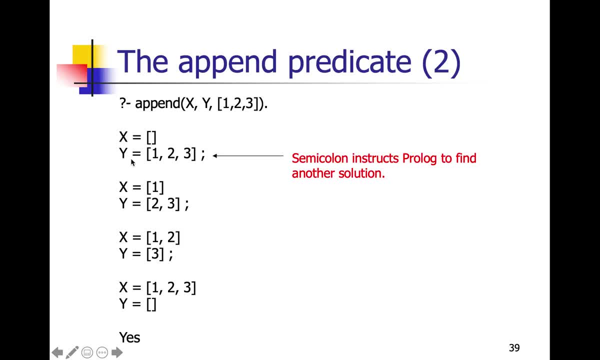 and if it came back and said, well, x is empty y, let's say, make that one, put a semicolon in there. then it continues: x is 1,, y is 2, 3,, x is 1,, 2,, y is 3, x is 1,, 2,, 3.. 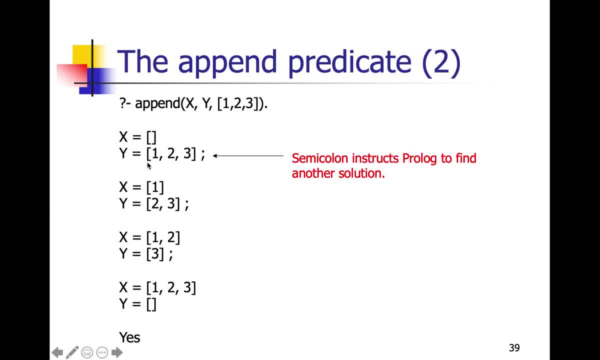 This continues to resolve it by substituting in character by character or list item by list item, And so the semicolon at the end of the line says continue. Continue the resolution process to find the associated fact that matches and see if we can resolve this. 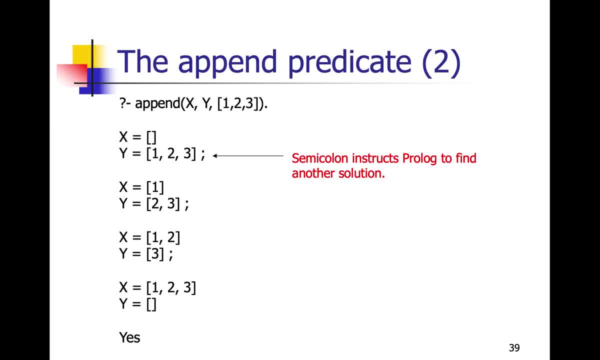 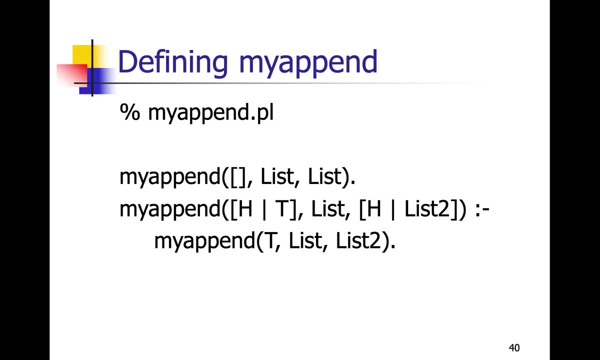 And so then we can figure out and say, yes, x is 1,, 2,, 3,, y is empty. So Here is another defining a function. This is called my append. My append takes an empty list and adds two lists together. 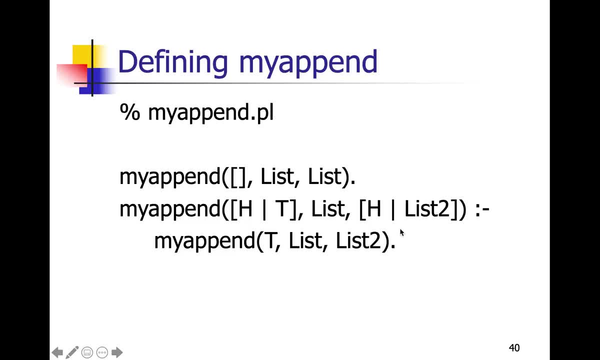 So you know, just in case I haven't given you enough of the answers already, here's how you would write a function. So this is how you would write a function or a functor to define how to combine two lists together. My append takes one list and appends another list to it. 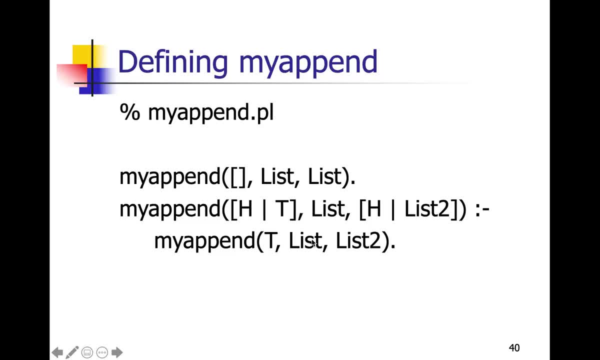 And so My append has a head and a tail. The head is the list, The tail is the other list, And so my append takes and takes the tail and has it equal to the list plus the second list, The first list and the second list. 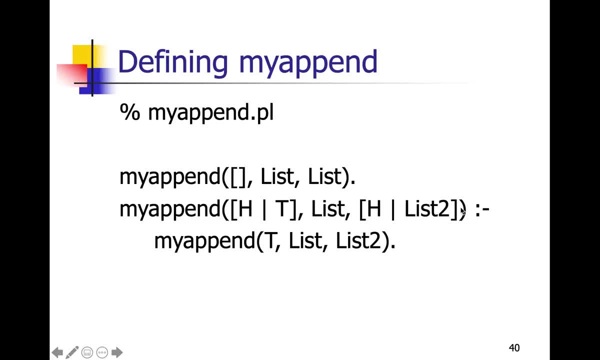 I guess we could have called it list one and list two, but it's just list and list two, So that actually is how you would append two lists together One to the other. And so if you wrote this, this, this rule, it really is a rule with a fact. 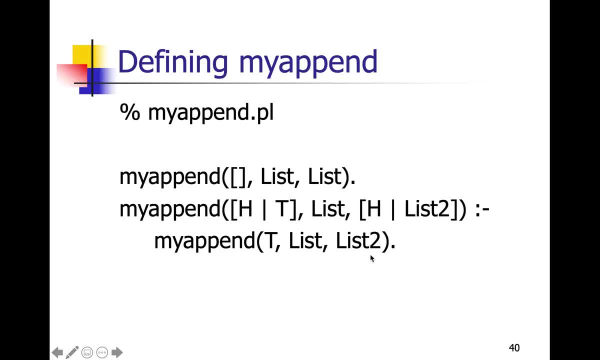 There's a fact. There's a fact And then there's a rule in here. So there's the fact, There's the rule And you put it in a file. You can put it in a file and call it my append dot. PL. 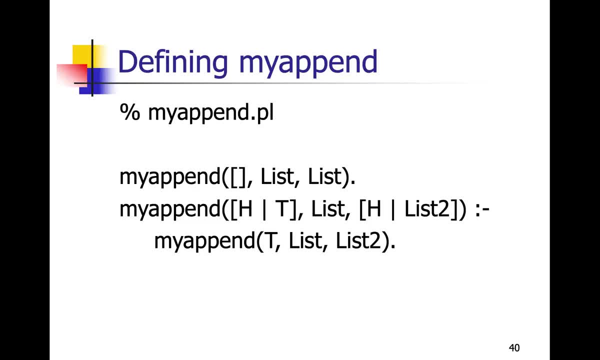 All prolog files have PL for prolog as the file extension And then you could just run the prolog file or import it into the prolog session, load it up and then you could run it. So how would you load it up? 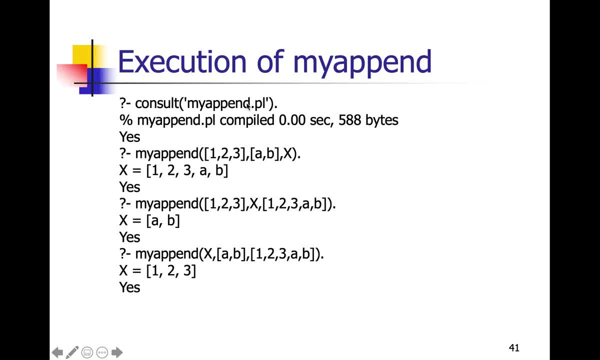 You'd use the word consult- Consult this When you consulted this. it's kind of like an import or include. Consult brings the file in, so now we can run the function. And then we just run the function And guess what. 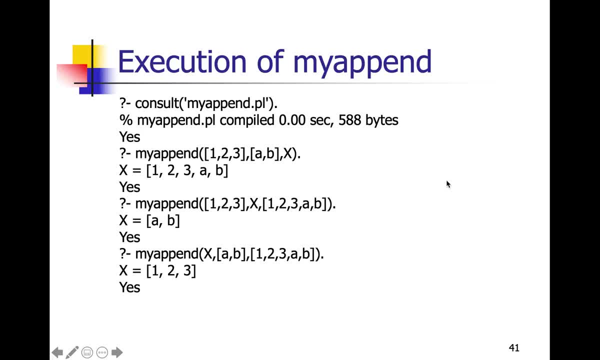 Here's the function And this is how the function works. So I'm going to let you dwell on that, because I've already given too much of the assignment away and I want there to be some element of learning going on with this. So study this a little bit and you'll see how the process resolves. 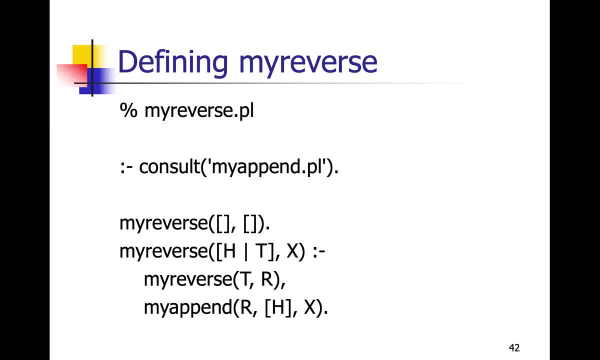 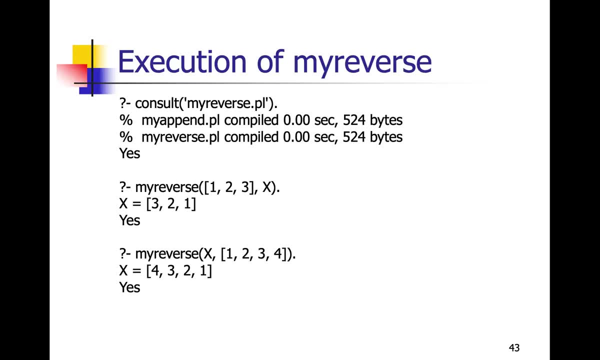 Here's my reverse. You might imagine it reversal-less. It takes and puts it in the opposite order, And so you can consult it and then take a list- one, two, three- and then return it as x. Excuse me. 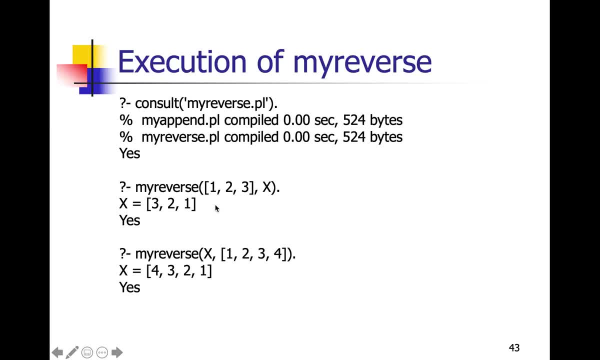 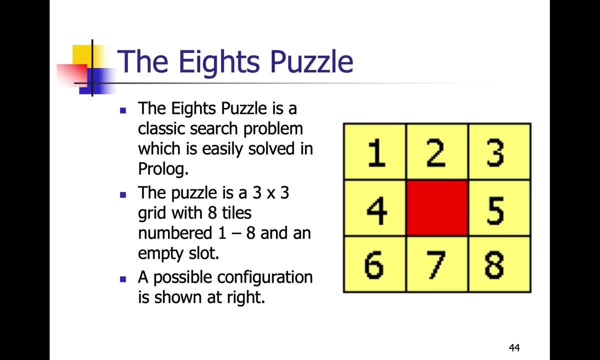 And then we're going to have: x is equal to three, two, one. So here's prolog, solving the eights puzzle. And so the eights puzzle is a game. These are like little squares that you'd move around, And this happens to have the blanks. 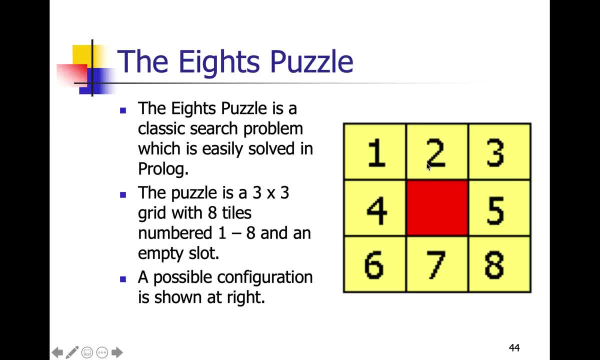 And there's one blank square because you need space in order to move the squares around. So you have a three-by-three grid with eight tiles, numbered one through eight, and an empty slot in the middle, And this is a possible configuration or a solution to the eights puzzle. 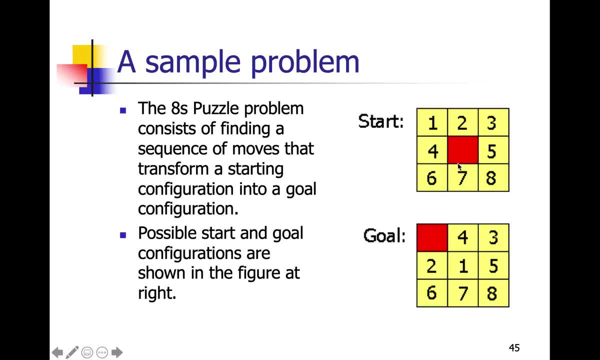 And so you can have a start. Let's say, maybe this was the start And the goal is to put it into this format, Although you probably would want to do the goal as this and start with this and the goal with that. But in any way, you can do it any way you want. 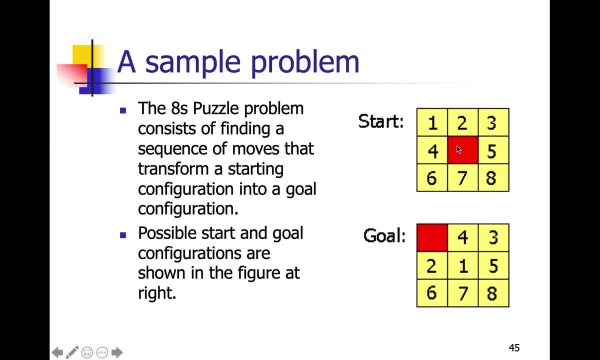 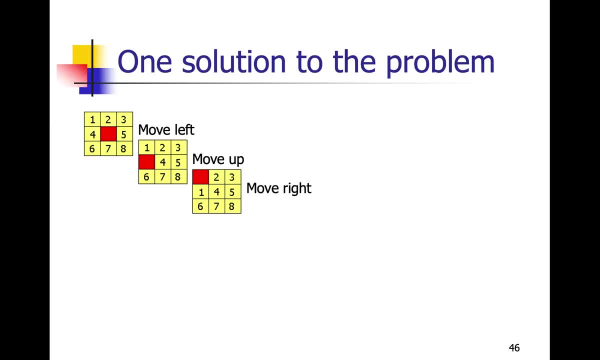 And so you can have a possible start and a goal configuration as shown here, And then you can come up with a solution to it by moving things around. And if you watch the flow of this, you'll see how you could move the spaces into the empty to move everything around. 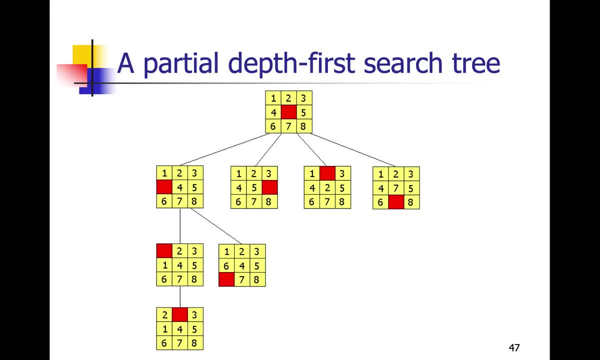 until you've reached the goal state, And so you have a partial depth first search tree. This is what the search tree would look like to get from the start state to the goal state, moving the pieces around, And you can put this in a Prolog program and have Prolog solve it for you. 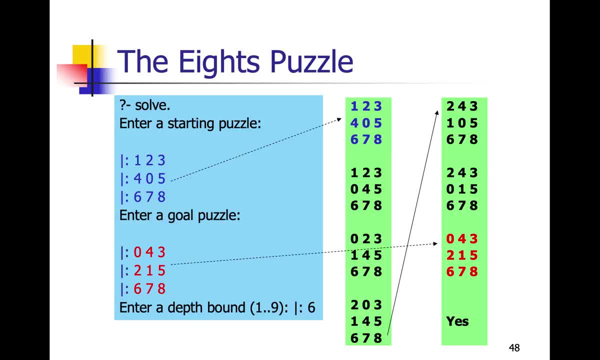 And so this is how you would solve it. You would enter in as a list, the three-by-three grid, So you'd have three lists of three items each. You'd have put in the start list. You'd have put in the start state. 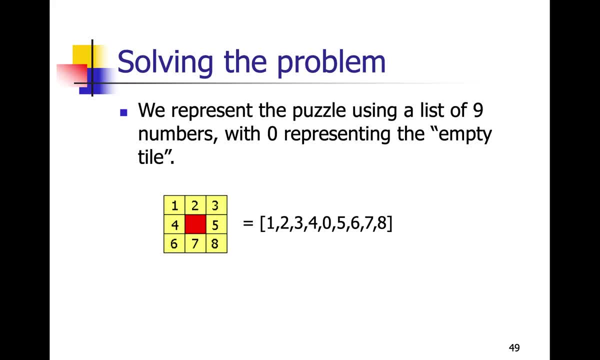 You'd put in the goal states And then Prolog would have the information given to it. So you'd represent the puzzle using a list of nine numbers with zero representing the empty space. So you can sort of see how these nine numbers would show. the grid would show in a list of nine numbers. 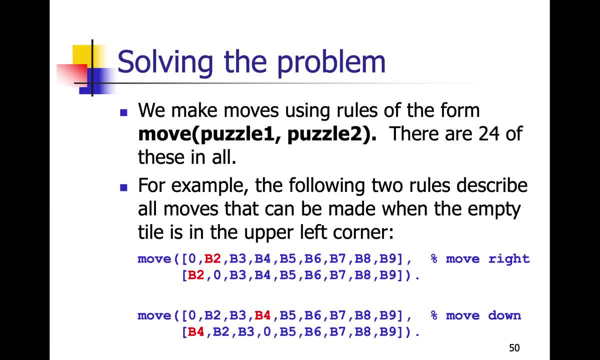 And then you'd have a move function that would move, So you'd make moves using the rule in the form of move function, From puzzle one to puzzle two, And there's 24 of these in all, And so the two rules describe all of the moves that can be made with the empty upper left-hand corner. 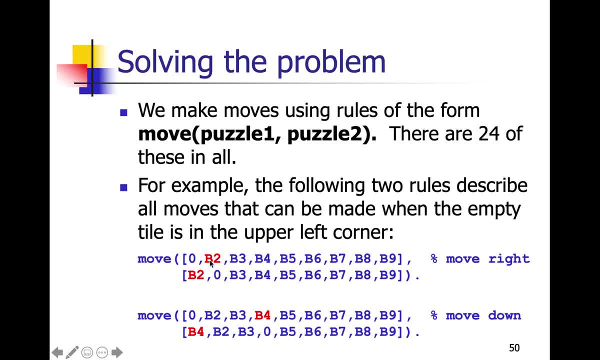 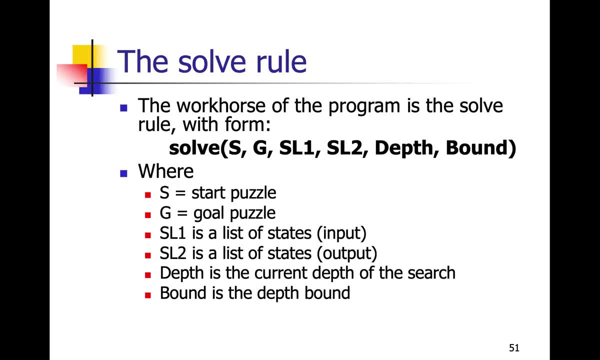 So upper left corner, So move. and then the B's, the ones in bold, are showing you what pieces are actually being moved, And you could go through the entire series of 24.. So the workhorse of the program is to solve the rule with solve. 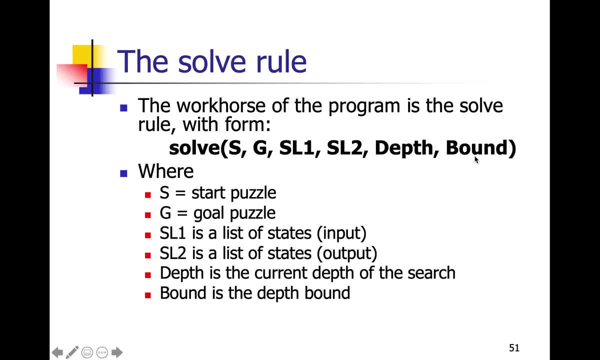 With the start, the goal State one, state two, depth and bound, Where you've got the list of the input, the list of the output, the depth of the current search tree and the length of the tree and the depth of the bound. 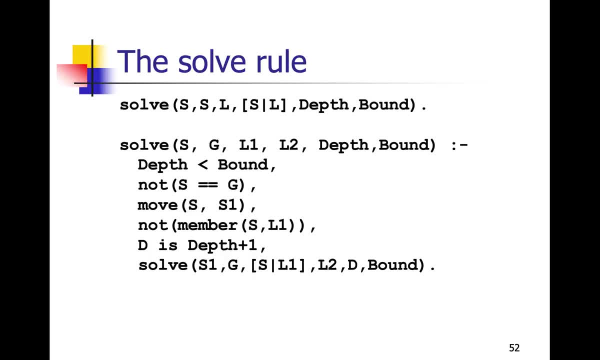 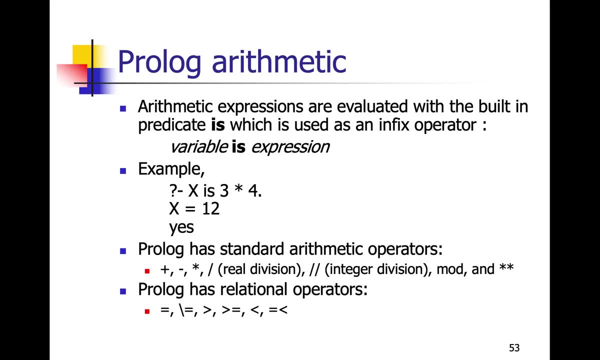 And so you'd solve it by going through each one of the states until you reached it from the start state to the goal state. So that's an example of how you would be able to use Prolog to solve a Rubik's Cube question. 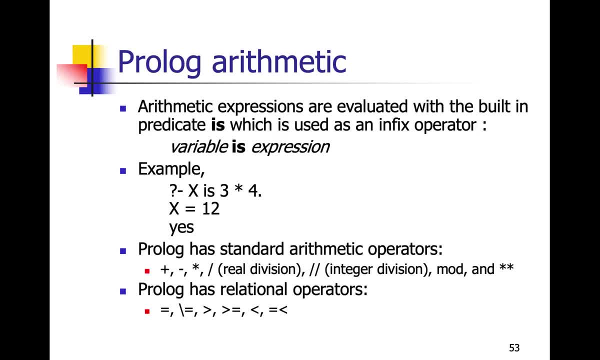 Prolog does math. This is absolutely not a math language And I don't recommend doing math with this language, But there's arithmetic expressions that can also be evaluated. There's a predicate: is, which is used as an infix operator, So the variable is expression. 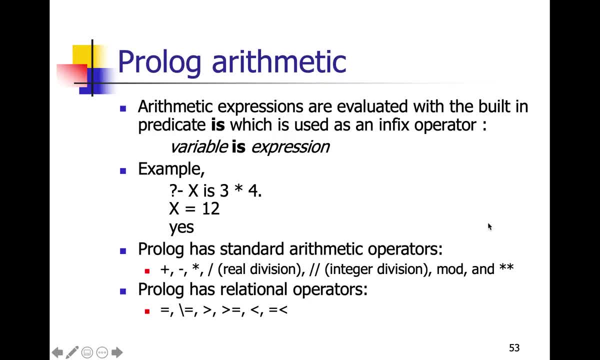 So X is, in this particular case, 3 times 4.. And then, as you might imagine, the arithmetic operators that you're familiar with are used as well. It also supports relational operators: The less than or equals to- Okay, The greater than. 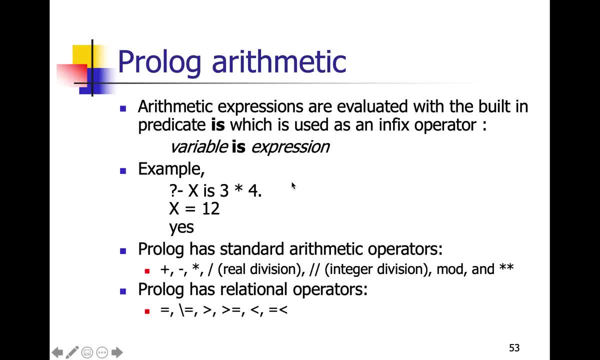 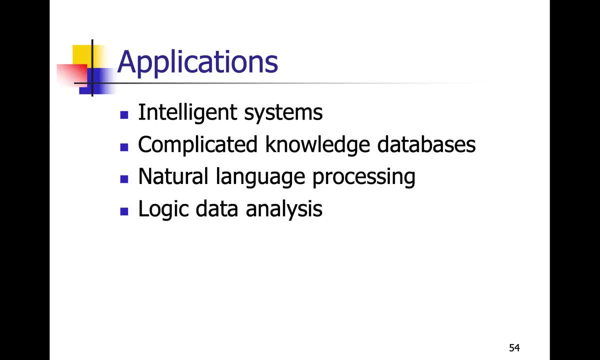 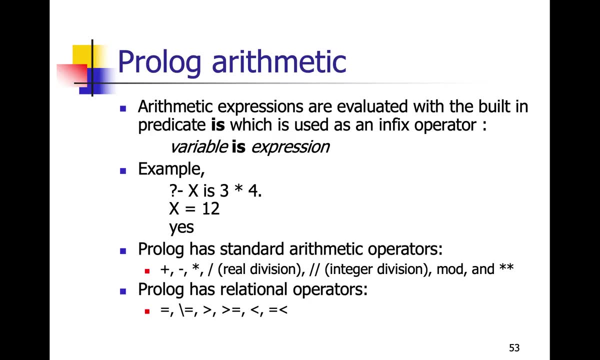 So you just go 3 times 4.. Yes, Prolog can do math and arithmetic expressions And people do use it for this, But I don't know if I'd recommend it. Just go back to the midterm and think about the order of operator precedents and how many levels of operator precedents are really defined. 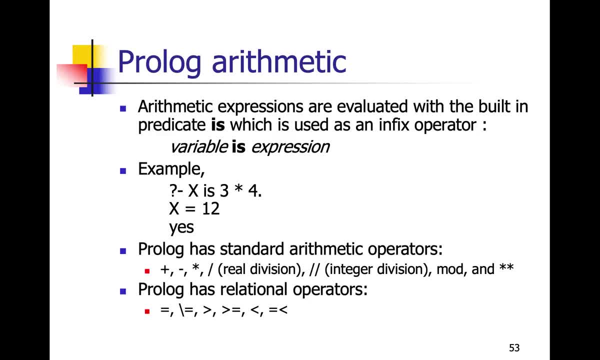 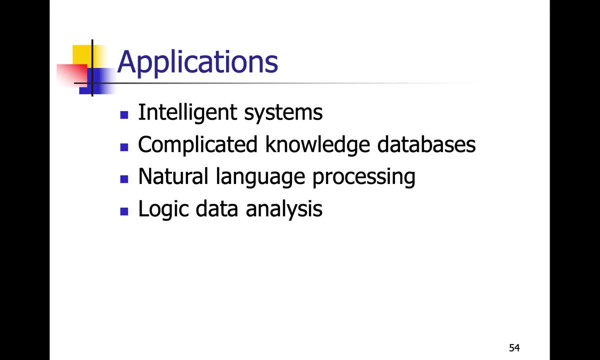 Nothing. Just one level And associativity rules is just one. So it's just one associativity rule, One associativity with that. So it is kind of limited. Other applications for Prolog would be intelligence systems, complicated knowledge bases, natural language processing, logic and data analysis. 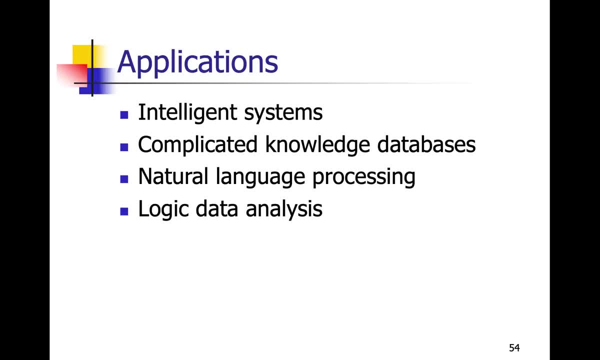 These are some areas where, if you go on to take an artificial intelligence course, you might get exposed to Prolog again. Prolog does a lot of language processing. It does a lot of problem solving, where you have lists of data and you're trying to find correlations between the data or you're trying to answer questions on it. 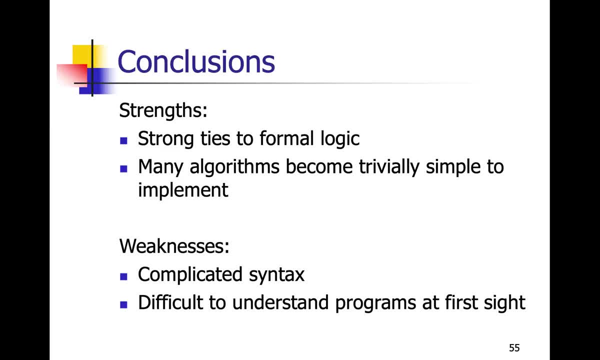 So, in conclusion, we have some strengths. We have a strong tie to formal logic, many algorithms that become very simple if implemented, And Prolog does all of this for you. You just give it the pieces, give it the facts, give it the rules. 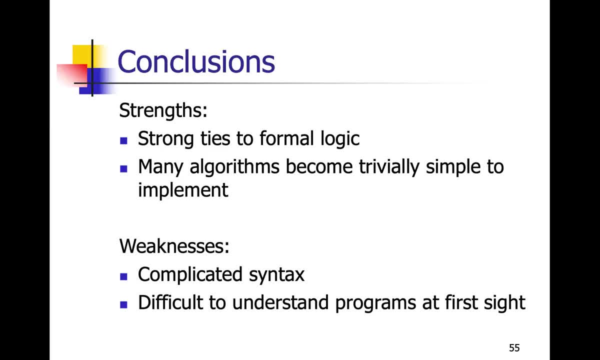 It already knows how to make decisions. Weakness. Well, it's kind of complicated syntax. It's kind of limited. All you need to do is write facts and rules or create a list and have the list processed through a functor, And it is kind of complicated. looking for a programmer. 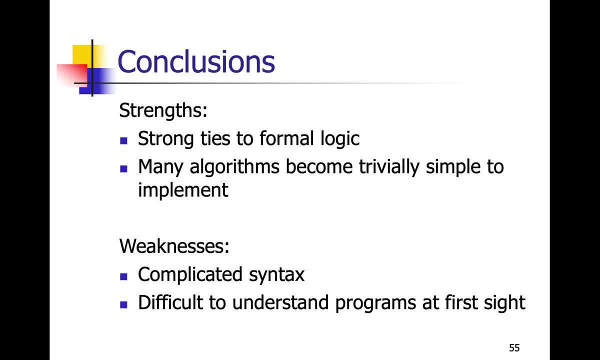 Now, if you're not a programmer, you'd probably think this was easiest programming on earth. And you go: oh, I want to be a programmer because this is really simple, There's not very much to write. But unfortunately, when you look at it, it's difficult to understand the program. 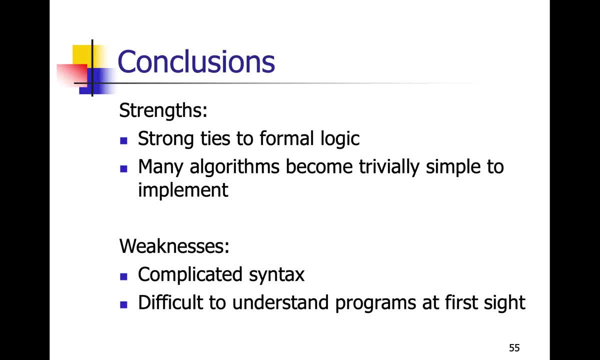 What is the program doing? I have no idea. In fact, just go on to the Swishy website and you'll look at some of the sample programs that are out there, And the first thing you're going to say is: how do I run this? 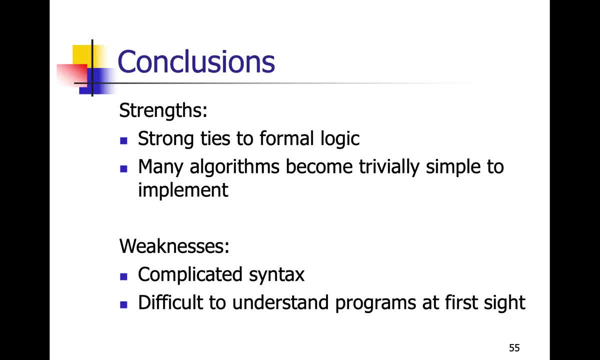 How do I make this work And if you really want to get familiar with Prolog, go out there and play around with some of those sample databases, Or knowledge bases as they're supposed to be called, And see if you can ask it questions and see if you can use it. 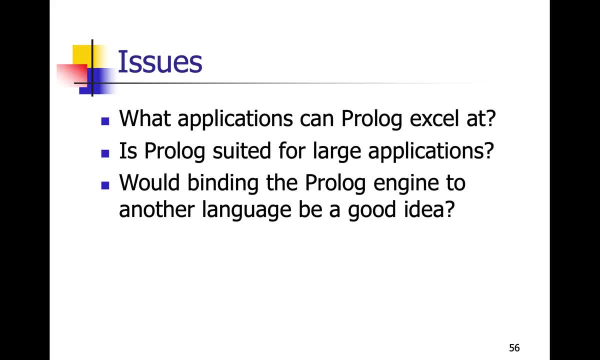 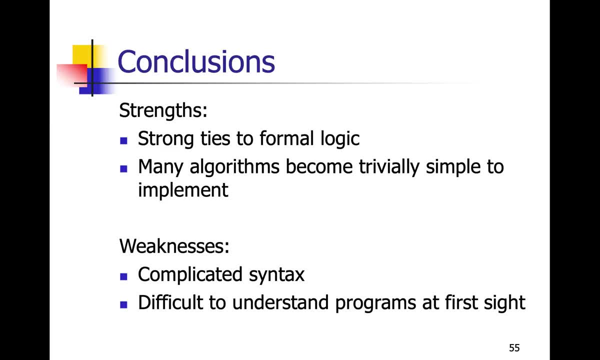 And follow through the documentation And it will, You'll definitely be able to hopefully pick up. to see. You guys are computer science students. You should be able to figure out how to run a Prolog program And it's pretty simple actually. 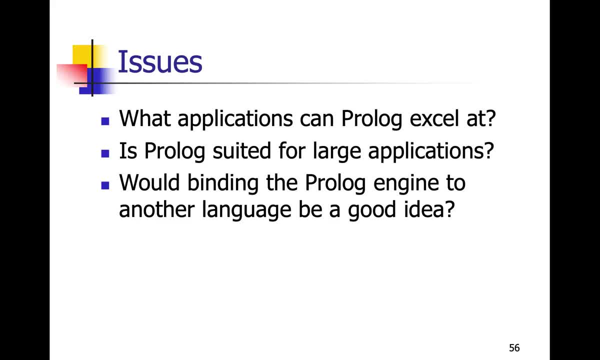 But it's difficult to understand the program at first sight. Issues are: what applications can Prolog excel at Knowledge bases? It's pretty limited. I couldn't write. I can't really even write hello world with it. really, I guess you could write hello world. 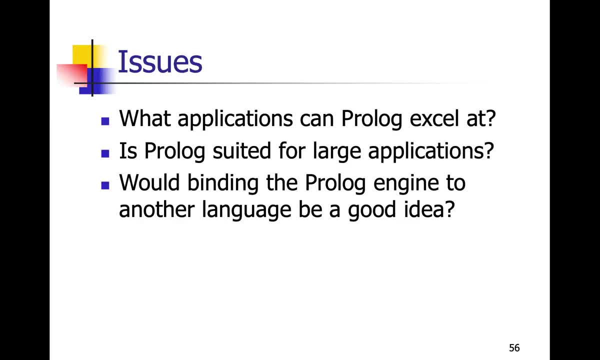 Just make a fact that the world says hello world. And then you say, well, Hello world. And it comes back and says, yes, Is Prolog suited for large applications? Probably not. How about binding Prolog with another language? Is that a good idea? 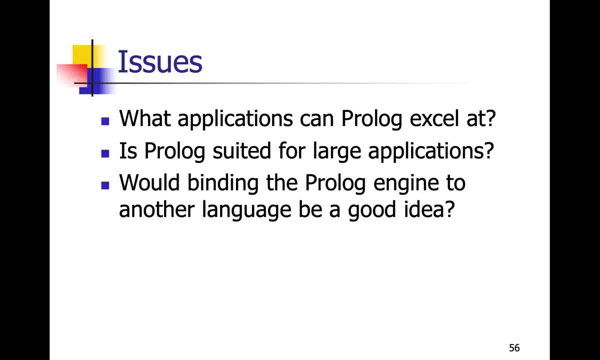 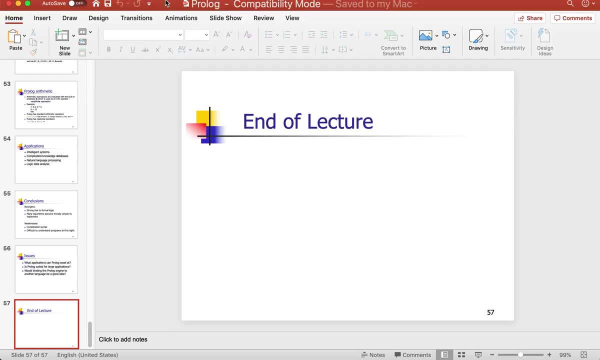 Yes, but it's not been done yet. It hasn't really been done yet. So I'd say, Maybe it is a good idea, but we haven't seen it yet, So Okay, so That's pretty much all I could give you on the Prolog language. 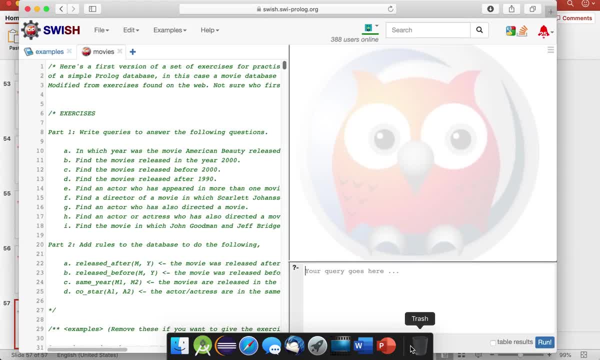 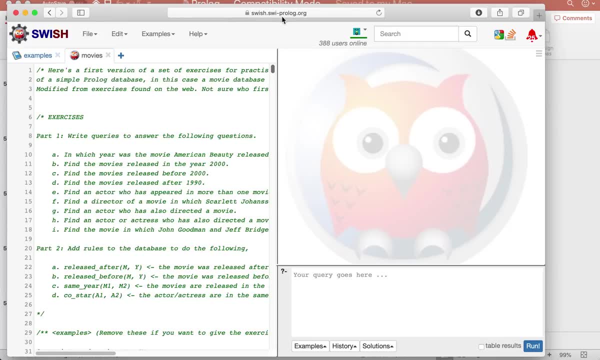 It's. It's very straightforward. Your next step- what I would try to do- is go to the Swish website. Here it is up. here You can pause the video and go to this website up here You can download. You can cut and paste from the window and save your code. 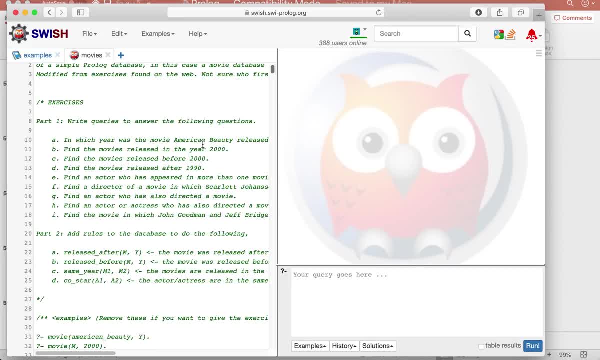 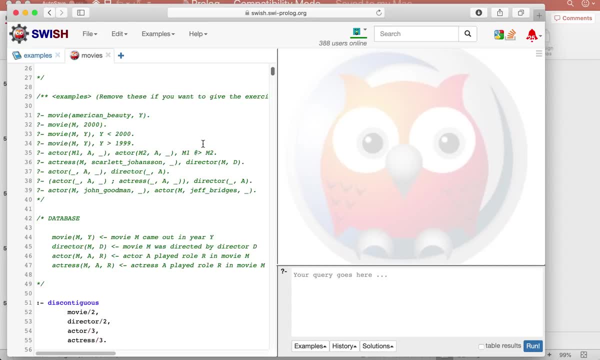 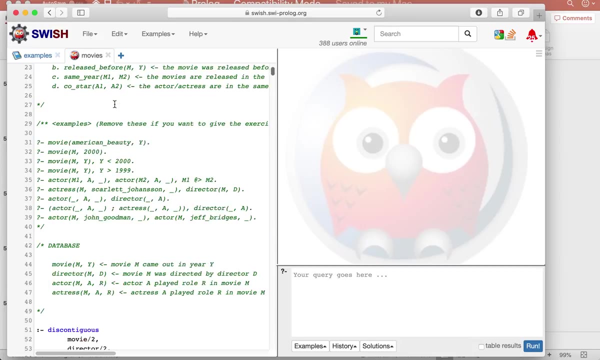 You can download it, Save it When you submit it to me. you can actually just open up the Microsoft Word file and paste in the answers to the questions and the functions that you're writing. These are examples. What do I have open? 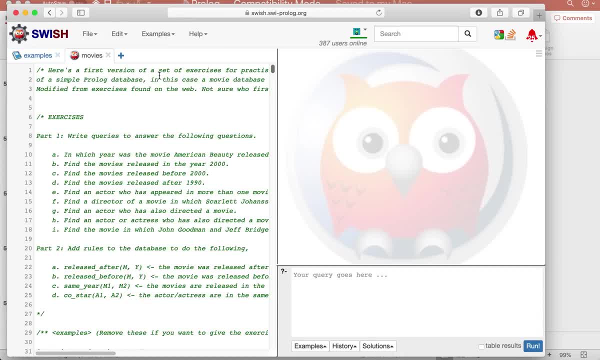 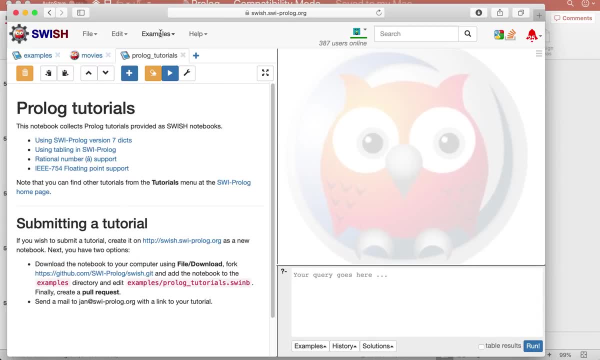 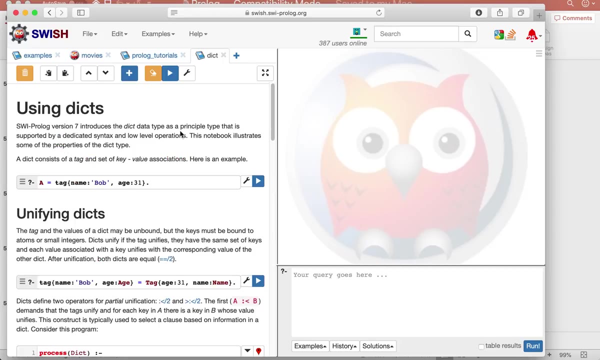 I have the movie one open. There's a Prolog tutorial you can run through. Learn about how to write Prolog programs. The tutorials are pretty cool using Swishy version 7.. It shows you how to use it, So play around with this website.